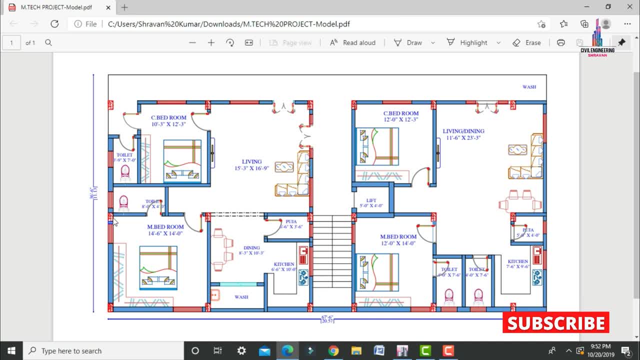 in vertical direction. the first column to second column distance- let us take it as 3 meter. Again I am taking second column to third column distance- is 4 meter, which is equals to 7 meter. This is applicable for G plus 4 building plan, So I will take same particulars for the respected G plus. 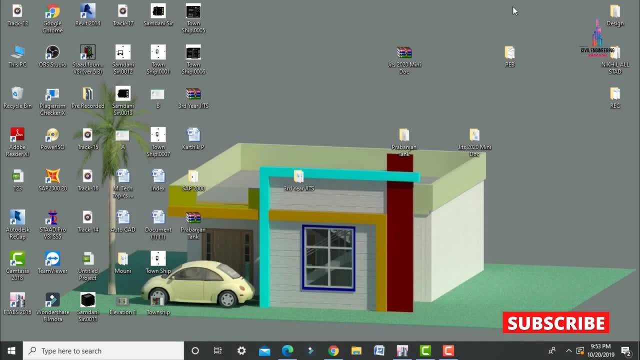 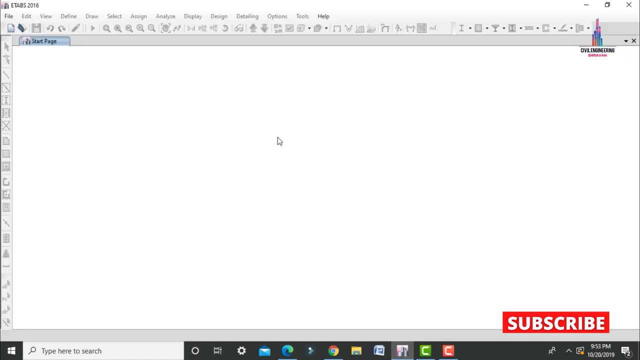 4 building structure. So for that, initially we need to click on the ETAP software. So select your ETAP software here, double click on it. The software will be open like this. So initially we need to click on file option here. Click on new. 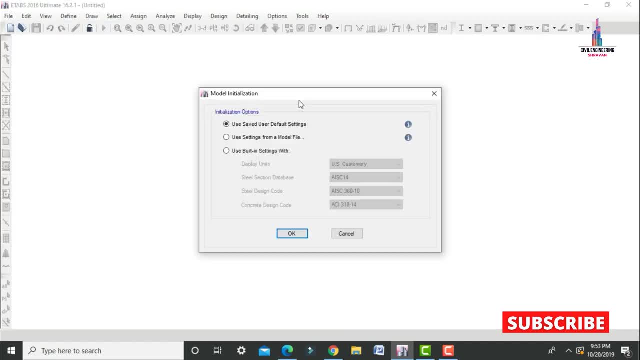 model here. So click on new model. So initially we need to select the initialization options here. So it will be consisting of user saved, user default settings, user settings from model file and user built-in settings. So from this respected three options we need to select. 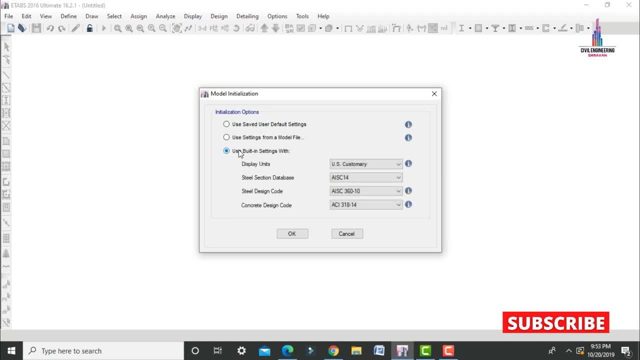 the last one, which is consisting of your user built-in settings with. So it will be consisting of display units option, steel section database and steel section design code, concrete design code. So, as per the considerations, we are doing this project in Indian standard system, So we need to take the values as well as your. 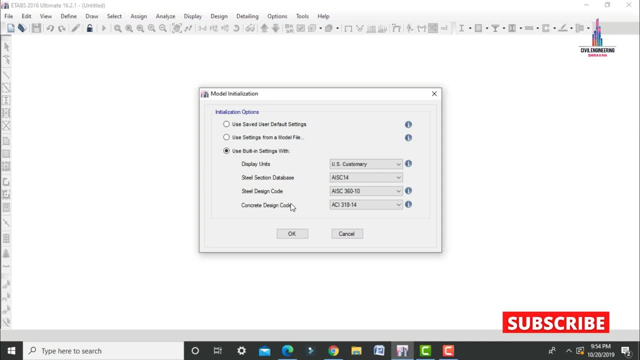 respected code or provisions as per the Indian standard system only. So here I am taking display units in metric SI system. Again I am taking the steel section design database as per the IS code. So here I am selecting the unit code as Indian standard system. Indian. 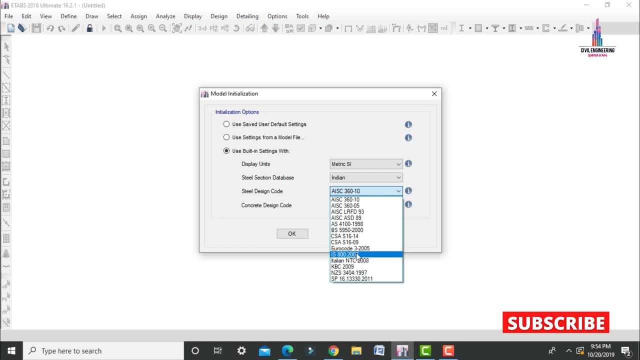 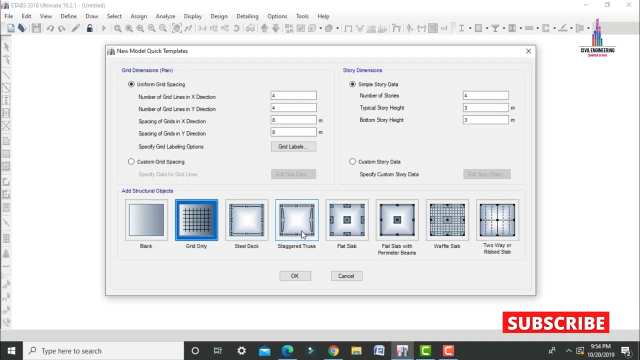 Again I am selecting. the steel design code is also Indian, which is consisting of IS 800-2007.. Now we have to select the concrete design code here Again. here also we need to select the code as Indian standard system 456.. So after that, click on ok option. Now it will open your respected 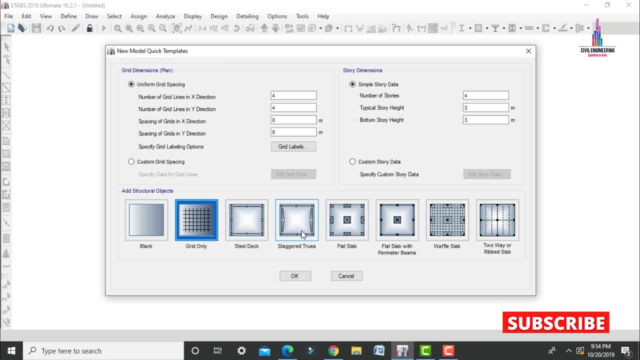 new model quick templates option like this, So it will be consisting of your grid dimensions data and story dimensions data. Grid dimensions data is nothing but the center to center distance between the column for each of the three options, So it will be consisting of your grid dimensions. 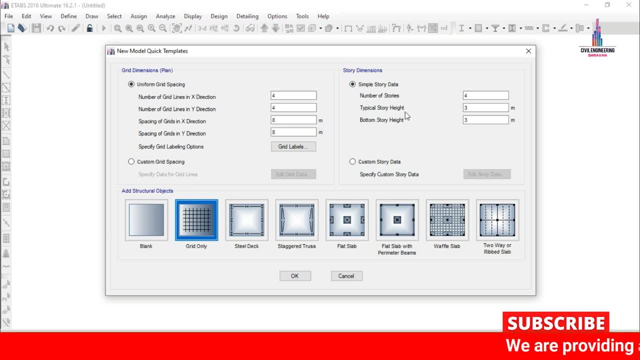 data and story dimensions data for each floor. Story dimensions data is nothing but the data which is related to the number of floors and floor to floor height. So it will be consisting of number of grids in x direction, number of grids in y direction, spacing in x direction. 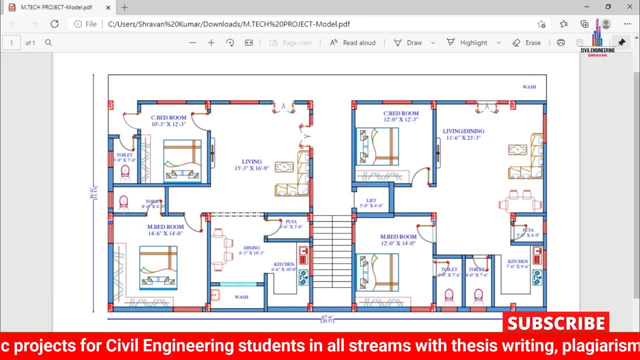 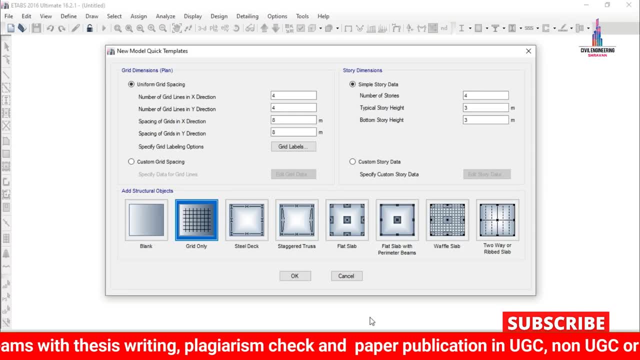 spacing in y direction. So, as per the plan, it will be consisting of: number of lines in x direction are 1,, 2,, 3,, 4,, 5, 6 here. So here we have to take the x lines are 6.. Again, we have. 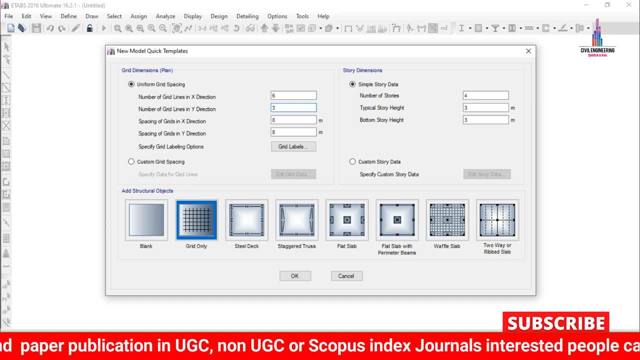 to take the number of lines in y direction which are equal to 3 here. Why? Because we are taking the two sections, So again we have to enter the spacing in x direction- Let us take it as 3, and spacing in y direction, Let us take it as 3, for example. 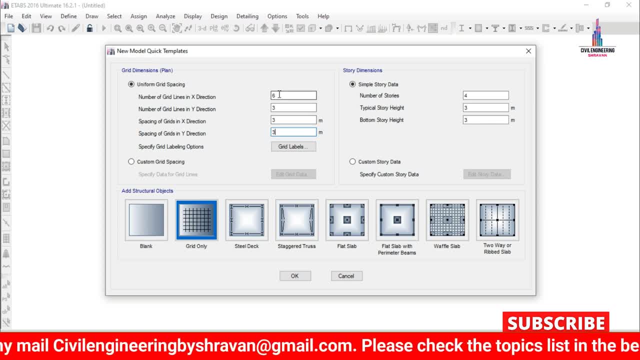 So after that it will open your respected 3,, 3 options for the 6 number of grids here. So we have to add the data which is related to the center to center distance between the column with varying dimensions. So here I was taking 3 value, 3 value which is regular value which is multiplied. 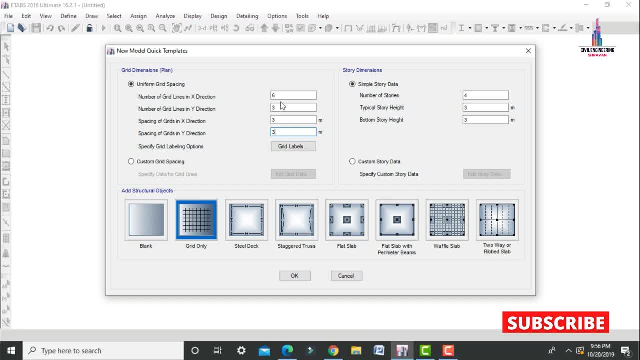 by your respected 6.. This will give you the number of grids in x direction. So after that we have to enter 2 foreign lines and we will get 18 meter, which is ve hiç upgrading length, which will be abstract. positive value of grids for the new basic grid rather than 3 models with. 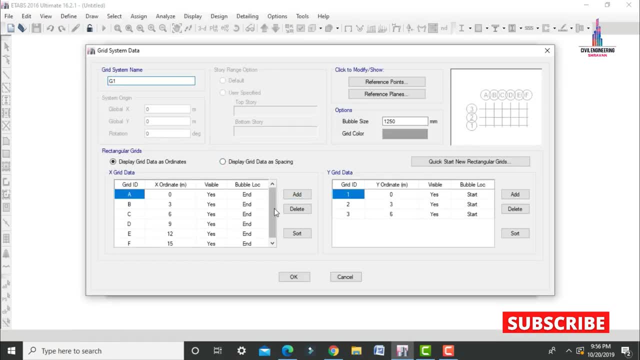 grade value of 18 meter. My building length is not equal to 18 meters by 18 meters, but it is equal to 17 meters. To edit the respected data, we have to select the Custom grid space option here. Click on Edit Grid Data Map scope. Change the dimension as per your specification related: 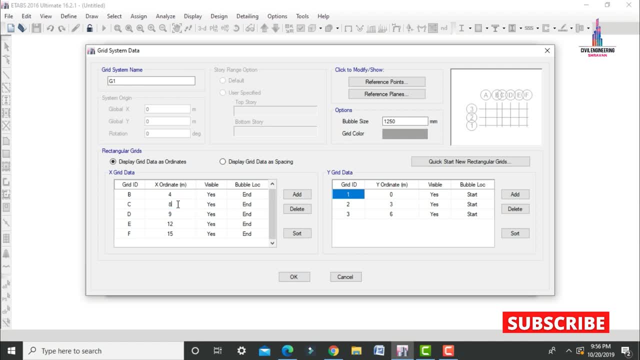 to coordinate x or coordinate z. So initially we have to enter the data for the respected options. the second grid, which is equal to 4 plus 4, which is equal to 8. here again i am taking third grid, length, which is consisting of 8 plus 2, which is equal to 10. now i am taking the next grid, which 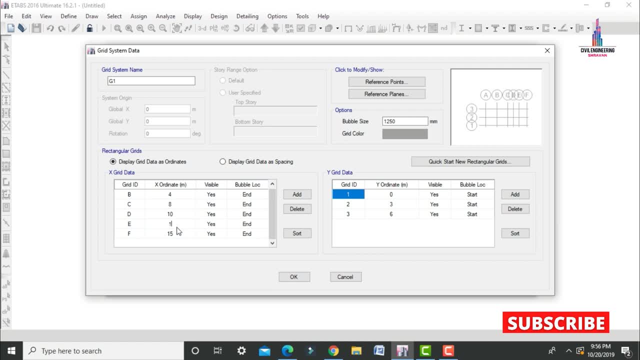 is equal to 10 plus 3, which is having the intensity of 13. again, i am taking the last grid, which is consisting of 13 plus 4, which is equal to 17 meter. so after that we have to enter the data which is related to the y direction grids. so initially i am selecting the 2 value as 3. 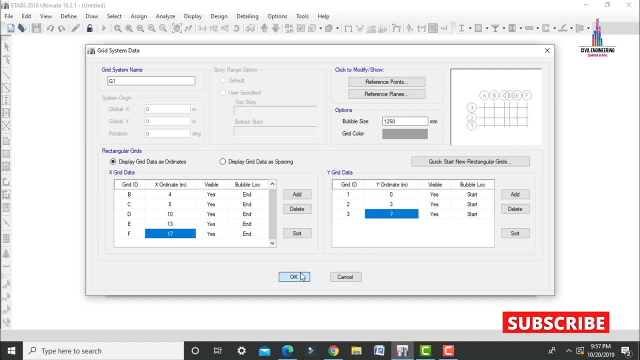 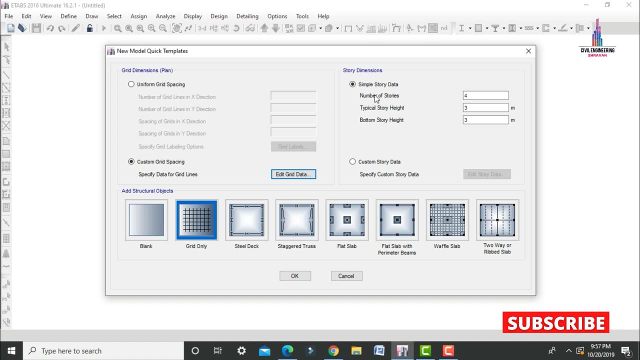 again, i am taking the 3 value as 7, so click on ok, so it will change the grid dimensions data here. so after that we have to enter the story dimensions data. so here, as per the problem we have to consider, the number of stories are 5. why? because? why? because we are considered the g plus 4. 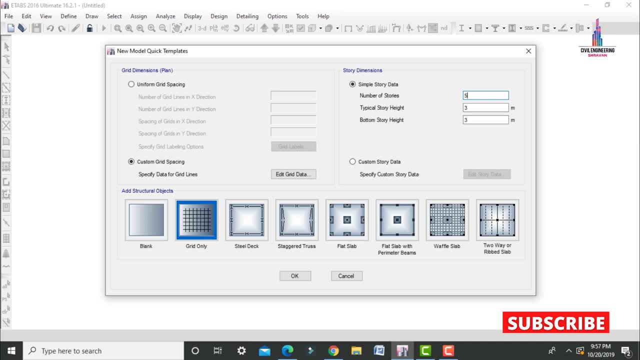 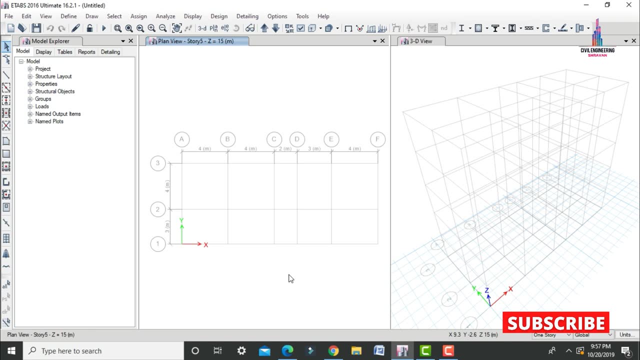 structure, so 4 plus 1, which is equal to 5. now we have to select the grid only option here. okay, click on ok option so it will open your respected grid options here like this: okay, so this is the left hand side section window. this is the right hand side section window. left hand side section window will be consisting of: 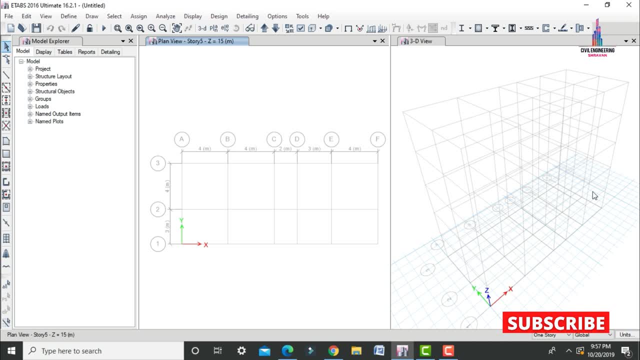 the plan view of the building and right hand side section will be consisting of the 3d of the building. okay, so after adding these grid lines, which is related to your g plus 4 building, we need to define the material properties. material properties is nothing but the grade of the. 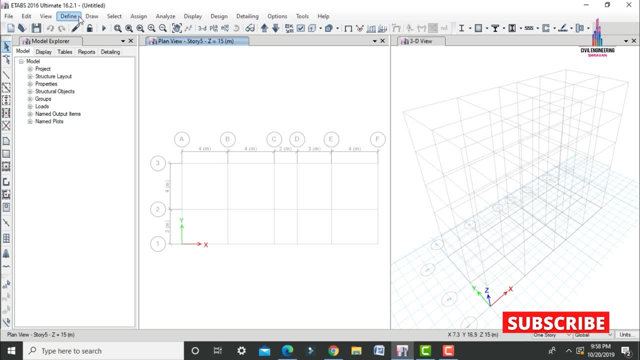 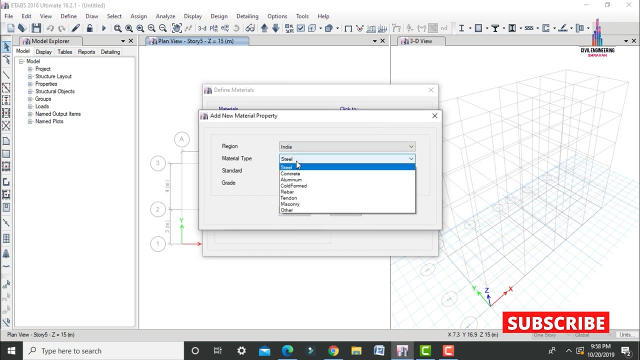 concrete and grade of the steel. okay, so for that initially. click on define option. here select the material properties. so initially we need to delete all previous properties here. so here i'm selecting this property. click on add new material. here initially we need to select the indian standard system code and material will be of concrete section. so here i'm selecting. 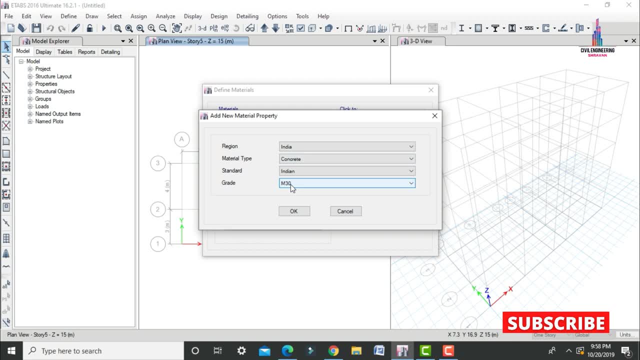 indian standard system which is having concrete grade of m30 grade. click on ok. so after that we have to click on ok option here. now we have to add the steel section also, so click on add new material. so it will be consisting of your respected indian standard system code and material type will be of: 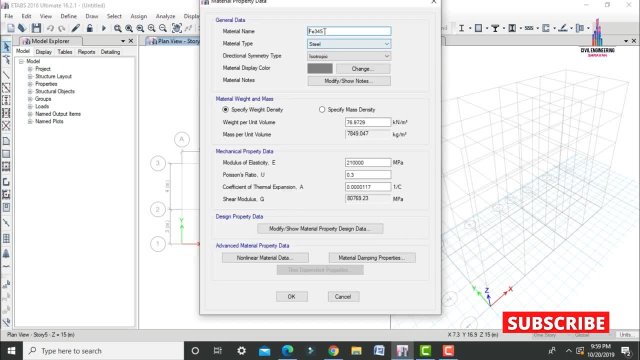 indian standard system. click on. ok, so, but the material property which is related to the steel. it was added with fe 3, 4, 5, but here, as per the definition, we need the value of 500 grade, let us consider. so here we have to enter the data which is related to the 500 grade. so for that, 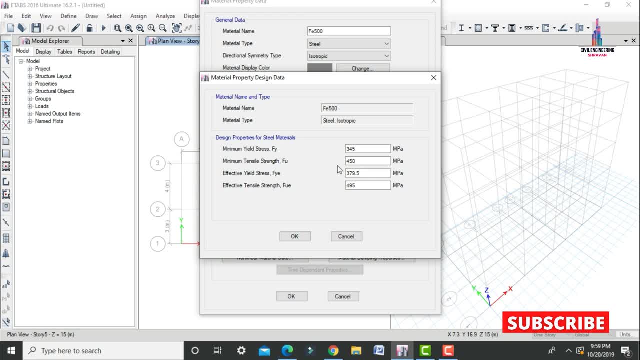 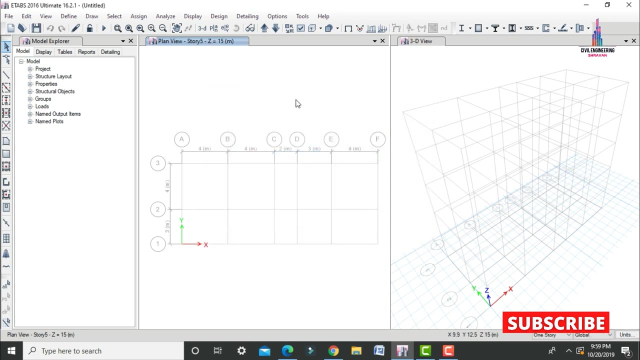 we have to select the modify show material property data here now. here we have to change the data from 4 or 3, 45 to 500. again, every value will be same. click on ok. click on ok here. so click on ok now. after defining the material properties, we need to define the beam size and column size. 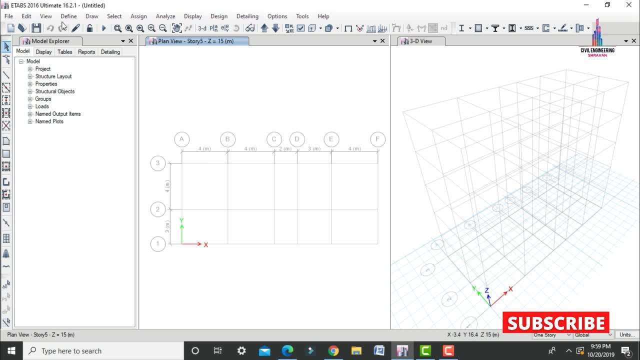 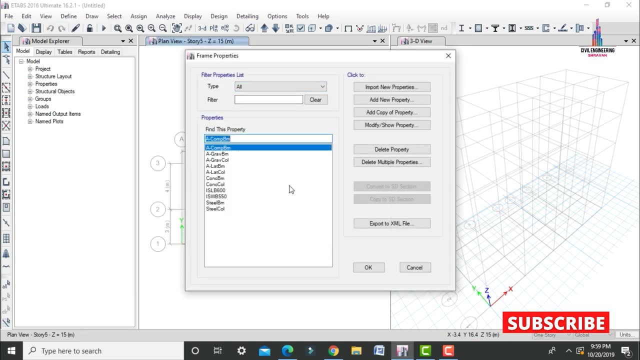 for this building. so for that, initially we need to click on define option here. so click on section database, select the frame section so it will be consisting of the number of sections like this: initially we need to delete all previous sections. so here i'm selecting delete multiple options. 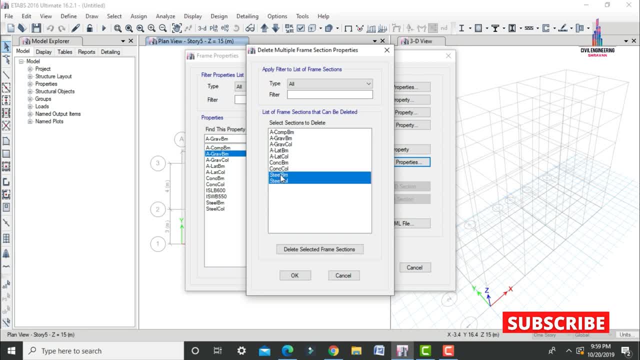 so select all previous sections here for this respected structure building. so here i'm selecting all my previous section. click on delete frame sections so it will be deleted with all previous sections, but at least it. it is needed to add two properties, so that's why it was added with two. 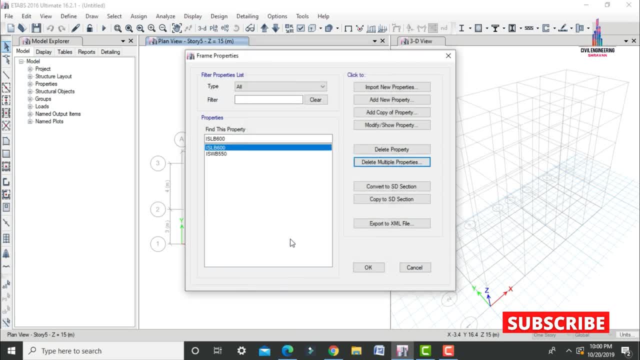 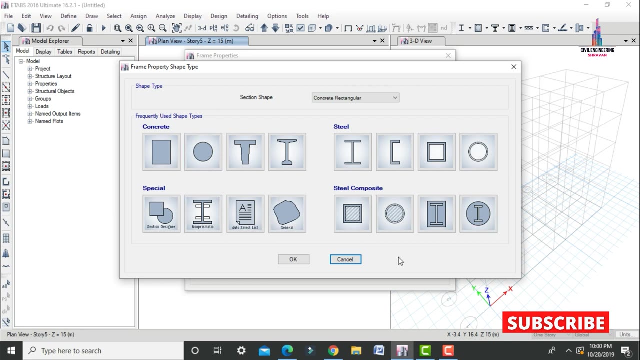 sections here. after adding the requirements of our beam size, column size, we will delete this respected property. so initially we need to add the beam size, so click on add new property here. so we need to select the concrete section or steel section or special section. add composite section, depending upon your 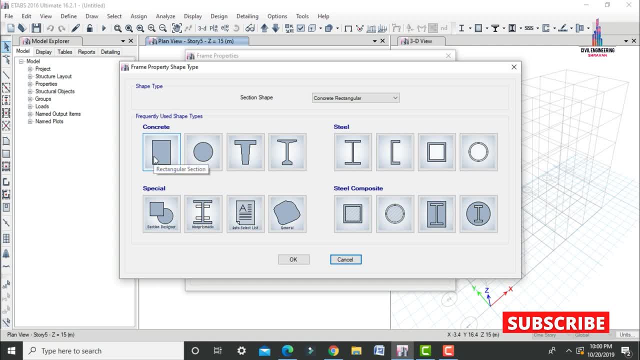 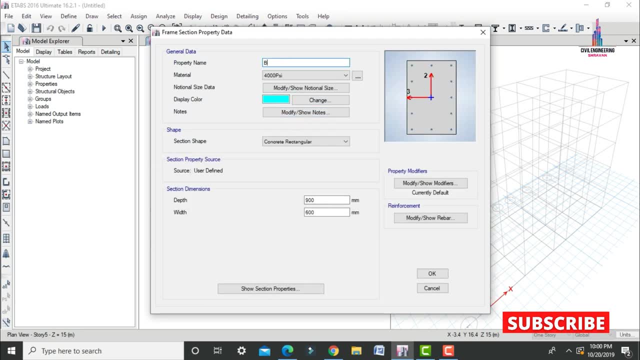 requirements. so here, as per my definition, i am considering the rcc building only. so that's why i just am selecting rectangular section here. so here we have to give the property name. initially just i'm taking 0.35 cross. 0.35 is the beam size. again we have to select the material property as per the 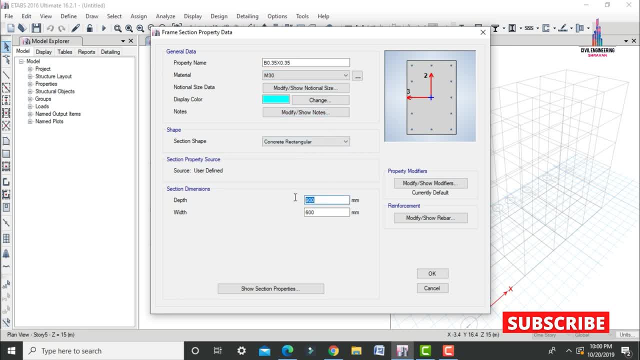 grade of the concrete. now we have to select the depth as well as width of the beam. okay, so here, considering depth of the beam is 0.35, again, uh, width of the beam is 0.35, which is equal to 350 cross 350 intensity values here. okay, which is related to the section dimensions: 350 cross 350. 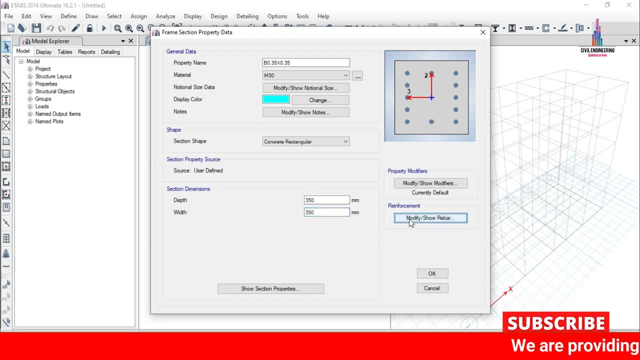 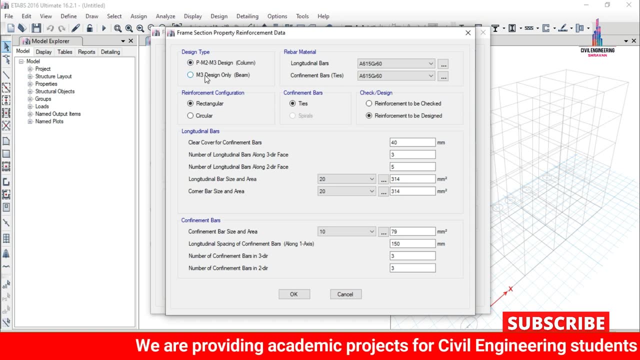 here. okay, so after that we have to click on reinforcement option here now. here we have to select the uh rebar material, which is related to the beam section. only select the beam here. so again we have to select the longitudinal bars and lateral bars, which is related to the 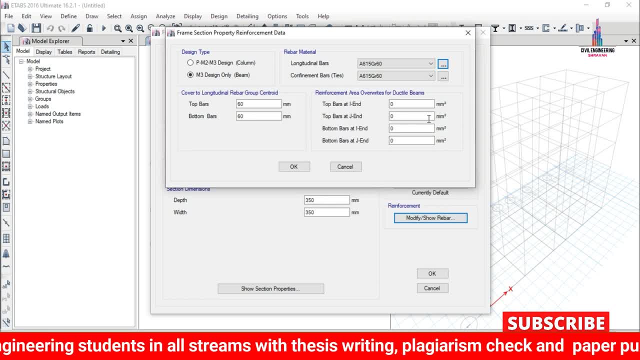 fe 500 gray steel. click on ok so it will add your respective properties here like this: now again i am selecting. the next one is fe 500 gray steel. here: now, here i am selecting. the top as well as bottom cover will be equal to 50 mm. 50 mm. click on ok option. so click on ok again in the 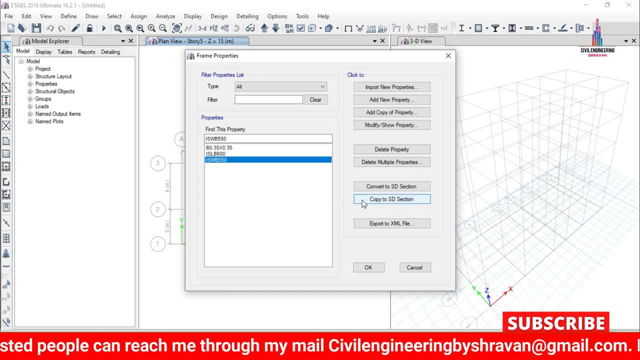 same way. we have to delete the two properties here. so click on delete multiple options. select this property again. i'm selecting this property. click on delete option. click on ok. so it was added with only pro 1 property, which is related to the beam which is having the dimensions of 0.35 cross. 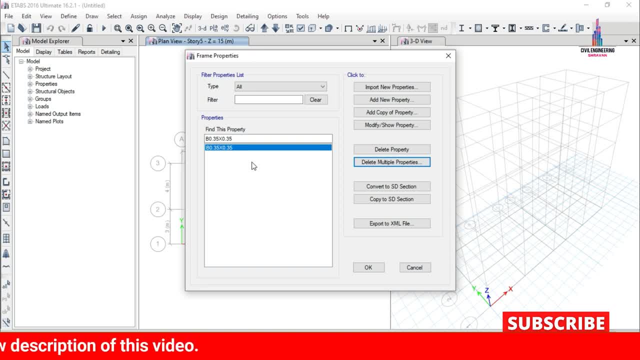 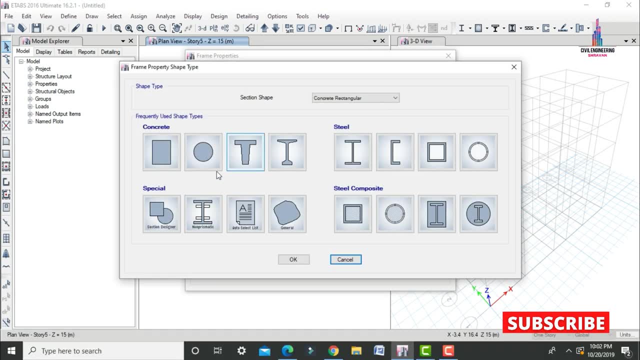 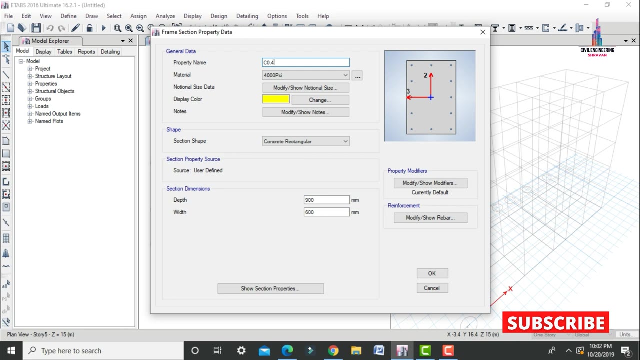 0.35. so after adding the beam dimensions we need to add the column dimensions. so initially we need to define the column dimensions. also add a new property here: select the concrete material. so now we need to give the name of the column. select zero point. four, five, cross zero point. 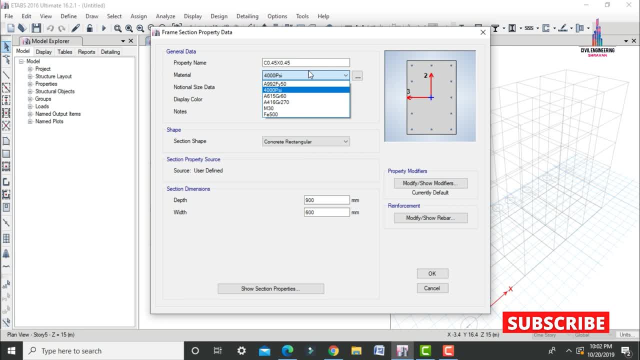 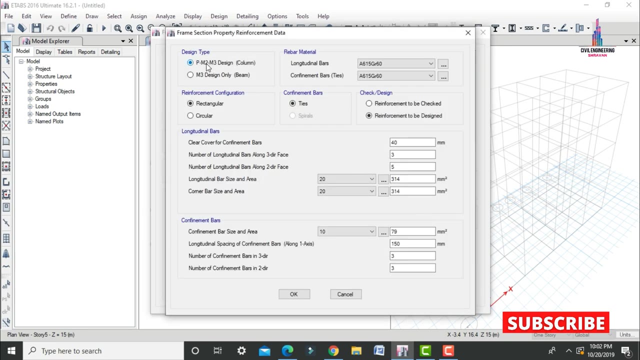 four, five is the column dimensions. now i am selecting the fe- sorry, m30- grade, concrete. now here i am giving the depth as 450. again, width as 450. now, in the same way, we have to select the reinforcement here. click on the reinforcement, select the column here and change the longitudinal. 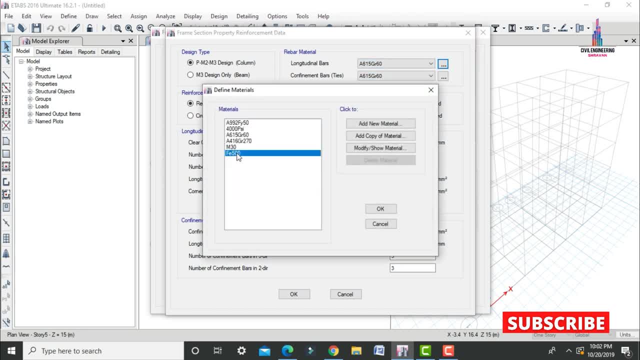 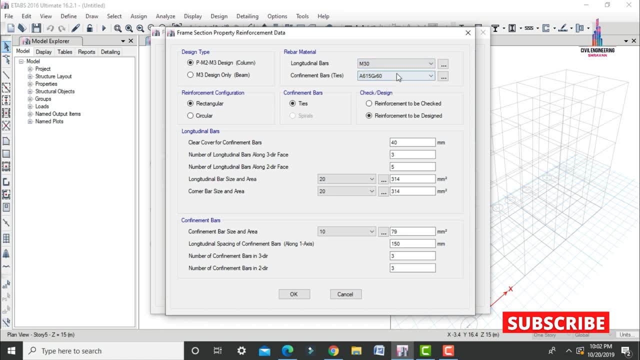 bars and confinemental bars as per the indian standard code which is related to the fe 500 gray steel. again i am selecting this material. sorry, again i'm selecting this material. click on add button. again i'm selecting this material. click on add button. so after that we had to enter the longitudinal bars. so here it was suggested that. 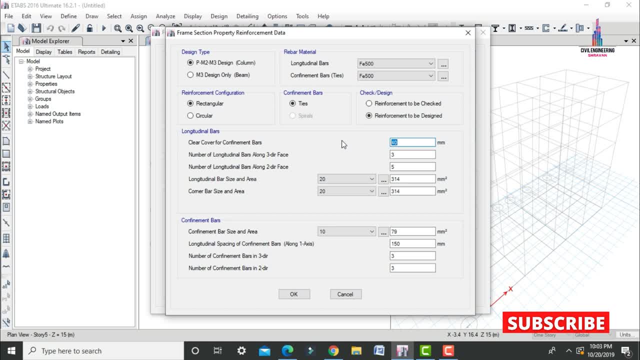 the cover as 40 mm, which is taken as 10 percentage of the dimensions of the column, so you can modify it as 50 here. and number of bars: along three direction you can change it to four. and longitudinal two direction was also four, so here we had to select the longitudinal bar size, corner bar size. 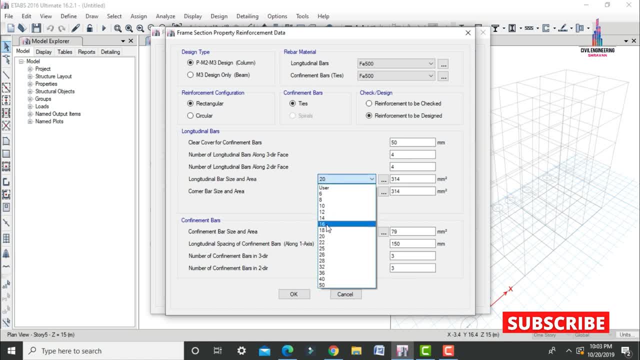 so, as per your requirement, you can go ahead and change the bar size as per your requirement. consider the bar sections. okay, so here i'm taking 20 mm bars for longitudinal bars and corner bars for confinement bars. here i'm selecting it as 10 mm bars. click on ok option again: click on ok. 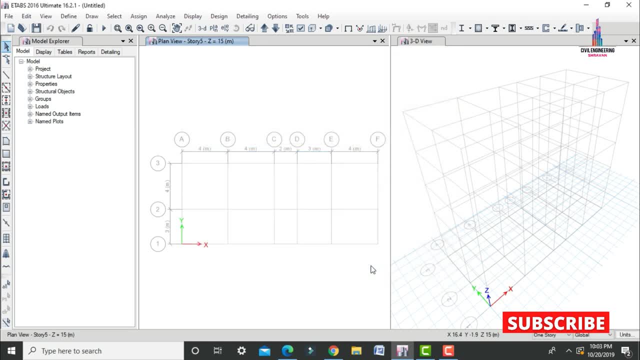 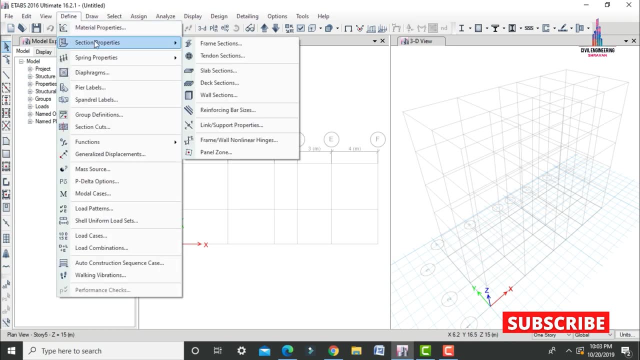 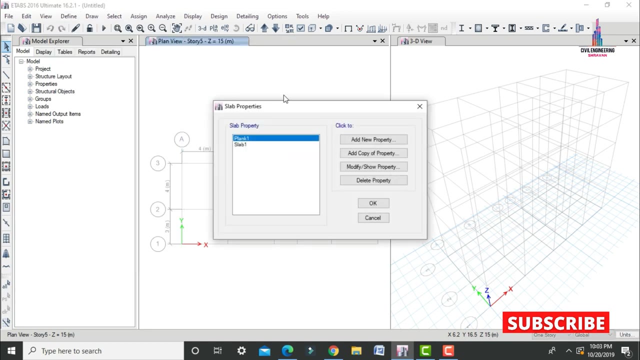 option. so after that we have to click on ok. option: now we have to define the slab thickness for this building. so click on define. so select the section properties. in this we need to select the slab thickness, slab sections- okay. third option: so select this. so initially we need to delete the. 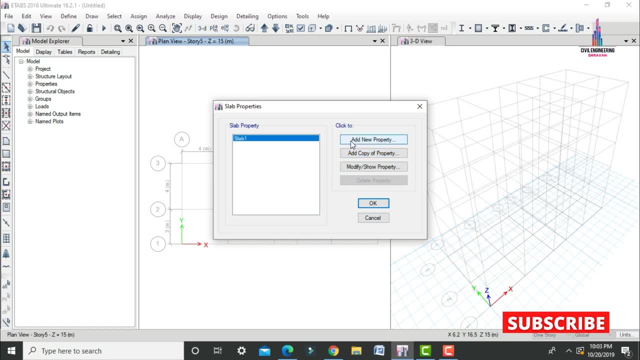 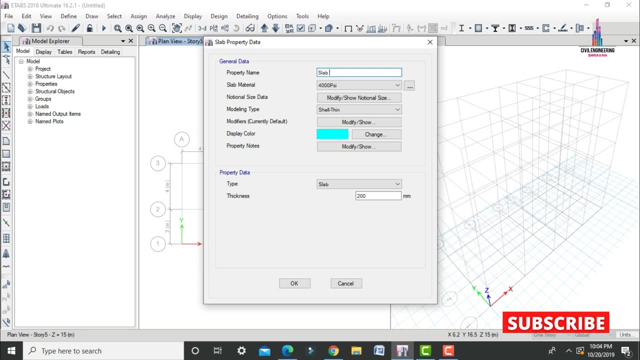 property which is related to the default one. so click on add new property here now. here we need to give the property name, okay, so slab- let us consider it as 150, and slab material will be related to m30 grade and we have to select this as membrane section. it will be consisting of: 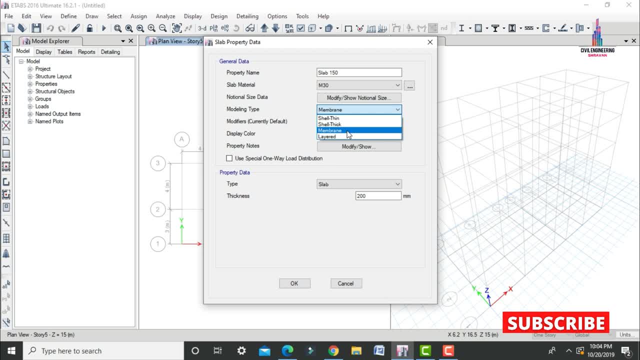 shell thin, shell thick, membrane, and this respected section. so in that we need to consider the membrane only, so after that we have to select the type as slab and we have to give the thickness as 150 mm, okay option. so after that we have to select the slab. 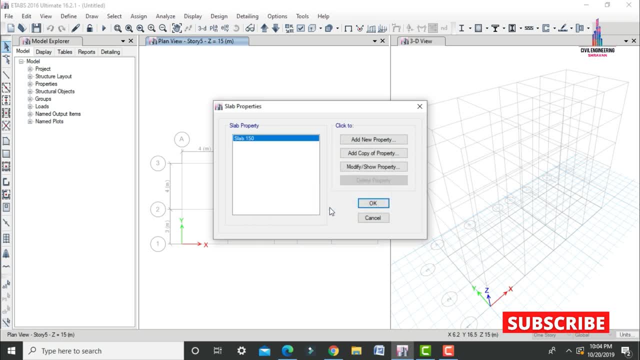 one section here. click on delete property. click on s option, click on ok. so after defining the properties which is related to the beam sections, column sections and slab sections, we have to assign those properties for this building. so for that, initially we need to change the one story. 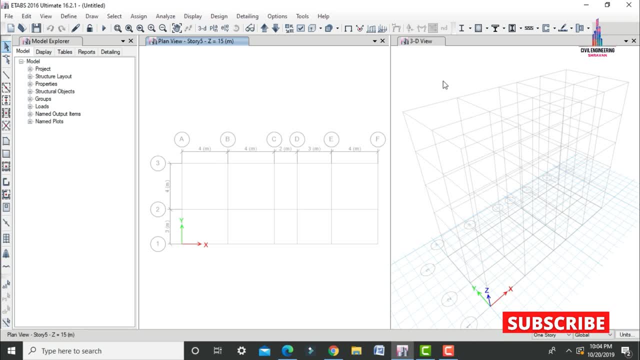 option. so for that we need to change the one story option. so for that initially we need to change the one story option. so for that initially we need to change the one story option to the all stories option, to the all stories option here. okay, so here it will be consisting of the option here as one story. 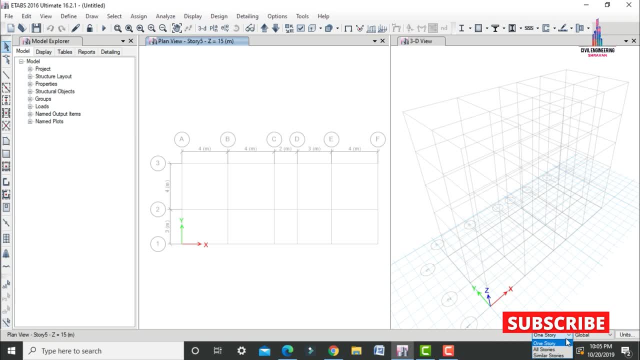 here: okay, so here it will be consisting of the option here as one story instead of one story option we need. instead of one story option. we need to convert that to all stories options. select all stories option. to convert that to all stories options. select all stories option here. okay, so now we need to assign. 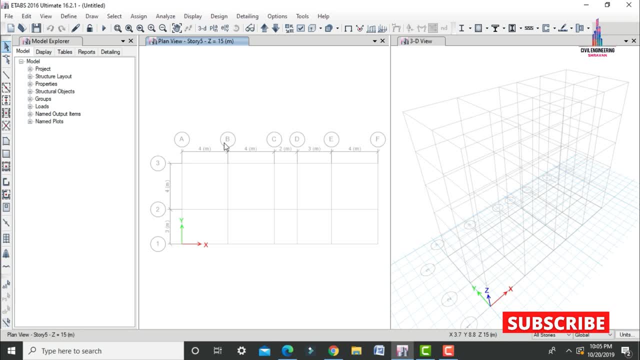 here. okay, so now we need to assign the beam sections. for assigning the beam sections generally, we will the beam sections. for assigning the beam sections generally, we will have two methods. okay, now, i will have two methods. okay, now i will explain you the first method. so after that i will explain you the. 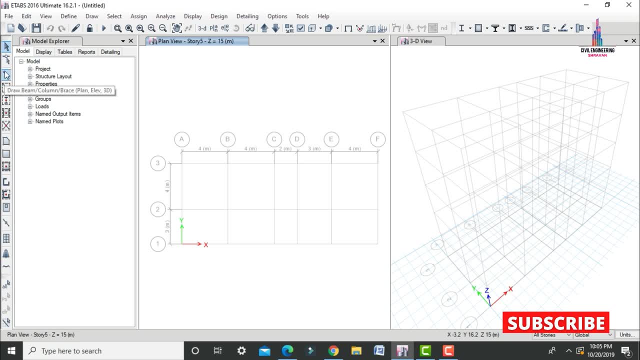 explain you the first method, so after that i will explain you the second method. first method is we need second method. first method is we need to draw the lines, okay, and draw the beams okay. so select this, to select this, to select this respected option, draw beam option. so it 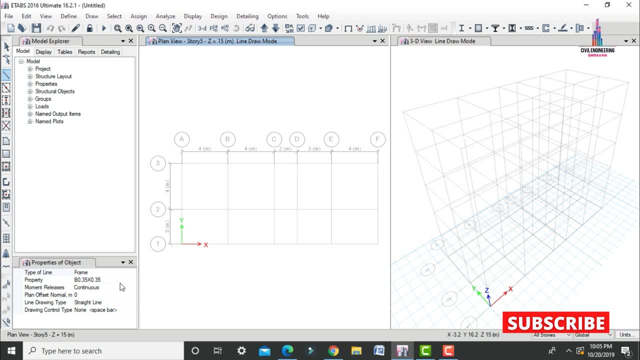 respected option. draw beam option so it respected option. draw beam option so it will open your respected properties. will open your respected properties, will open your respected properties. option here like this. so initially we need option here like this. so initially we need option here like this. so initially we need to check that property, whether it is. 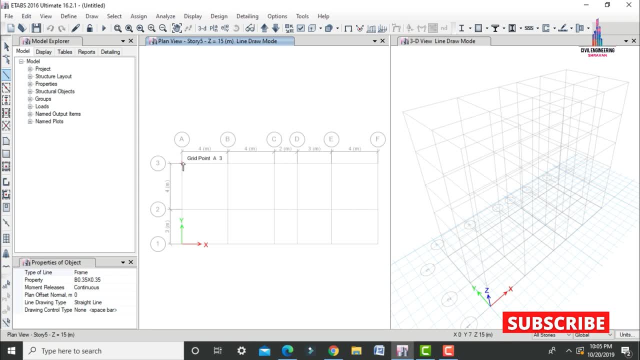 to check that property. whether it is to check that property, whether it is comes under your beam section or column comes under your beam section or column comes under your beam section or column section. now we have to select the first section. now we have to select the first. 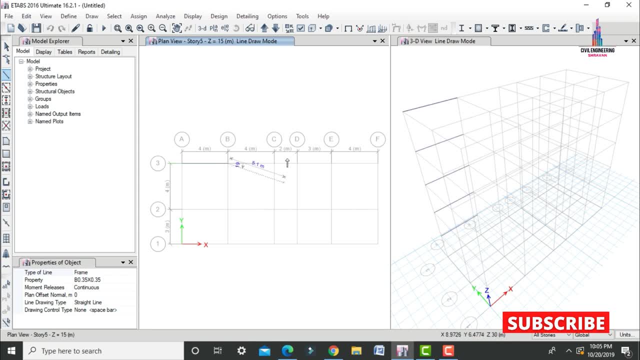 section. now we have to select the first grid and we have to select the second grid and we have to select the second grid and we have to select the second grid. okay, so it will assign your beam grid. okay, so it will assign your beam grid. okay, so it will assign your beam property here like this: now we can see: 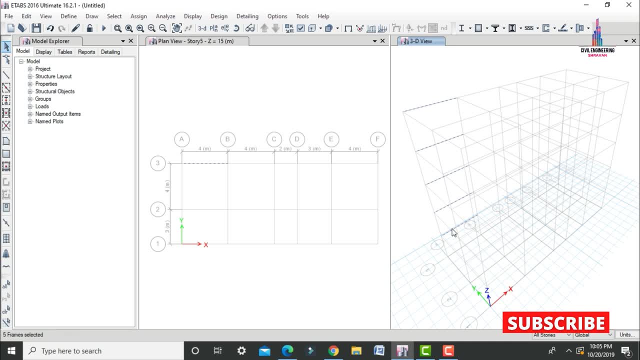 property here like this: now we can see. property here like this: now we can see: the blue lines are indicates your beam. the blue lines are indicates your beam. the blue lines are indicates your beam. sections in each floor: okay, you can. sections in each floor: okay, you can. 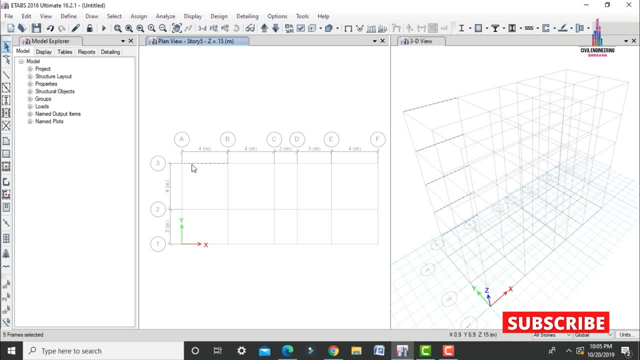 sections in each floor. okay, you can select that blue lines and you can select that blue lines and you can select that blue lines and you can delete it, delete it, delete it, uh, as per your requirements. okay, so here, uh, as per your requirements. okay. so here, uh, as per your requirements. okay, so here the first option will be: indicates your. 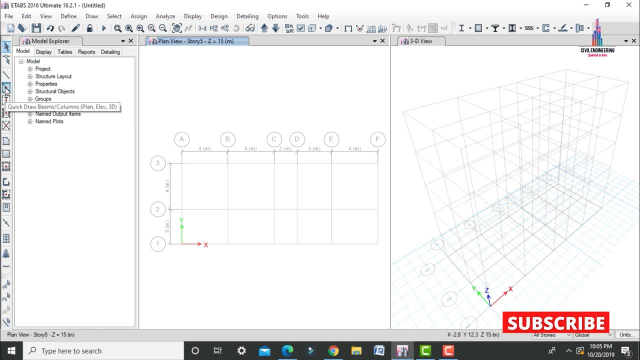 the first option will be indicates your. the first option will be indicates your draw option: draw option- draw option- okay. second option will be indicates your okay. second option will be indicates your okay. second option will be indicates your uh. quick draw beams option- okay, so you okay. second option will be indicates your uh. quick draw beams option- okay, so you can select the center point of. 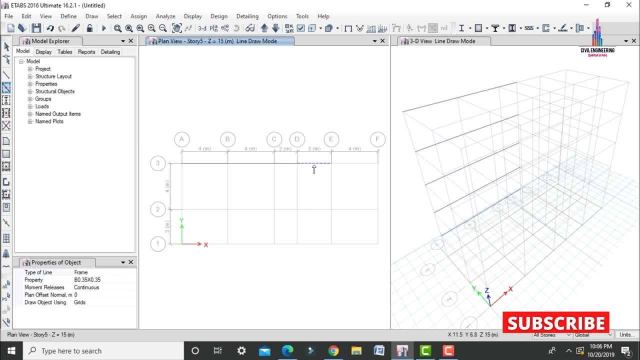 can select the center point of. can select the center point of that respected structure. you can select that respected structure. you can select that respected structure. you can select the beam sections here like this: so it the beam sections here like this: so it the beam sections here like this: so it will assign your beam sections like this: 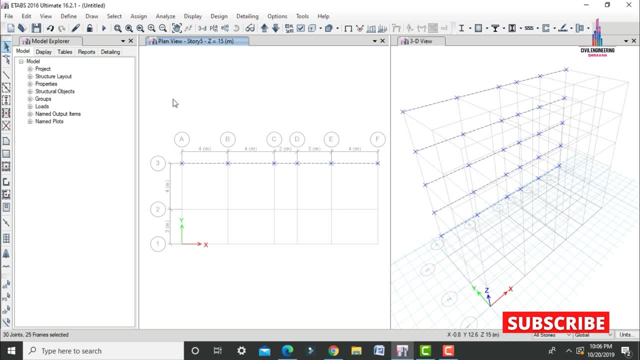 will assign your beam sections like this. will assign your beam sections like this: okay, so, in this same way, you can assign: okay, so, in this same way. you can assign: okay, so, in this same way, you can assign to the respected properties for this, to the respected properties for this. 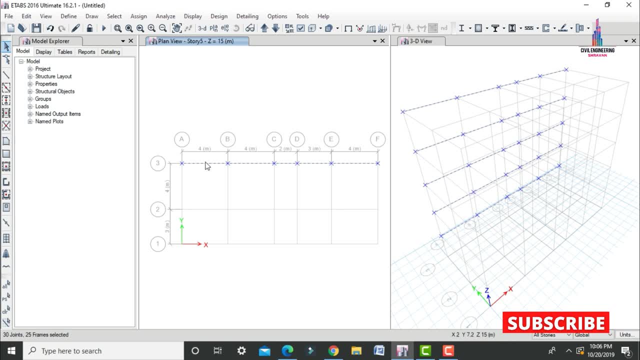 to the respected properties for this building. okay. so if you are facing any building, okay. so if you are facing any building, okay. so if you are facing any kind of the difficulty for assigning, if kind of the difficulty for assigning, if kind of the difficulty for assigning if this respected properties, for that we 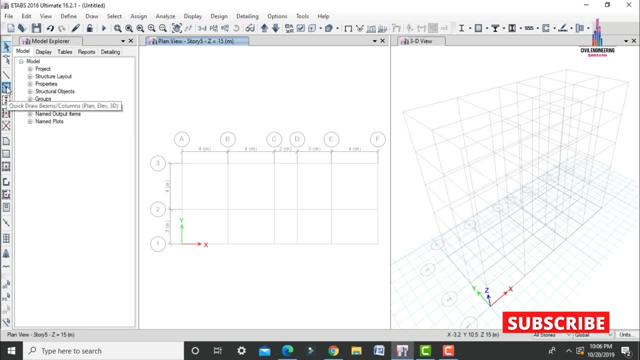 this respected properties, for that. we this respected properties for that we have. another method is also there, so have another method is also there, so have another method is also there, so select the second option simply. you can select the second option simply. you can select the second option simply. you can select the option properties here as per. 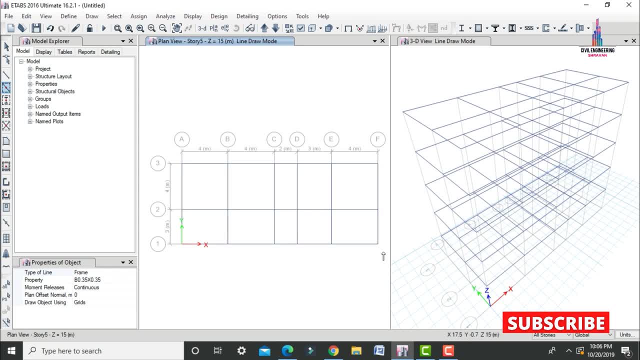 select the option properties here as per. select the option properties here as per the beam sections. you can drag to the the beam sections. you can drag to the the beam sections. you can drag to the respected properties here. okay, so it respected properties here. okay, so it respected properties here. okay, so it will assign your respective beam. 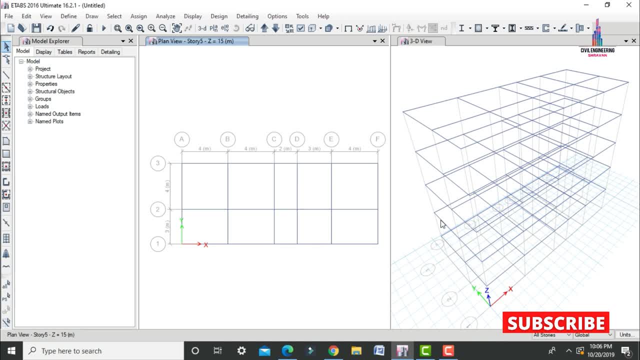 will assign your respective beam, will assign your respective beam sections for this building of g plus 4. sections for this building of g plus 4, sections for this building of g plus 4. so after that, we have to assign the. so after that, we have to assign the. 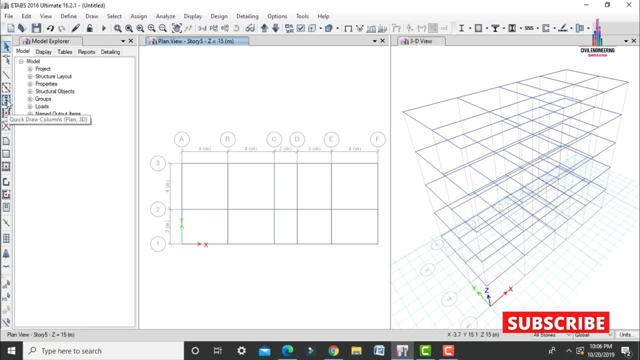 so after that we have to assign the column sections. so for that we have column sections. so for that we have column sections. so for that we have second option is there which is related? second option is there which is related. second option is there which is related to the quick draw columns you can select. 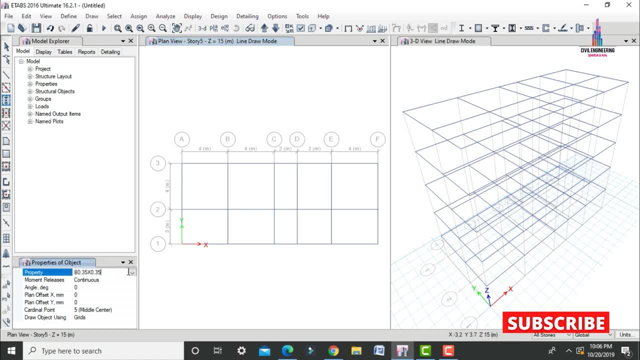 to the quick draw columns. you can select to the quick draw columns. you can select this option and you can change the this option. and you can change the this option and you can change the property from beam sections to the column. property from beam sections to the column. 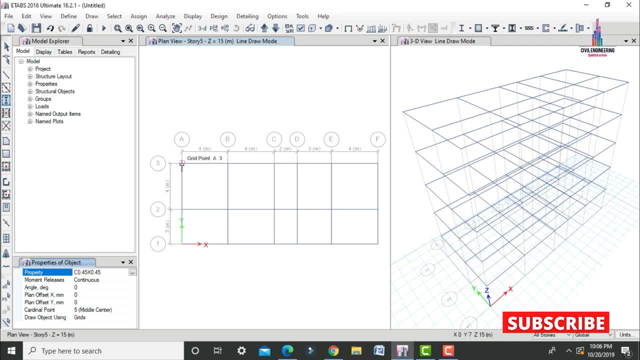 property from beam sections to the column sections, which is of 0.45 cross 0.45. sections, which is of 0.45 cross 0.45. sections, which is of 0.45 cross 0.45. you can select the center point at: 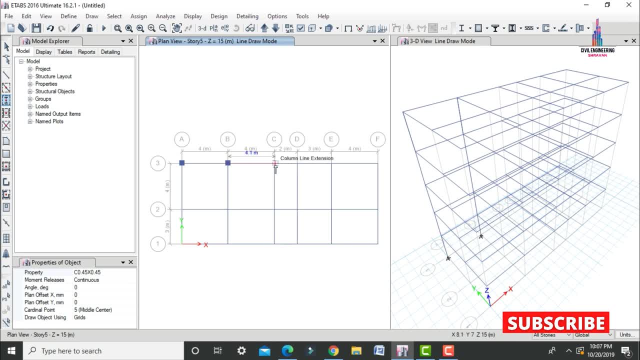 you can select the center point at. you can select the center point at different positions. okay, so you can different positions. okay, so you can different positions. okay, so you can select this center point for this. select this center point for this. select this center point for this. respected structure. otherwise we have. 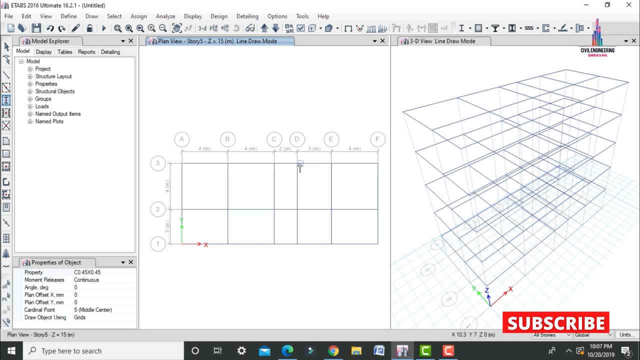 respected structure. otherwise we have respected structure. otherwise we have one more option is there for assigning? one more option is there for assigning? one more option is there for assigning of the column section for this section of the column section for this section of the column section, for this section. column section for the building. so you, 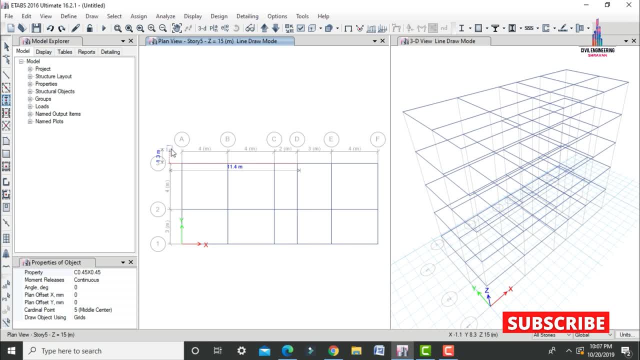 column section for the building. so you column section for the building, so you can select the i section. here you can can select the i section. here you can can select the i section. here you can drag to the respected model here, like: drag to the respected model here, like: 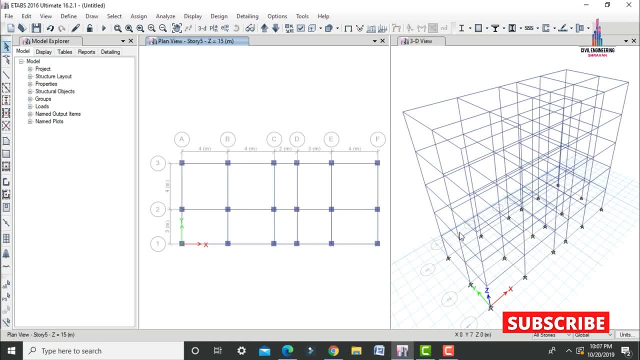 drag to the respected model here, like this: so it will directly takes your this, so it will directly takes your this, so it will directly takes your respected node points and it will respected node points and it will respected node points and it will directly assign your columns here, like: 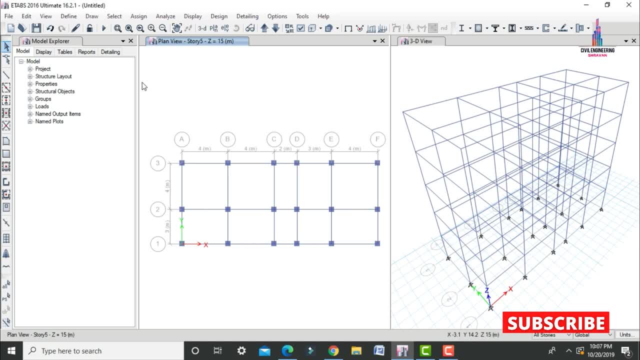 directly assign your columns here, like: directly assign your columns here, like this: so after that we have to assign a this. so after that we have to assign a this. so after that we have to assign a slab section. so for assigning the slab, slab section, so for assigning the slab. 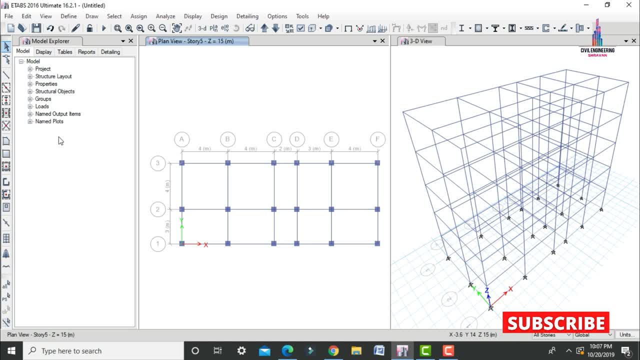 slab section. so, for assigning the slab section, we have three options. are there section? we have three options. are there section? we have three options. are there individually? i will explain you the individually. i will explain you the individually, i will explain you the usage of that respective three options. 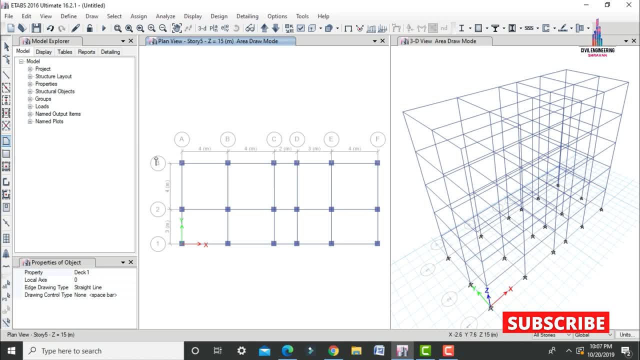 usage of that respective three options. usage of that respective three options. so in that first option is draw floors. so in that first option is draw floors. so in that first option is draw floors, okay, select this option and you have to. okay, select this option and you have to. 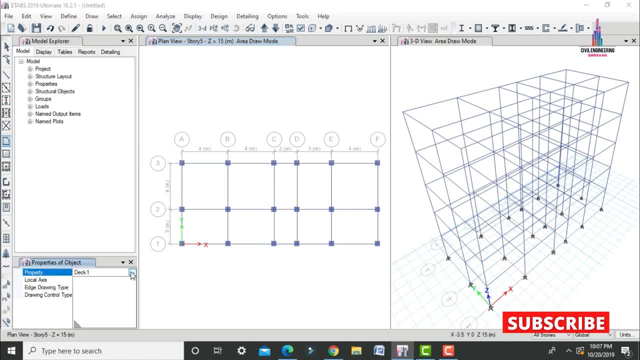 okay, select this option and you have to change the property from deck to change the property from deck. to change the property from deck to slab here, so it will be consisting of slab slab here, so it will be consisting of slab slab here, so it will be consisting of slab 150. now select first two point select. 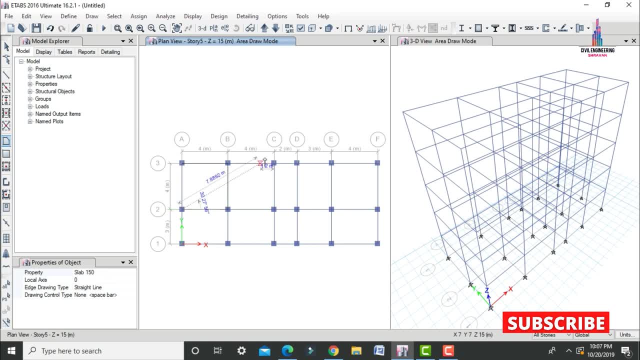 150 now. select first two point. select 150 now. select first two point. select second point here again. select third second point here again. select third second point here again. select third point again. click on fourth point here. point again. click on fourth point here. point again. click on fourth point here. okay again, come to the first point. so it 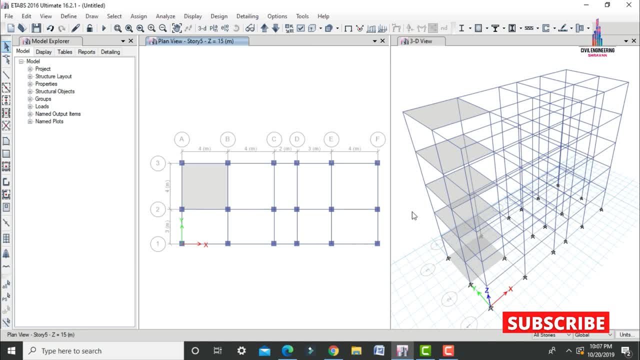 okay again. come to the first point. so it. okay again. come to the first point. so it will assign your respected property of. will assign your respected property of. will assign your respected property of slab here, like this: okay, so this is the slab here. like this: okay, so this is the. 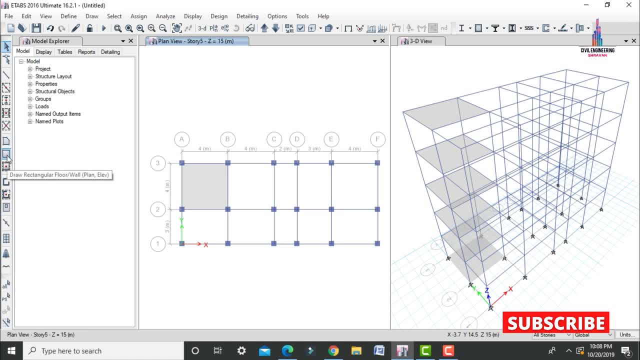 slab here like this. okay, so this is the first method and second method is first method and second method is first method and second method is drawing the rectangular floors. okay, so, drawing the rectangular floors. okay, so, drawing the rectangular floors, okay. so for that, initially we need to select. 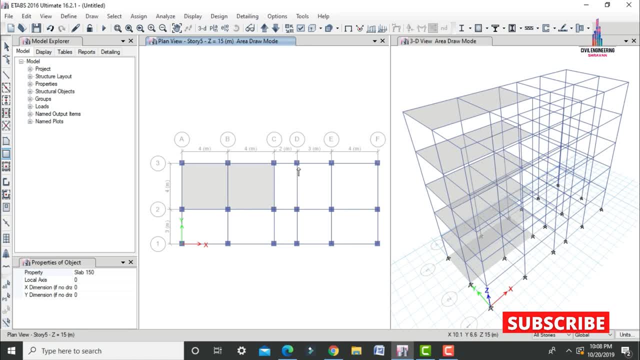 for that initially. we need to select for that initially. we need to select the one node point again. we had to drag the one node point again. we had to drag the one node point again. we had to drag to the respective second node point. okay, to the respective second node point, okay. 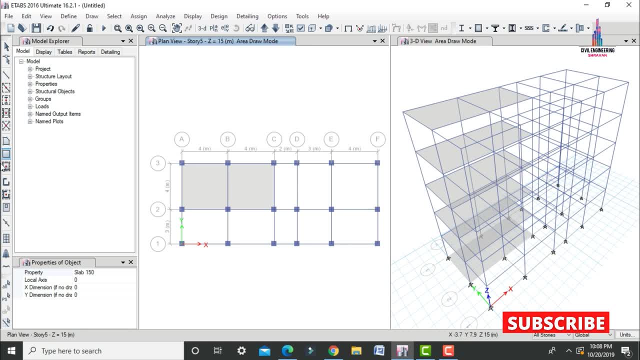 to the respective second node point. okay, in the same way we have third method. in the same way we have third method. in the same way we have third method option also there. so that is related to option also there. so that is related to option also there. so that is related to the quick draw floors option. so select. 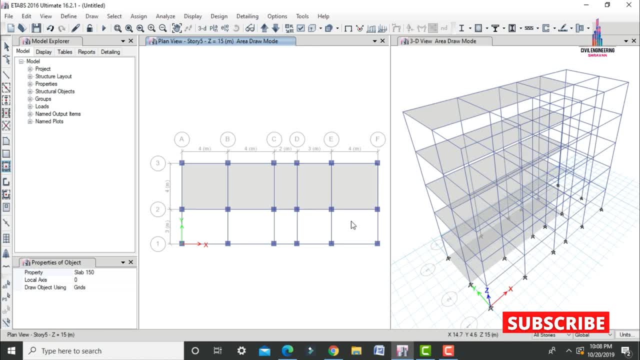 the quick draw floors option. so select the quick draw floors option. so select this point again. select next point again. this point again. select next point again. this point again. select next point again. select next point again. select next. select next point again. select next. select next point again. select next point again. select next point again come. 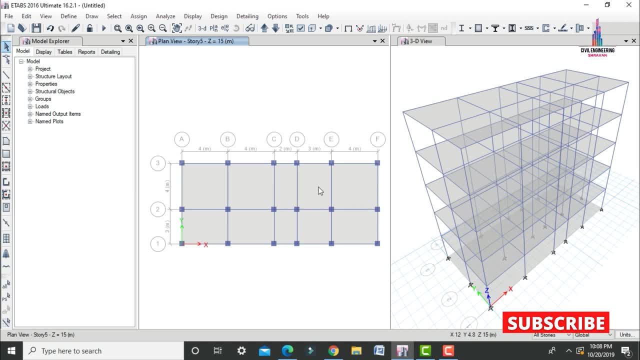 point again. select next point again. come point again. select next point again. come to the first point. okay, so this is the to the first point. okay, so this is the to the first point. okay, so this is the procedure to assign the slab section for. procedure to assign the slab section for. 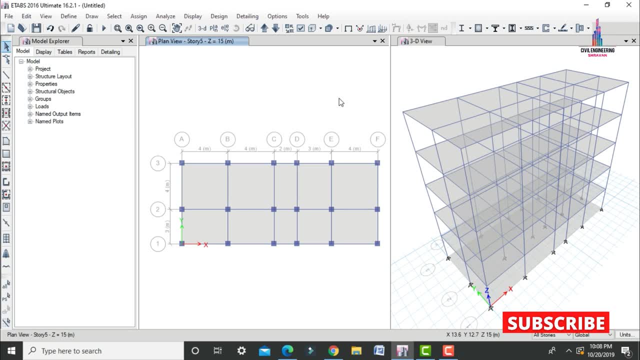 procedure to assign the slab section for the building: okay. so after assigning the the building: okay. so after assigning the the building: okay. so after assigning the slab section, we have to delete all the slab section. we have to delete all the slab section. we have to delete all the properties at the base for this. 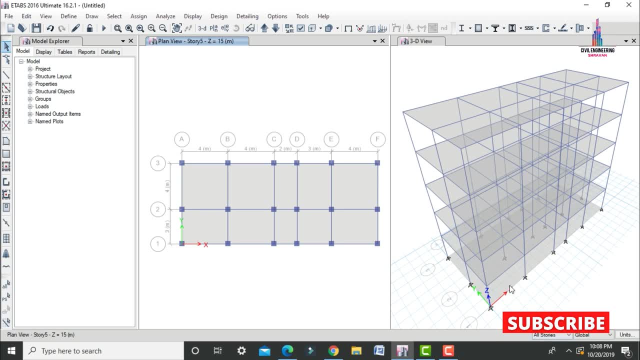 properties at the base for this, properties at the base for this respected building. why? because it was respected building. why? because it was respected building? why? because it was assigned, with the slab sections at the assigned, with the slab sections at the assigned, with the slab sections at the base. we need to delete the respected 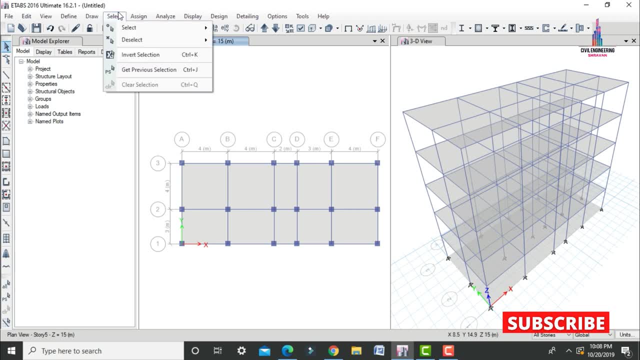 base. we need to delete the respected base. we need to delete the respected properties. okay, so go to select option properties. okay, so go to select option properties. okay, so go to select option here. select so select here. go to select here. select so select here. go to select. 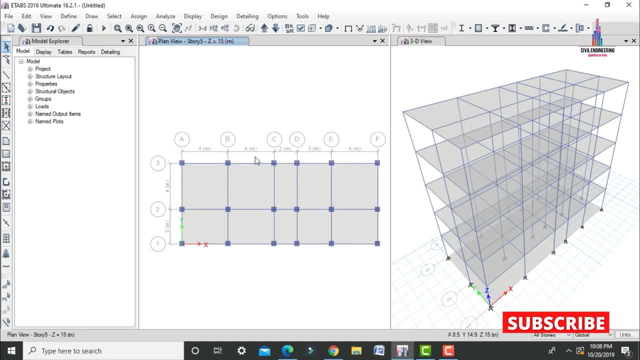 here select, so select. here go to select. to bright, so go to select by stories. to bright, so go to select by stories. to bright, so go to select by stories here. so here we have to select the base here. so here we have to select the base here. so here we have to select the base. click on select option so it will select. 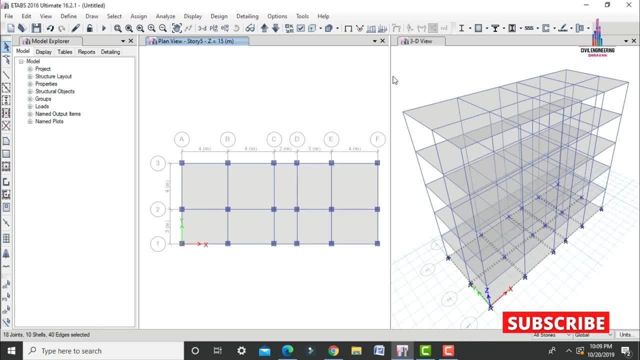 click on select option so it will select. click on select option so it will select all the properties at the base for this, all the properties at the base for this, all the properties at the base for this building. now we have to click on delete building. now we have to click on delete. 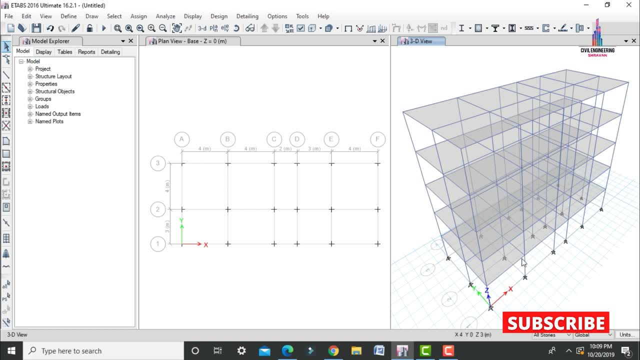 building. now we have to click on delete option, so it will delete all your option. so it will delete all your option. so it will delete all your properties at the base for this building properties at the base for this building properties at the base for this building, here, like this: so after assigning the 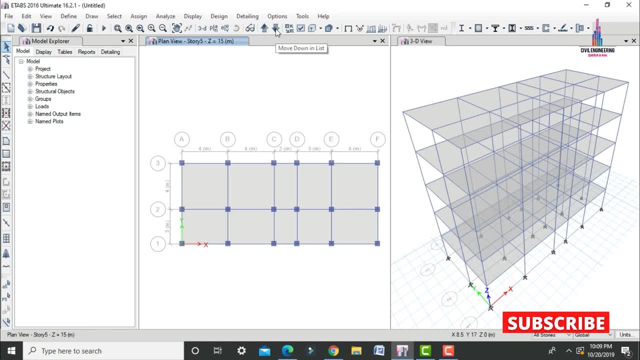 here, like this: so after assigning the here, like this: so after assigning the properties for the structure initially, we properties for the structure initially, we properties for the structure initially. we need to see this model in rendering, need to see this model in rendering, need to see this model in rendering view. okay, so for that we need to click on. 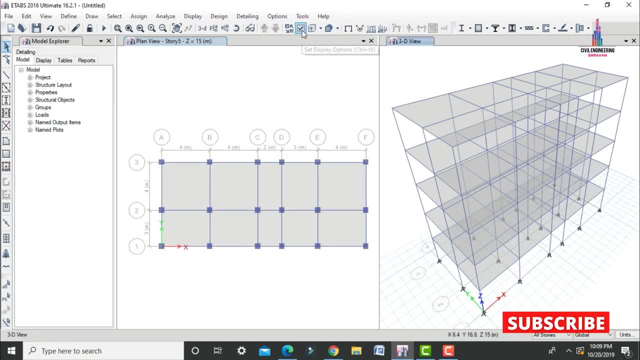 view. okay, so for that we need to click on view. okay, so for that we need to click on the rendering view option here. so select the rendering view option here. so select the rendering view option here. so select the right mark here on the top of the, the right mark here on the top of the. 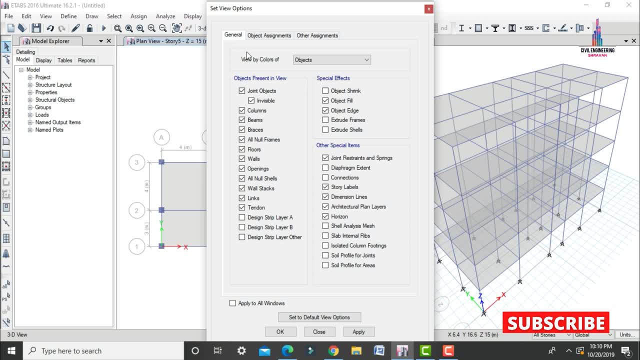 the right mark here on the top of the building, so select this. so in this we building, so select this. so in this we building, so select this. so in this we need to select the object to fill, need to select the object to fill, need to select the object to fill options and extrude shells and extrude. 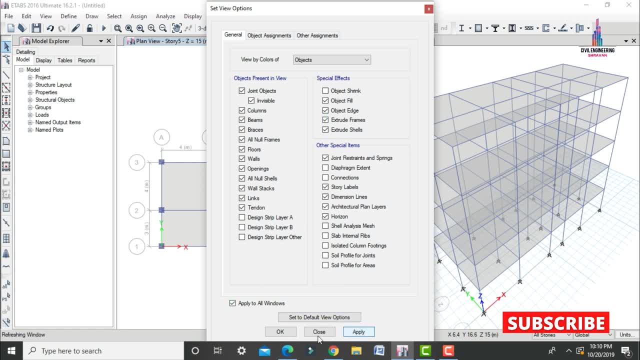 options and extrude shells. and extrude options and extrude shells and extrude frames. apply to all windows here. frames apply to all windows here. frames apply to all windows here: apply okay here. okay, now we can see the. apply okay here. okay, now we can see the. 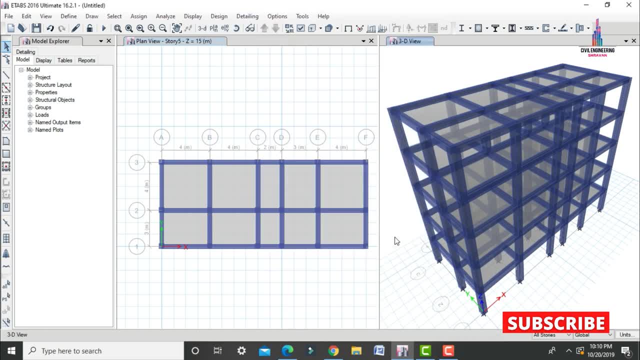 apply: okay here. okay, now, we can see: the building model was open here, like this building model was open here, like this building model was open here, like this: which is consisting of your expected 0.3, which is consisting of your expected 0.3, which is consisting of your expected 0.3 cross 0.3 beam size and 0.45 cross 0.45. 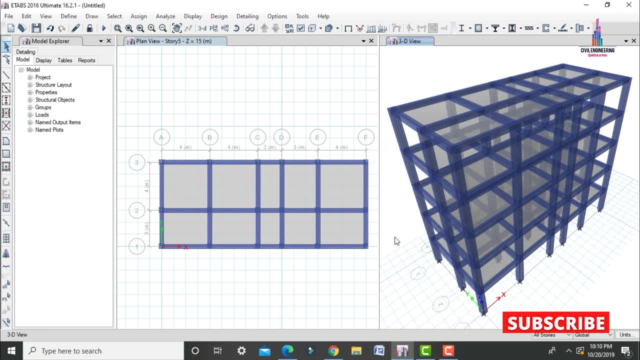 0.45 cross. 0.45 is the column size and clap thickness is the column size and clap thickness is the column size, and clap thickness will be consisting of 150 mm. okay, so will be consisting of 150 mm. okay, so will be consisting of 150 mm. okay, so after modeling process completed, we need: 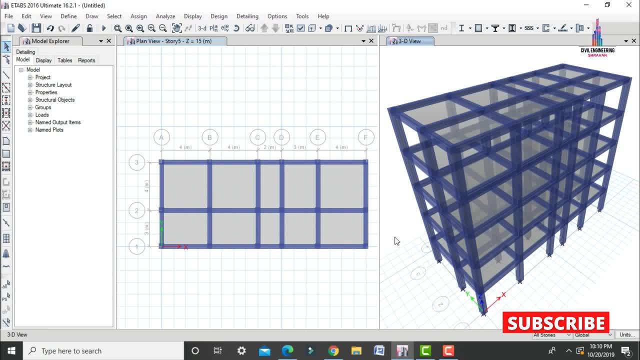 after modeling process completed, we need, after modeling process completed, we need to apply the load cases for this, to apply the load cases for this, to apply the load cases for this respected structure, basically for respected structure, basically for respected structure, basically for designing of this respected building. i am 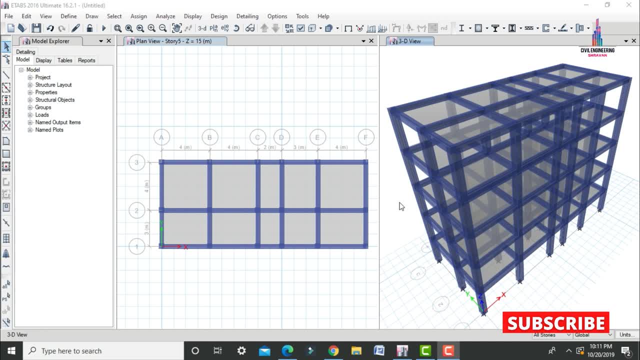 designing of this respected building. i am designing of this respected building. i am considering the load cases which are considering the load cases which are considering the load cases which are related to the dead loading condition. related to the dead loading condition. related to the dead loading condition, live loading condition, seismic loading. 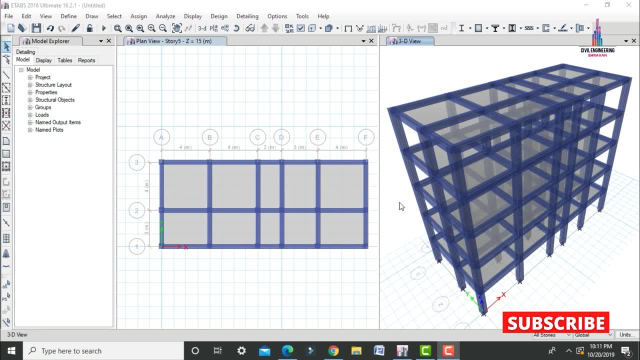 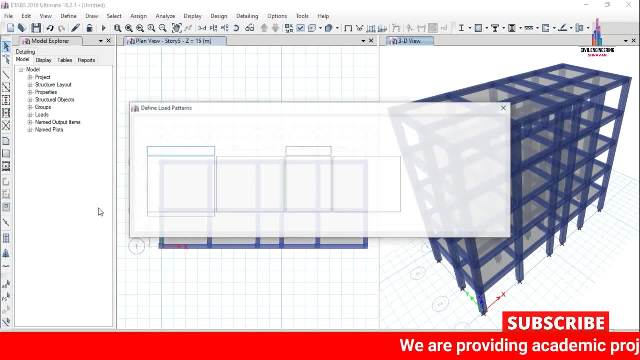 live loading condition, seismic loading- live loading condition, seismic loading condition, as well as wind loading as well as wind loading option. okay, so here it was already added option. okay, so here it was already added option. okay, so here it was already added- with dead loading condition as well as. 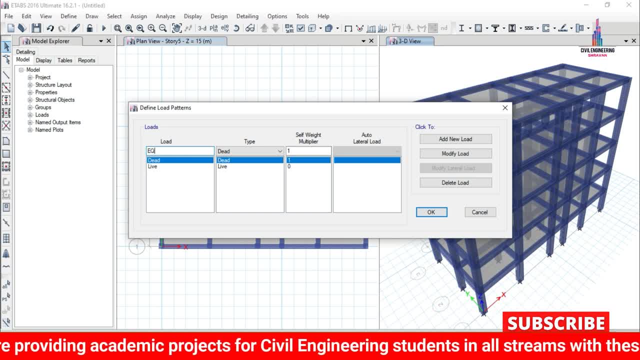 with dead loading condition as well as with dead loading condition as well as live loading condition. so initially i am live loading condition, so initially i am live loading condition. so initially i am taking the next load case is earthquake taking the next load case is earthquake taking the next load case is earthquake load which is in x direction condition. 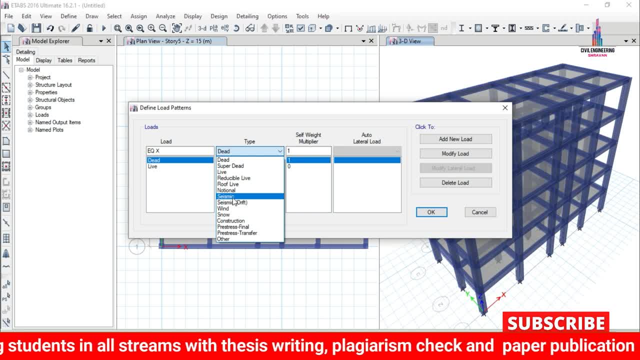 load which is in x direction condition, load which is in x direction condition. now we have to select the type here. now we have to select the type here. now we have to select the type here which is related to the seismic loading, which is related to the seismic loading. 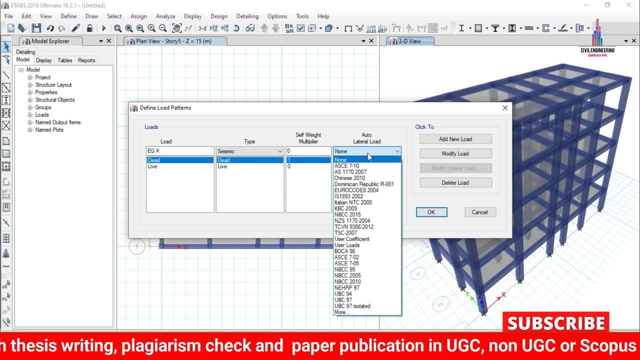 which is related to the seismic loading condition, and we have to select the is condition and we have to select the is condition and we have to select the is code from the auto lateral load code, from the auto lateral load code, from the auto lateral load combination. so here i am selecting is. 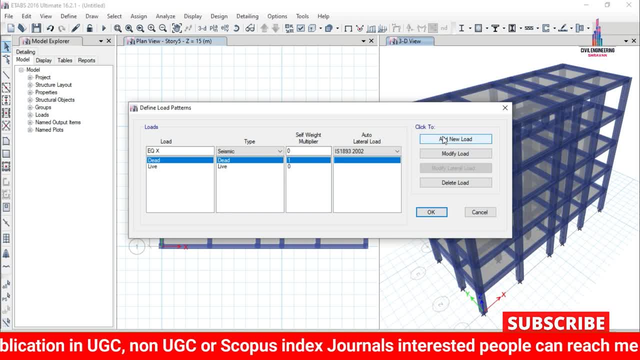 combination. so here i am selecting is combination. so here i am selecting is code which is related to the 1893 2002 code, which is related to the 1893 2002 code, which is related to the 1893 2002. click on add property now in the same. 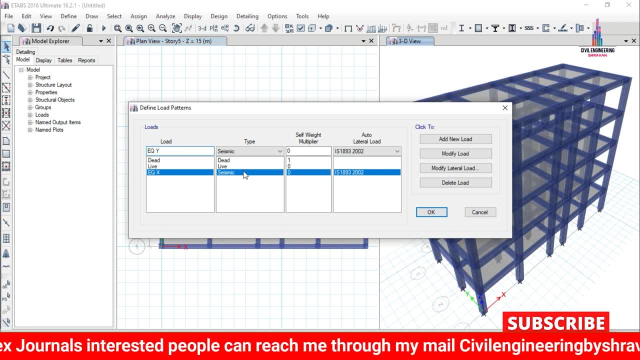 click on add property now. in the same click on add property now. in the same way we have to add earthquake load. which way we have to add earthquake load? which way we have to add earthquake load, which is in y direction condition, so click on, is in y direction condition, so click on. 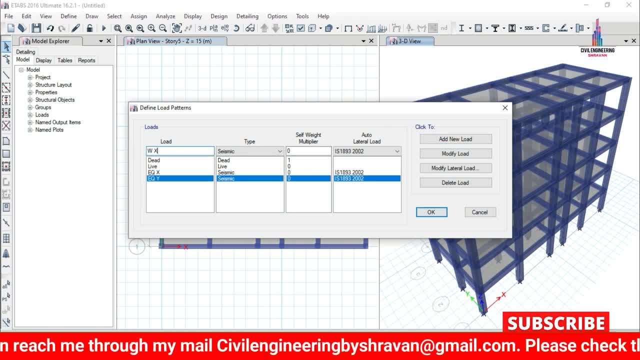 is in y direction condition, so click on add button. now i am entering the wind add button. now i am entering the wind add button. now i am entering the wind loading x direction condition. now here we loading x direction condition. now here we loading x direction condition. now here we have to select the title as win. 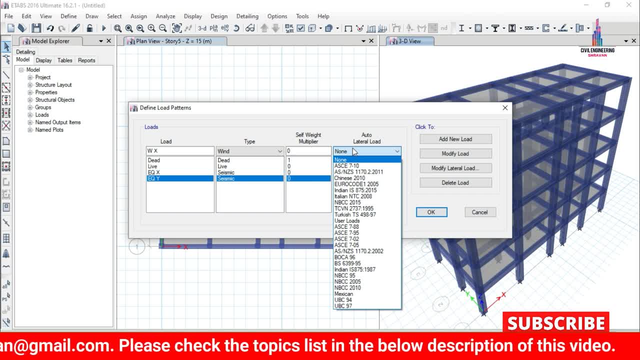 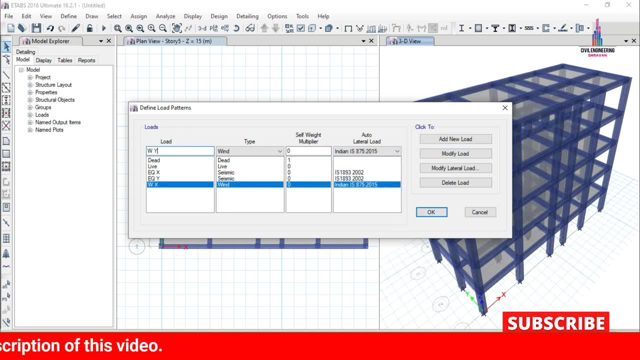 indian standard system of 875 2015. indian standard system of 875 2015. click on add. in a same way, we have to click on add. in a same way. we have to click on add. in a same way, we have to add the load, which is in y direction. 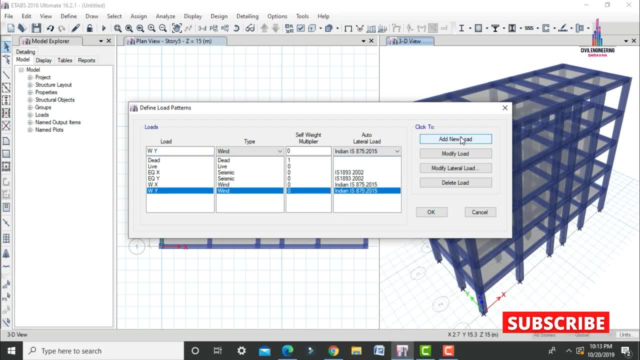 add the load which is in y direction. add the load which is in y direction. condition: condition: condition. okay. so, after adding the properties, we okay. so, after adding the properties, we okay. so, after adding the properties, we need to modify the data which is related. okay, so, after adding the properties, we need to modify the data which is related. 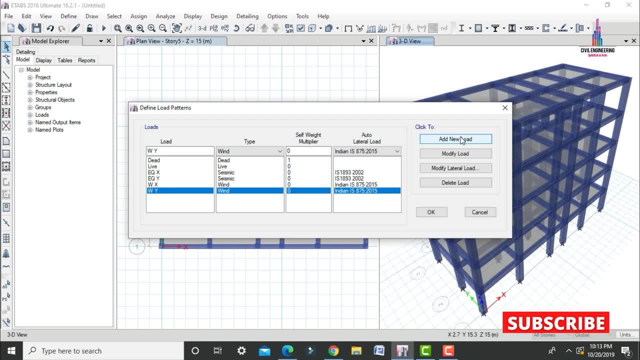 okay, so after adding the properties, we need to modify the data which is related to the seismic loading condition as well as to the seismic loading condition, as well as to the seismic loading condition as well as wind loading condition, basically seismic wind loading condition, basically seismic wind loading condition, basically seismic load. i was considered as per the is code. 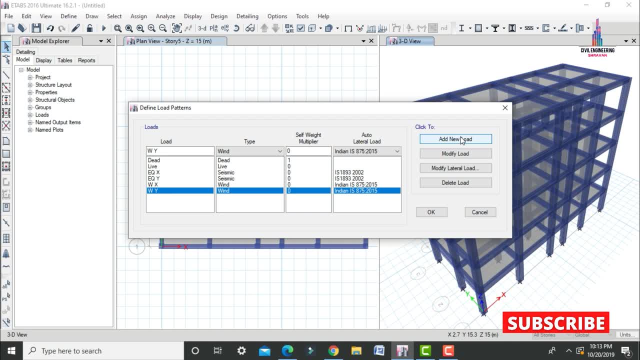 load i was considered as per the is code. load i was considered as per the is code which is related to the 1893 code. so as which is related to the 1893 code, so as which is related to the 1893 code. so, as per the is code, it was suggested that. 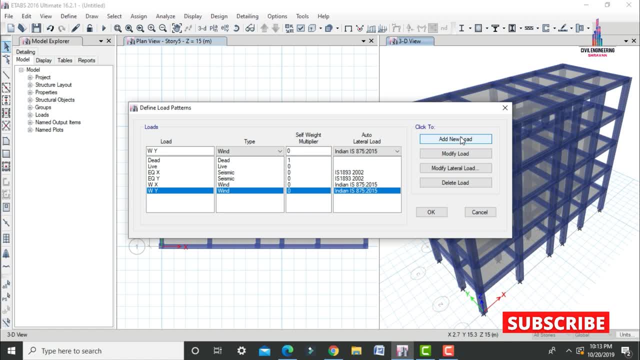 per the is code. it was suggested that. per the is code, it was suggested that the number of zones will be consisting of: the number of zones will be consisting of: the number of zones will be consisting of four, which is equals to zone 2, zone 3, zone. four: zone 3, zone 4, zone 5, which is having the coefficient 4, zone 5, which is having the coefficient 4, zone 5, which is having the coefficient factor of 0.1, 0.16, 0.24 and 0.36. you can. factor of 0.1, 0.16, 0.24 and 0.36. you can factor of 0.1, 0.16, 0.24 and 0.36. you can select any one of the zone as per your. 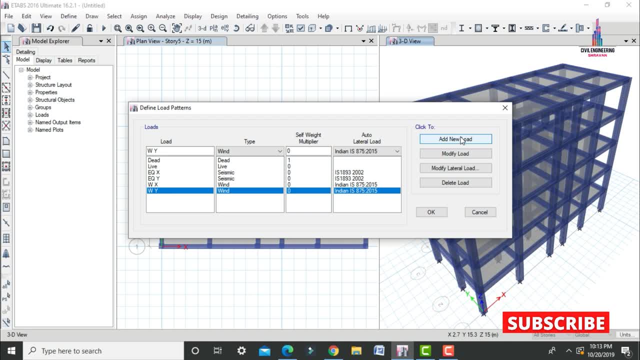 select any one of the zone as per your. select any one of the zone as per your considerations. so here i am considering considerations. so here i am considering considerations. so here i am considering the zone 5 condition which is placed in. the zone 5 condition which is placed in. 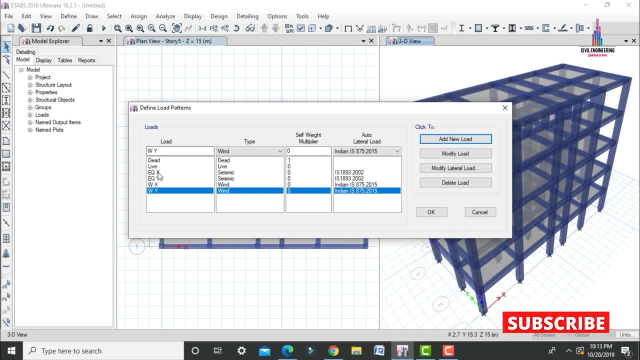 the zone 5 condition which is placed in medium soil condition. so select epic medium soil condition. so select epic medium soil condition. so select epic load which is in x direction condition load which is in x direction condition load which is in x direction condition. so here we have to click on modify. 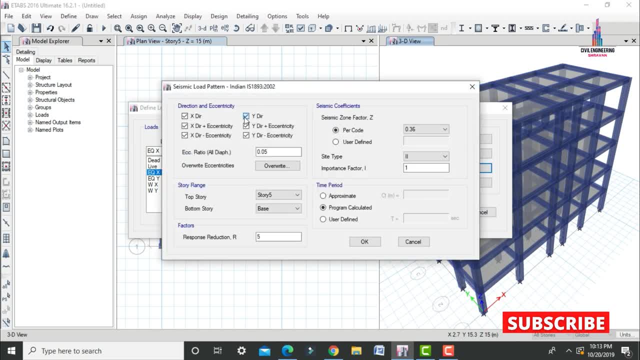 so here we have to click on modify. so here we have to click on modify lateral load option. lateral load option. lateral load option. select x direction load case: only here. select x direction load case- only here. select x direction load case: only here. so select x direction load case again. we. 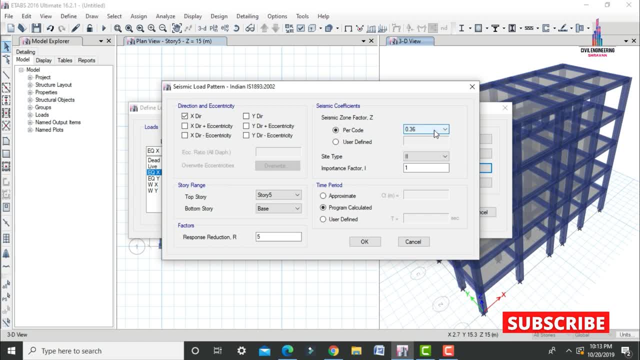 so select x direction load case again. we so select x direction load case again we have to select the per code value is 0.36. have to select the per code value is 0.36. have to select the per code value is 0.36. so click on. soil type is 2. again click on. 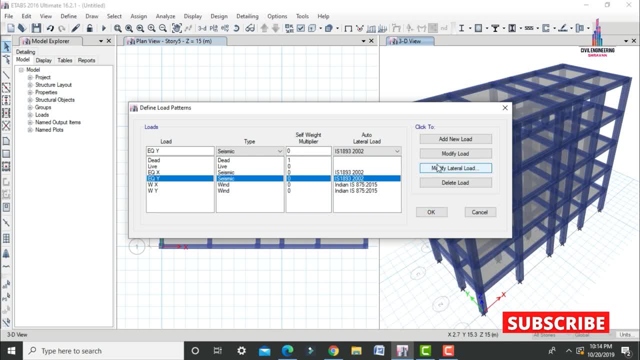 so click on soil type is 2, again click on. so click on soil type is 2, again click on ok option. in the same way, we have to ok option. in the same way we have to ok option. in the same way we have to select y direction. modify lateral load in. 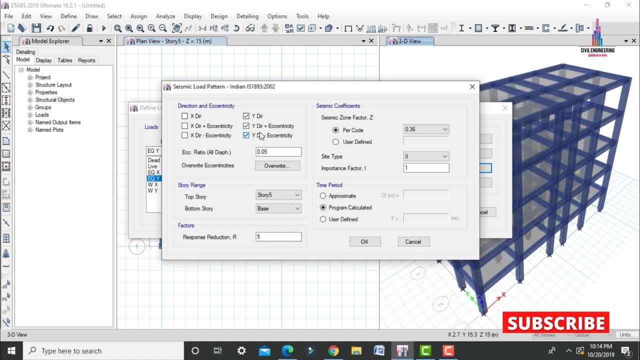 select y direction. modify lateral load in. select y direction, modify lateral load in the same way. select in y direction the same way. select in y direction the same way. select in y direction. condition only again. we have to select condition only again. we have to select condition only again. we have to select the per code value 0.36. so click on ok. 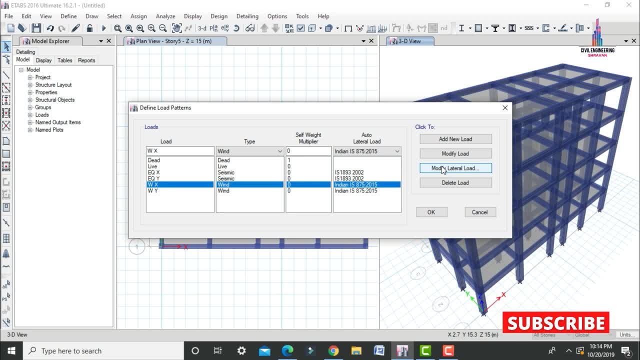 the per code value 0.36, so click on ok. the per code value 0.36, so click on ok. now i am selecting the wind load which now i am selecting the wind load which. now i am selecting the wind load which is in x direction. condition modify. 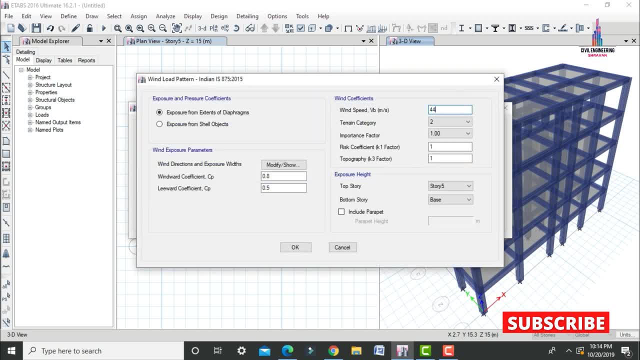 is in x direction. condition modify is in x direction. condition modify- lateral load. now, here we have to enter lateral load. now, here we have to enter lateral load. now, here we have to enter the basic wind speed value, and which is the basic wind speed value and which is: 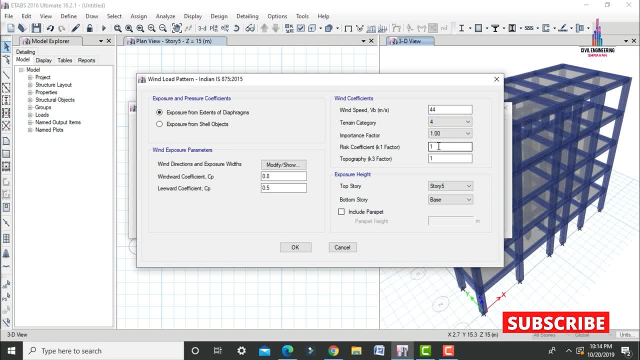 the basic wind speed value and which is consisting of your different types of, consisting of your different types of, consisting of your different types of terrains like this. so select any one of terrains like this. so select any one of terrains like this. so select any one of the terrain here. and importance factor. 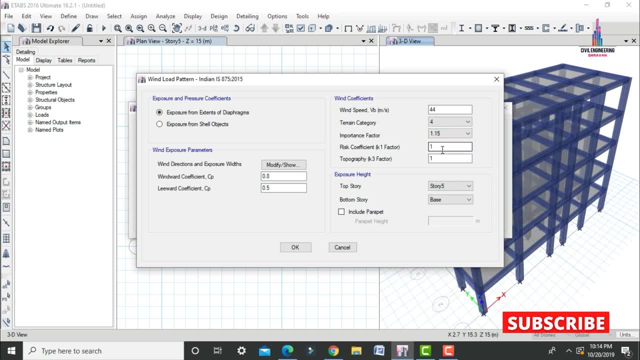 the terrain here and importance factor. the terrain here and importance factor. just i'm considering it as 1.15, just i'm considering it as 1.15, just i'm considering it as 1.15. and this coefficient is one typographic and this coefficient is one typographic. 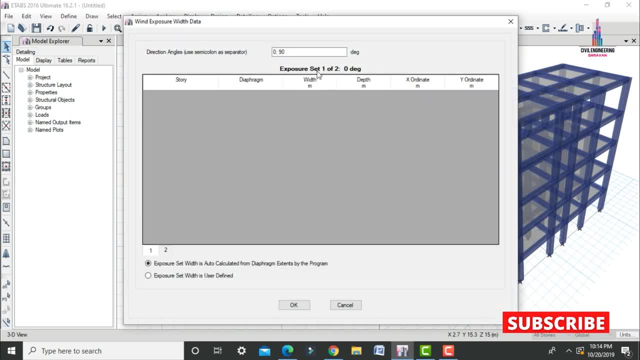 and this coefficient is one. typographic coefficient is one. okay, so click on. coefficient is one. okay, so click on. coefficient is one. okay, so click on modify show option here. so here we have modify show option here. so here we have modify show option here. so here we have to select the angle of. 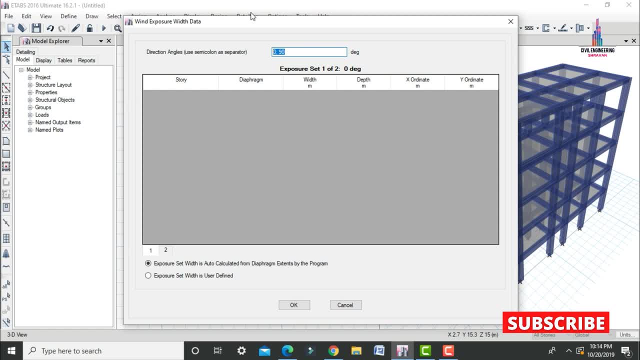 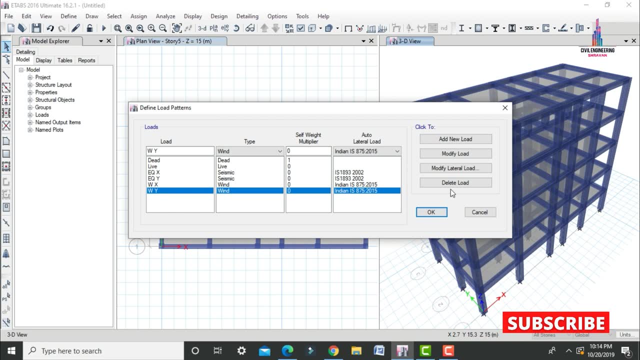 to select the angle of, to select the angle of direction for the wind load, so x direction for the wind load, so x direction for the wind load, so x direction. just i'm taking with angle is direction, just i'm taking with angle is direction, just i'm taking with angle is which is comes under your respected. 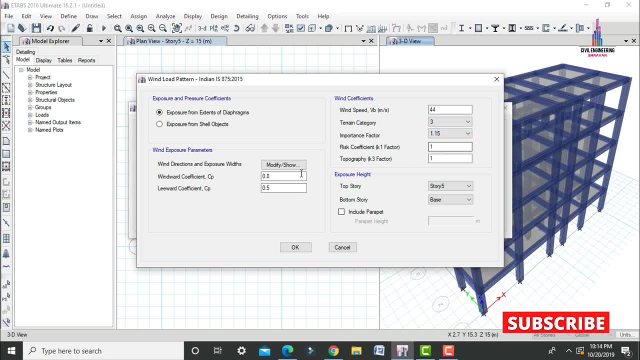 which is comes under your respected, which is comes under your respected terrain: category 3, which is having 1.15 terrain, category 3, which is having 1.15 terrain. category 3, which is having 1.15. and we have to click on modify show. 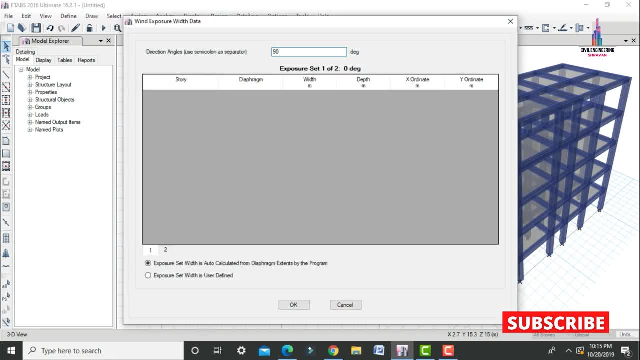 and we have to click on modify show and we have to click on modify show option. again, again in the same way. we option, again, again in the same way. we option again, again, in the same way: we have to enter the, have to enter the, have to enter the y direction. we already know. x direction is. 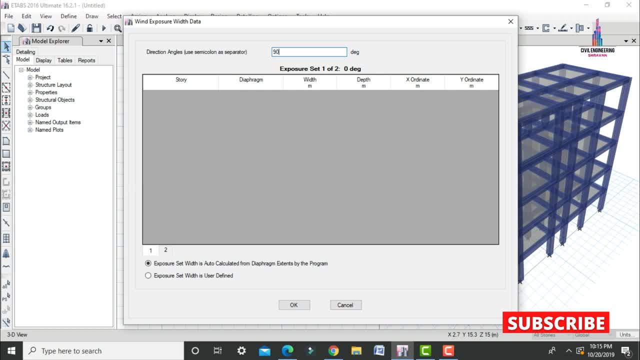 y direction. we already know x direction is y direction. we already know x direction is always perpendicular to y direction, always perpendicular to y direction, always perpendicular to y direction. so that's why i'm taking it as it has. so that's why i'm taking it as it has. 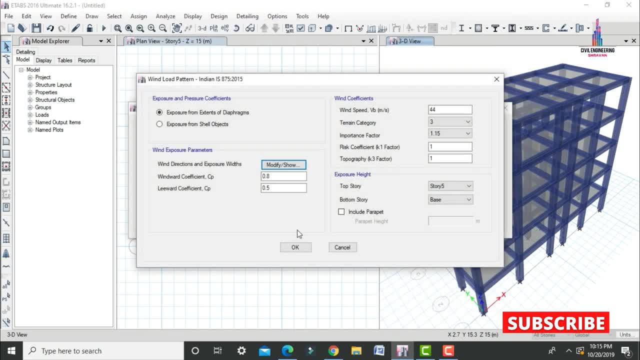 so that's why i'm taking it. as it has 90 degrees, click on ok. so after that we 90 degrees, click on ok. so after that we 90 degrees, click on ok. so after that we have to click on ok option. so here i was. have to click on ok option, so here i was have to click on ok option, so here i was. define the load cases which is related. define the load cases which is related. define the load cases which is related to the dead loading condition lie to the dead loading condition lie. 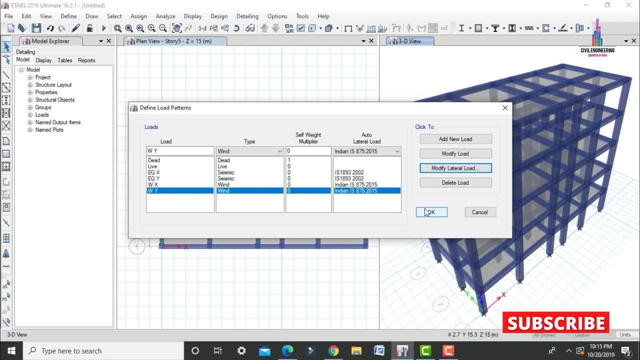 to the dead loading condition, lie loading condition as well as seismic loading condition, as well as seismic loading condition as well as seismic loading and wind loading condition. now loading and wind loading condition. now loading and wind loading condition. now we have to assign those properties. or we have to assign those properties, or 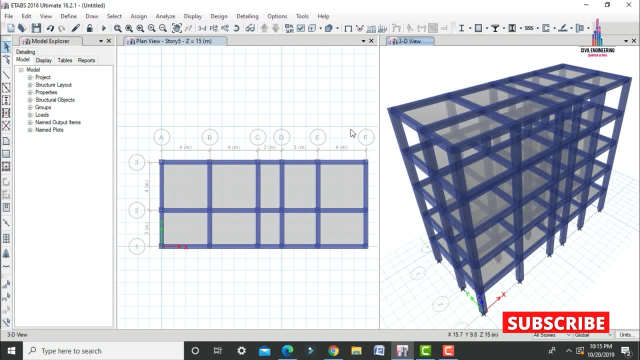 we have to assign those properties or assign those load cases for this building. assign those load cases for this building, assign those load cases for this building. so initially we need to apply the. so initially we need to apply the. so initially we need to apply the dead load for this structure. 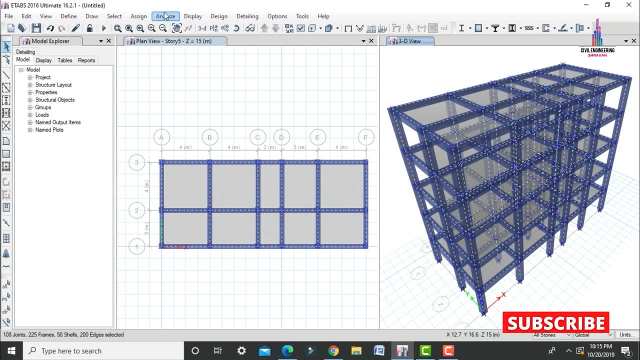 dead load for this structure. dead load for this structure. so initially i am selecting all the so initially i am selecting all the so initially i am selecting all the building here, so click on assign option. building here, so click on assign option. building here, so click on assign option. so here we have to select the joint. 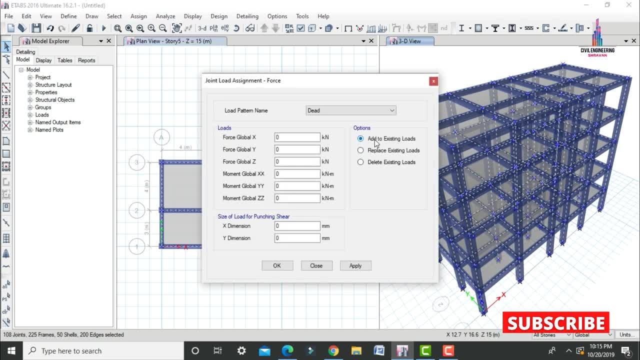 so here we have to select the joint. so here we have to select the joint loads, select the forces. here again we loads. select the forces. here again we loads. select the forces. here again we have to select the add to existing loads. have to select the add to existing loads. 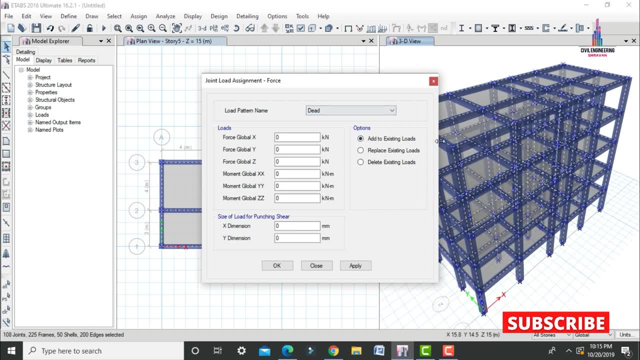 have to select the add to existing loads option. it will be consisting of three option. it will be consisting of three option. it will be consisting of three options here, which is related to the add options here, which is related to the add options here, which is related to the add to existing and replace existing, and. 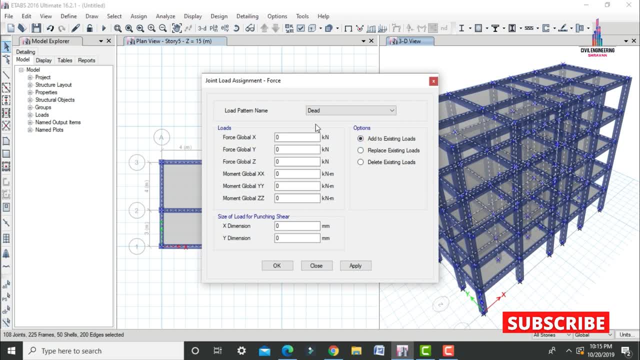 to existing and replace existing, and to existing and replace existing and delete existing. okay. so if you want to delete existing, okay. so, if you want to delete existing, okay. so if you want to add new one, you need to click on add. to add new one, you need to click on add to. 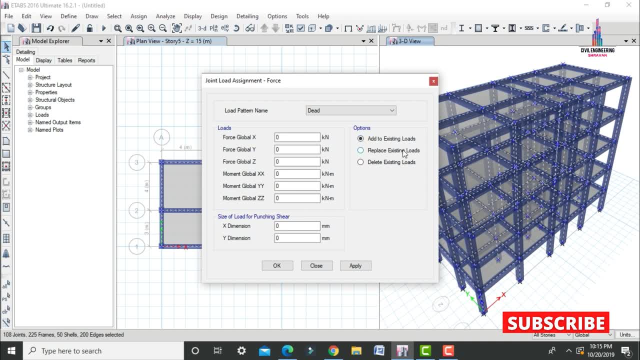 add new one. you need to click on add to existing load cases or if you want to existing load cases, or if you want to existing load cases, or if you want to replace the existing load with new. replace the existing load with new. replace the existing load with new intensity. you can select the second. 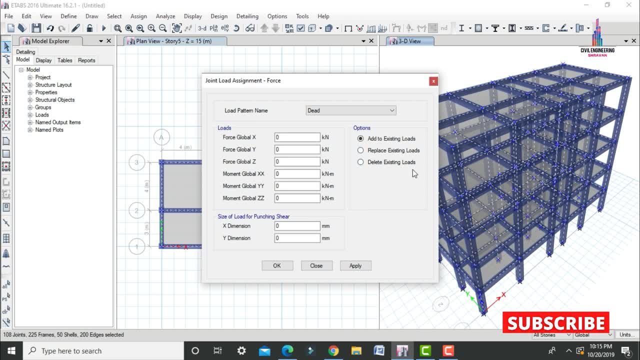 intensity: you can select the second intensity. you can select the second option otherwise, if you want to delete option otherwise, if you want to delete option otherwise, if you want to delete the intensity, you can select the last. the intensity: you can select the last. the intensity: you can select the last one. so here i'm selecting: add to. 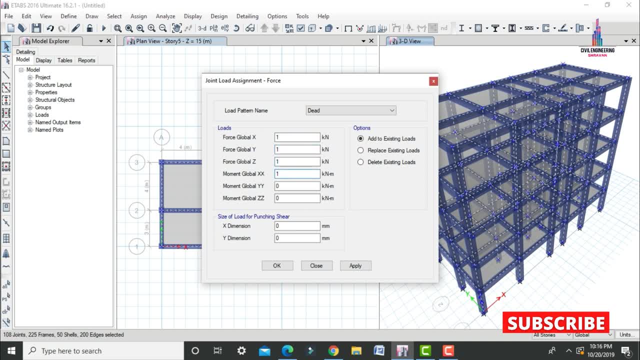 one. so here i'm selecting add to one. so here i'm selecting add to existing. why? because i'm adding the new existing. why because i'm adding the new existing? why? because i'm adding the new load cases here, which is having the load cases? here, which is having the 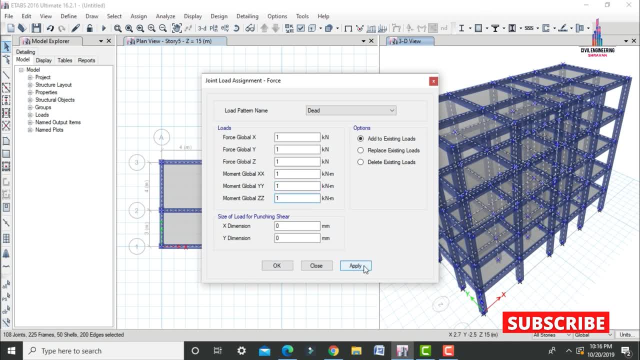 load cases here, which is having the factor of coefficient as one, one, one, one. factor of coefficient as one, one, one, one. factor of coefficient as one, one, one, one, one. click on apply. click on ok option. so click on apply. click on ok option. so click on apply. click on ok option, so it will apply your respective system. 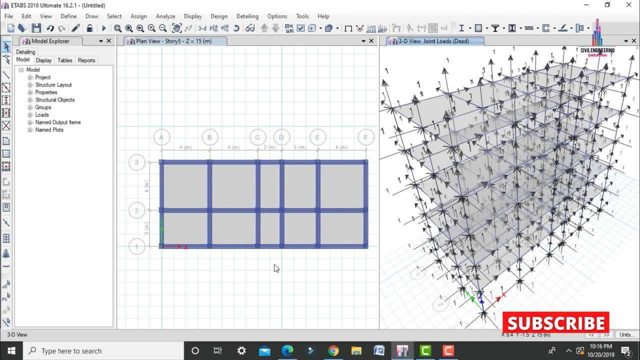 it will apply your respective system. it will apply your respective system. sorry self weight for this respective sorry self weight for this respective sorry self weight for this respective structure. so after that, we had to structure. so after that, we had to structure. so after that, we had to apply the dead load condition for the. 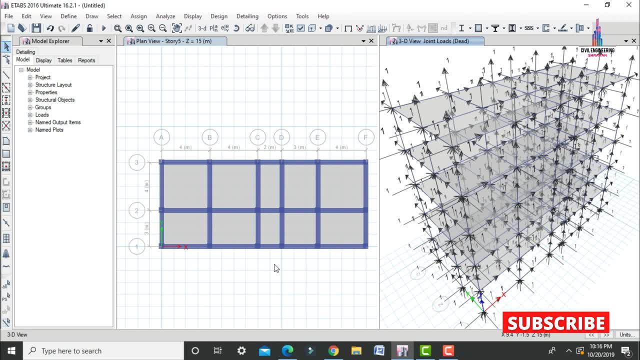 apply the dead load condition for the. apply the dead load condition for the beam. dead load condition for the column beam. dead load condition for the column beam. dead load condition for the column. dead load condition for the slab, so we. dead load condition for the slab, so we. 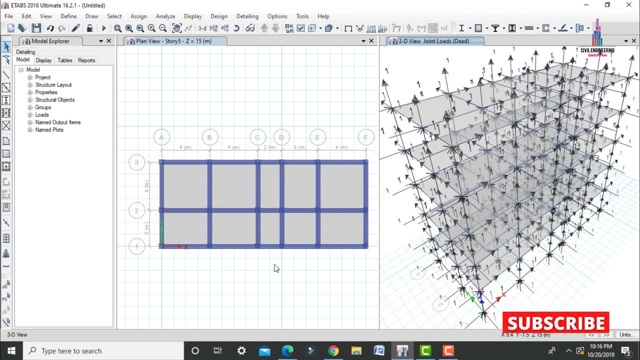 dead load condition for the slab. so we are already assigned the self weight, so are already assigned the self weight, so are already assigned the self weight, so that self weight is only related to the, that self weight is only related to the, that self weight is only related to the joint member load. okay, so joint, that is. 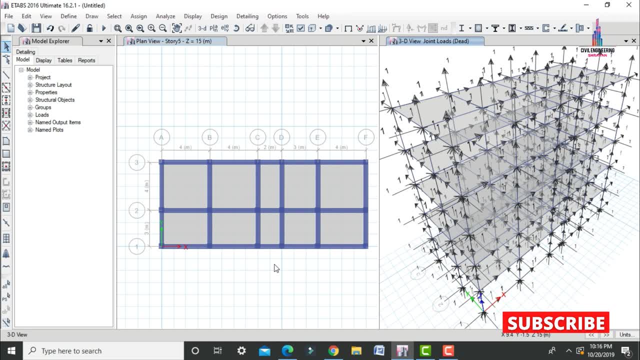 joint member load. okay, so joint, that is joint member load. okay, so joint, that is only related to the joint load. okay, now, only related to the joint load. okay, now, only related to the joint load. okay, now we have to add the member load for. we have to add the member load for. 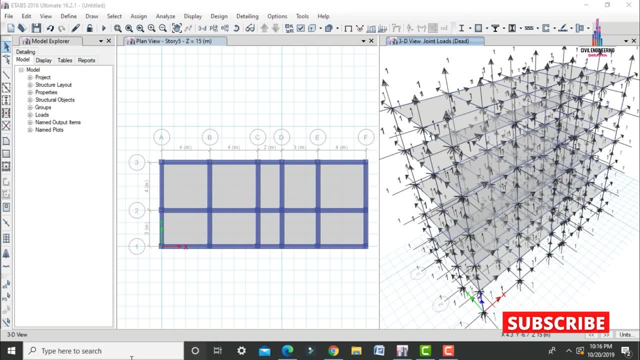 we have to add the member load for individual members. so initially we need individual members. so initially we need individual members. so initially we need to calculate the intensity of the load. to calculate the intensity of the load. to calculate the intensity of the load. okay, as per the considerations we need to. 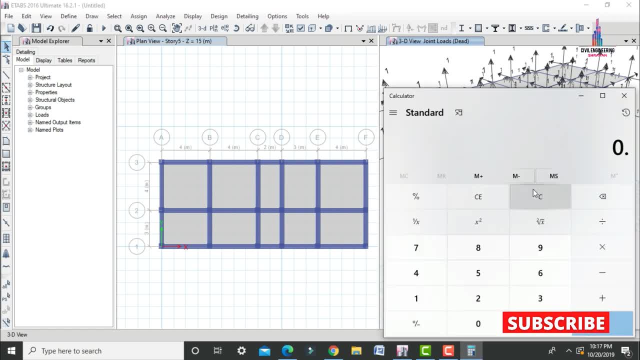 okay, as per the considerations we need to. okay, as per the considerations, we need to calculate the intensity of the load, calculate the intensity of the load, calculate the intensity of the load. so here i am taking the dimensions of. so here i am taking the dimensions of. so here i am taking the dimensions of the beam as 0.35 cross 0.35. 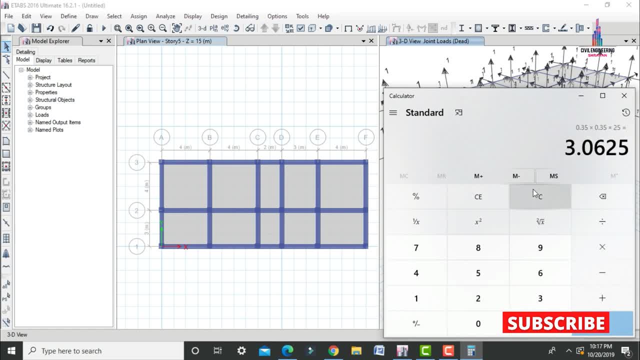 the beam as 0.35 cross 0.35, the beam as 0.35 cross 0.35. we have to multiply this respected value. we have to multiply this respected value. we have to multiply this respected value with 25, so it will give the intensity of. 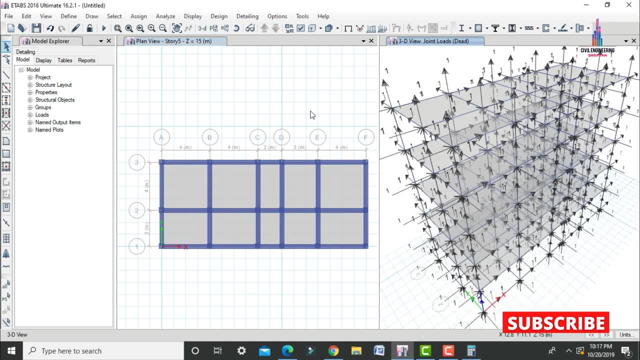 with 25, so it will give the intensity of with 25, so it will give the intensity of 3.0625. we had to initially select 3.0625. we had to initially select 3.0625. we had to initially select beams, select by properties. now here we. 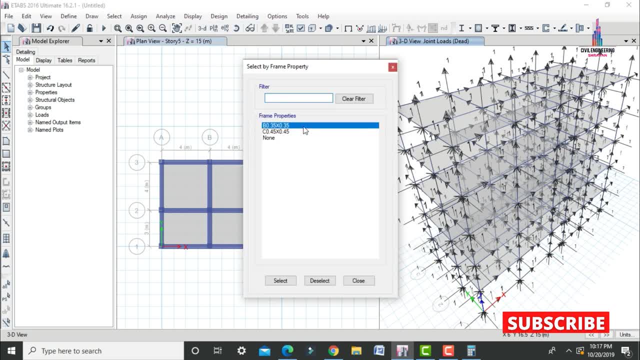 beams select by properties. now, here we beams: select by properties. now, here we have to select the frame sections. have to select the frame sections. have to select the frame sections. so select the beam which is consisting. so select the beam which is consisting. so select the beam which is consisting of 0.35, cross 0.35. 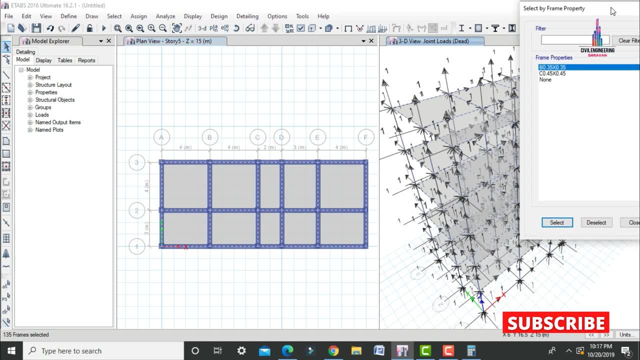 of 0.35 cross 0.35 of 0.35 cross- 0.35. click on select. it will select all your click on select. it will select all your click on select. it will select all your members here. like this, we have to. 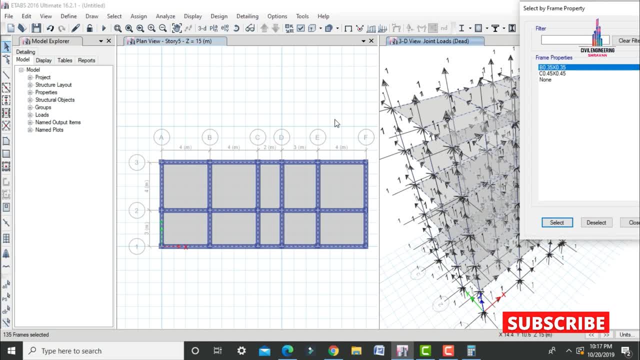 members here like this. we have to members here like this. we have to assign the 3.0625 load for this members. assign the 3.0625 load for this members. assign the 3.0625 load for this members only. so click on assign option here. 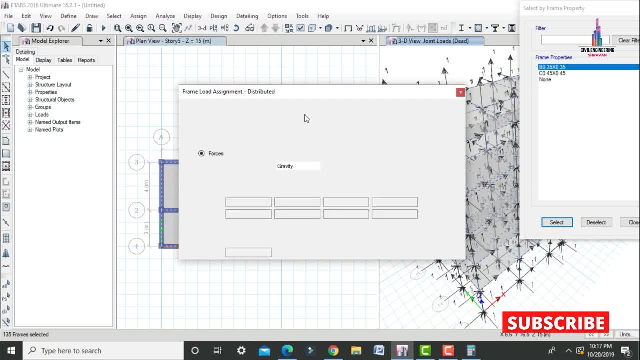 only so click on assign option here. only so click on assign option here. select frame loads. select distributed select frame loads. select distributed select frame loads. select distributed load. and we have to select add to load. and we have to select add to load and we have to select add to existing load. in this we need to enter: 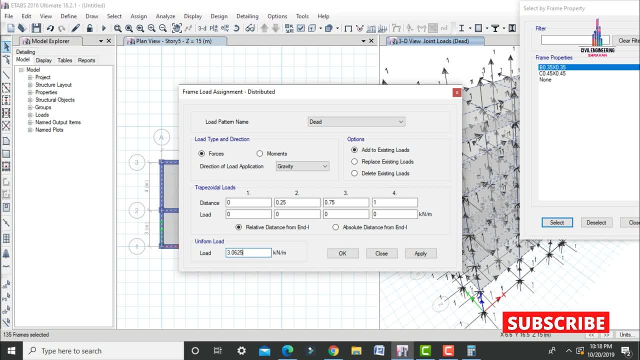 existing load in this, we need to enter existing load. in this, we need to enter the intensity of 3.0625. the intensity of 3.0625, the intensity of 3.0625. so click on apply. so click on okay, so it. so click on apply. so click on okay, so it. 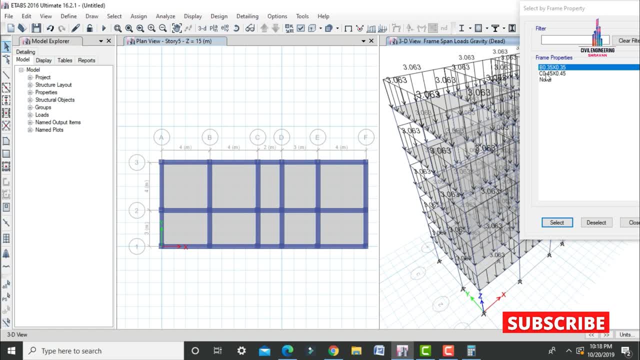 so click on apply. so click on okay. so it will apply your respective dead load for. will apply your respective dead load for. will apply your respective dead load for the beam section. in the same way we have the beam section. in the same way we have the beam section, in the same way we have to select the column here. so it will. 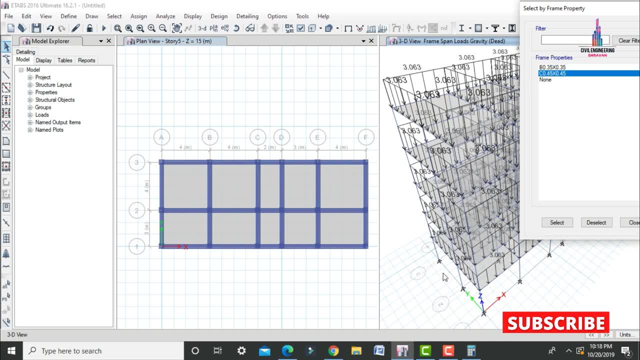 to select the column here, so it will. to select the column here, so it will select all your property which is related. select all your property which is related. select all your property which is related to the column section. now we have to. to the column section. now we have to. 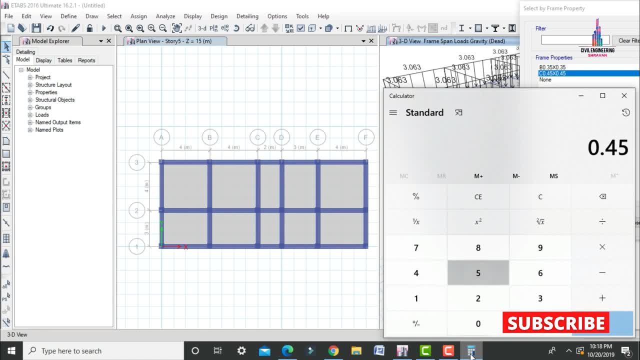 to the column section. now we have to calculate the intensity of the load. which calculate the intensity of the load. which calculate the intensity of the load which is related to the 0.45 cross 0.45 is related to the 0.45 cross 0.45. 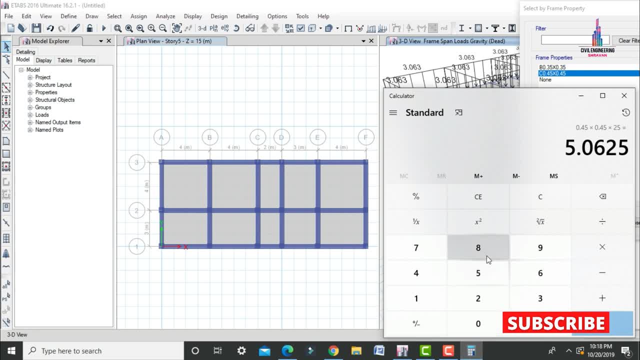 is related to the 0.45 cross. 0.45 multiplied by your 25, so it will give: multiplied by your 25, so it will give: multiplied by your 25, so it will give the intensity of 5.0625 intensity. so the intensity of 5.0625 intensity. so 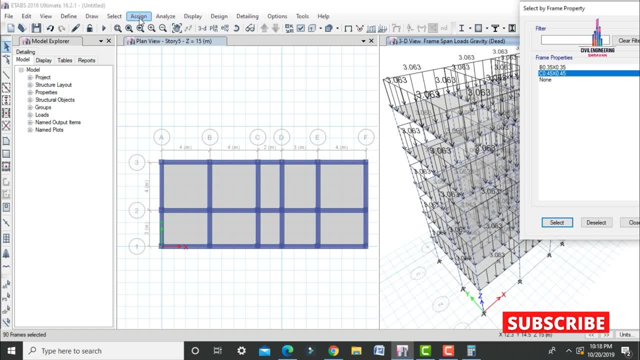 the intensity of 5.0625 intensity. so click on select option here. so we have click on select option here. so we have click on select option here. so we have to go to assign here: select. assign to go to assign here. select. assign to go to assign here. select. assign frame line load: distributed load in this: 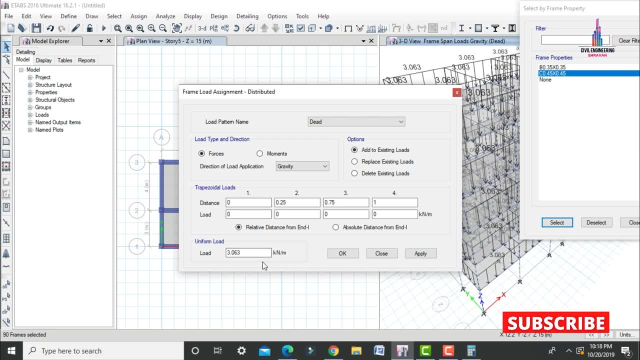 frame line load: distributed load. in this. frame line load distributed load. in this we need to select the dead load, which is. we need to select the dead load which is. we need to select the dead load which is: add to existing load intensity, which is: add to existing load intensity, which is: 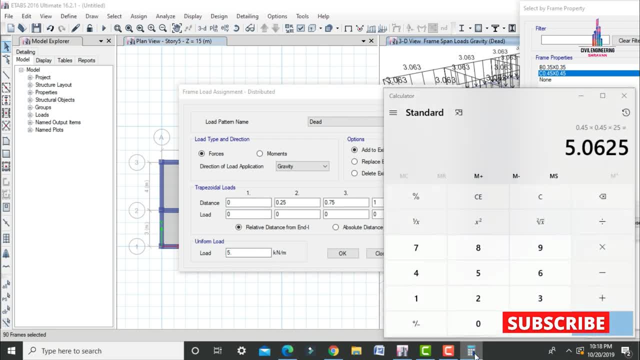 add to existing load intensity, which is having 5.0625. 5.0625 is the intensity we having 5.0625. 5.0625 is the intensity we having 5.0625. 5.0625 is the intensity we need to add for the respected column. 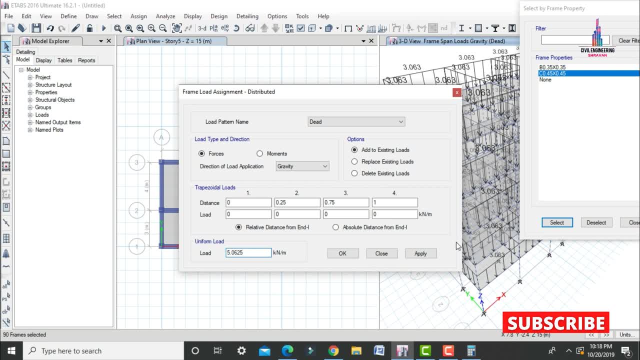 need to add for the respected column. need to add for the respected column: section 5.0625: click on apply option. section 5.0625: click on apply option. section 5.0625. click on apply option. click on. ok, so after adding the column. 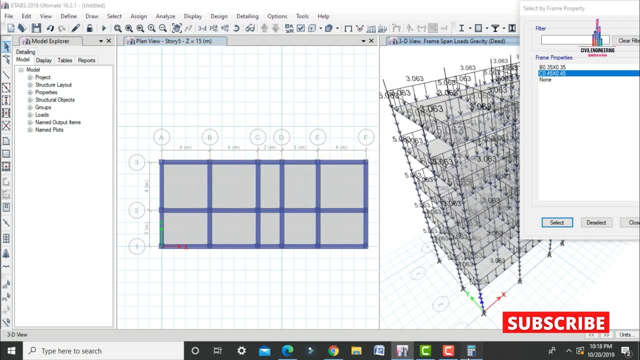 click on ok. so after adding the column, click on ok. so after adding the column dead load, we need to add the slab dead dead load. we need to add the slab dead dead load. we need to add the slab dead load also. we can calculate the respected load also. we can calculate the respected. 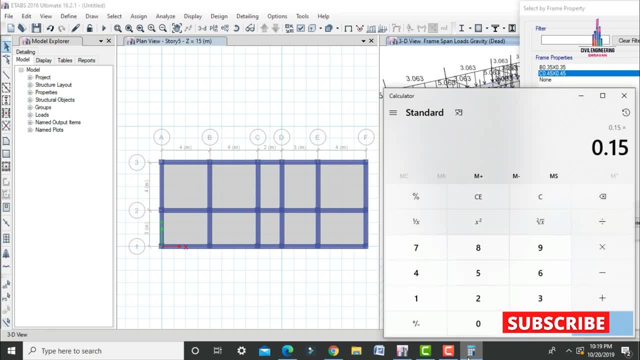 load. also, we can calculate the respected intensity with the help of the thickness intensity, with the help of the thickness intensity, with the help of the thickness 0.15 multiplied by 25, so it will give the 0.15 multiplied by 25, so it will give the. 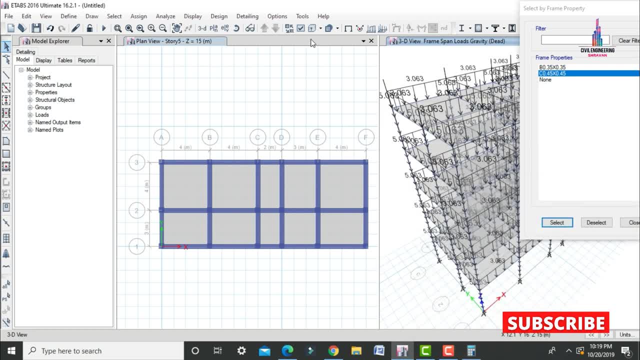 0.15 multiplied by 25, so it will give the intensity of 3.75. intensity of 3.75. intensity of 3.75. so select. go to select option. so select, so select. go to select option. so select, so select. go to select option. so select by properties. select by slab sections. 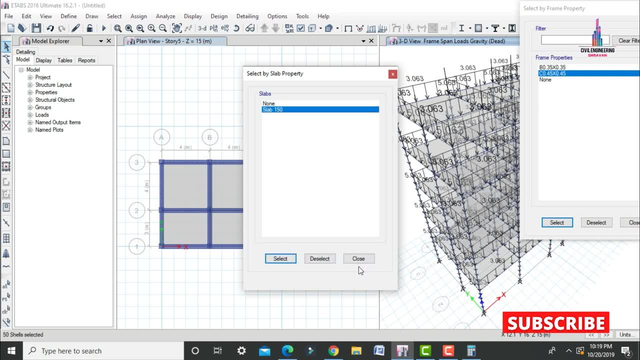 by properties: select by slab sections. by properties: select by slab sections. select s150 slab- select here so click on select s150 slab. select here, so click on select s150 slab. select here so click on select option here. click on close option. select option here. click on close option. 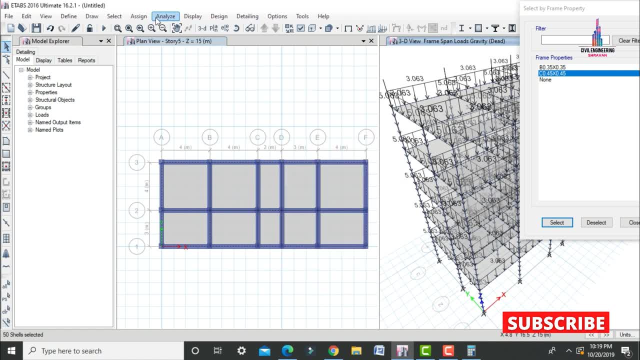 select option here. click on close option here, so it will select all your here. so it will select all your here. so it will select all your respected slab sections here. go to assign respected slab sections here. go to assign respected slab sections here. go to assign shell area loads uniform in this we need. 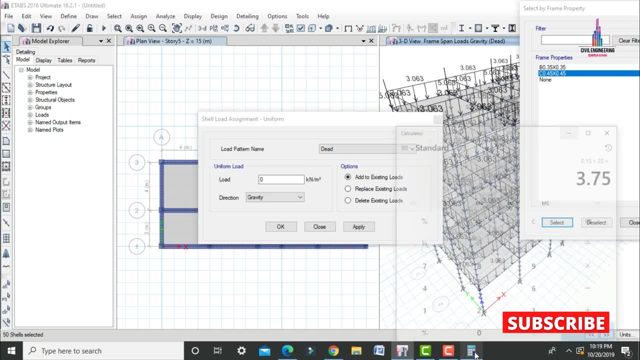 shell area loads uniform. in this we need shell area loads uniform. in this, we need to click on add to existing load, which is to click on add to existing load, which is to click on add to existing load, which is having the intensity of 3.75 load, so 3.75. 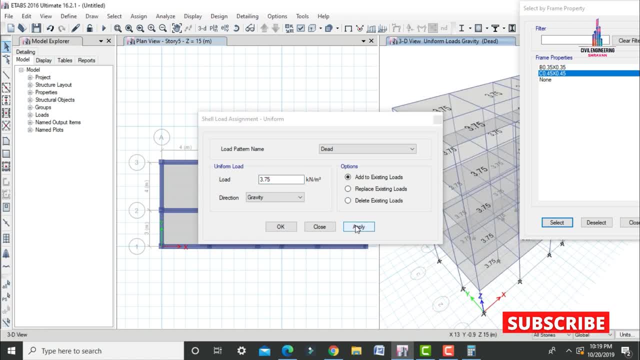 having the intensity of 3.75 load- so 3.75. having the intensity of 3.75 load- so 3.75. is the intensity of the load click on. is the intensity of the load click on? is the intensity of the load click on apply? so it will apply your respected 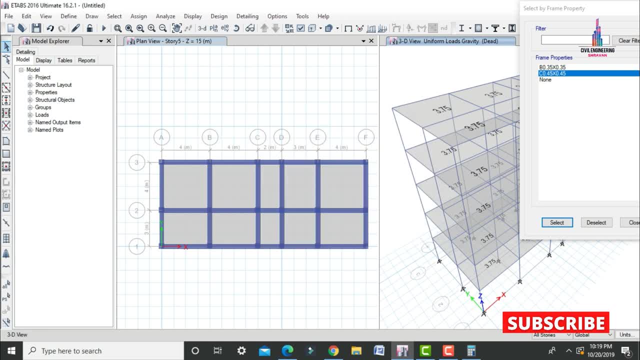 apply, so it will apply your respected. apply, so it will apply your respected: 3.75 for the slab members, only 3.75 for the slab members, only 3.75 for the slab members only. okay, so, after applying the slab dead. okay, so, after applying the slab dead. 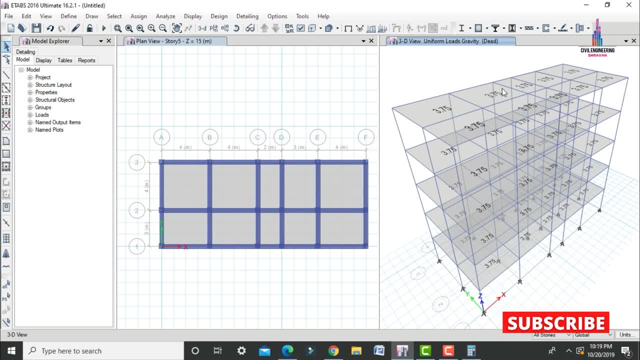 okay, so after applying the slab dead loading condition, to apply the live loading condition, to apply the live loading condition, to apply the live load for this building. so for that, we load for this building. so for that, we load for this building. so for that we have different options are there which? 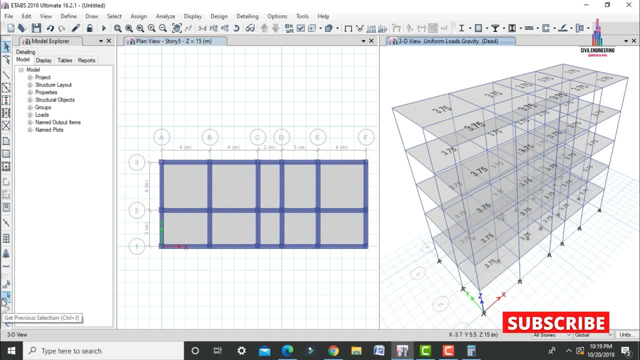 have different options are there, which have different options are there, which is related to the selection of all is related to the selection of all is related to the selection of all properties and previous section properties and previous section properties and previous section properties, clear property. so, if you want, 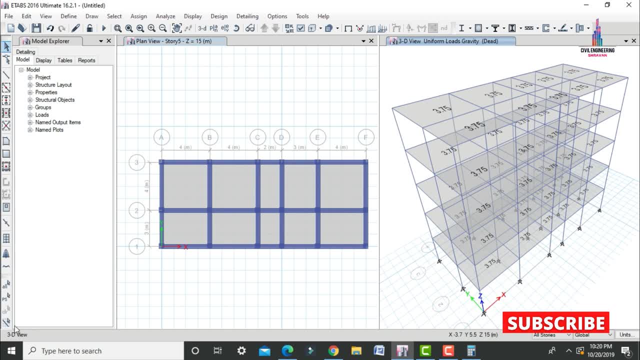 properties and previous section properties: clear property. so if you want properties and previous section properties, clear property. so if you want to clear the selected object, you to clear the selected object, you to clear the selected object. you can click on the clear if you wanted to, can click on the clear if you wanted to. 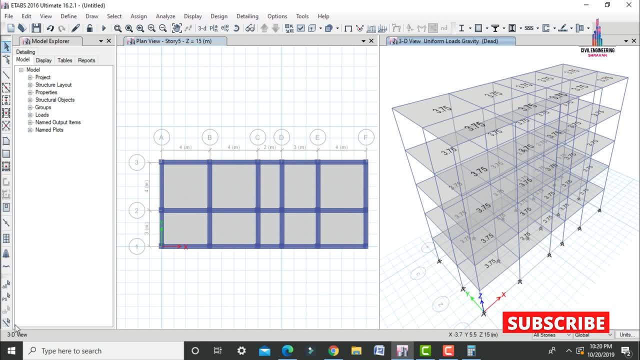 can click on the clear. if you wanted to select the previous objects. you can select the previous objects. you can select the previous objects. you can select the uh previous section option ps. select the uh previous section option ps. select the uh previous section option ps. and if you want to select all the, 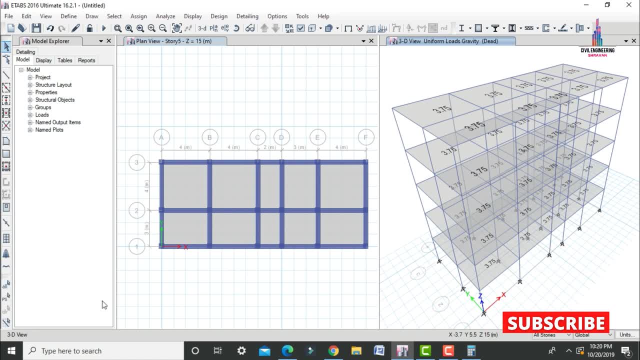 and if you want to select all the and if you want to select all the building structure, you can select all building structure. you can select all building structure. you can select all. okay. so here i am selecting the previous. okay, so here i am selecting the previous. okay, so here i am selecting the previous section, ps here, so it will select all. 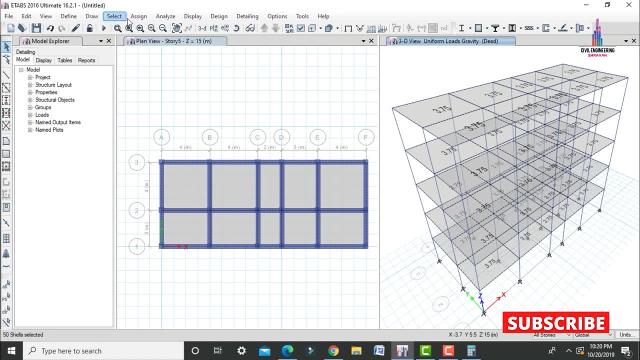 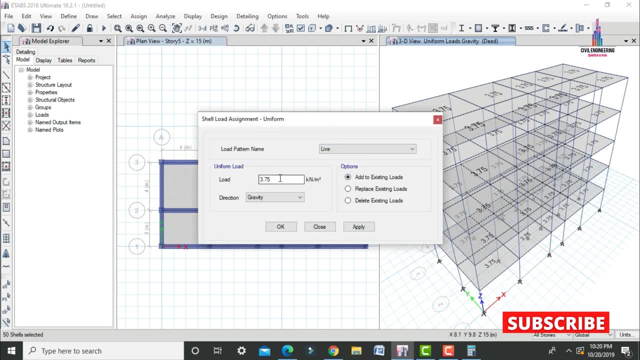 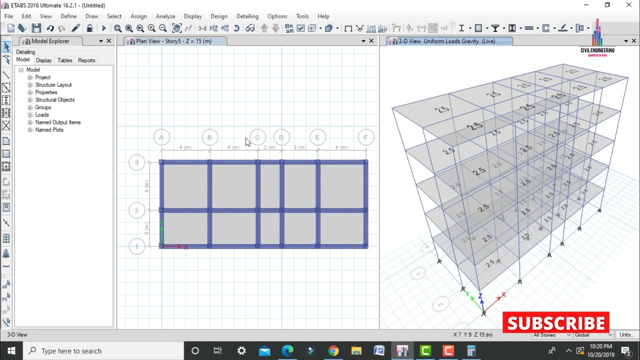 section ps here, so it will select all section ps here, so it will select all okay. so after that we have to apply the okay. so after that we have to apply the okay. so after that we have to apply the seismic loading condition which is in x. seismic loading condition which is in x. 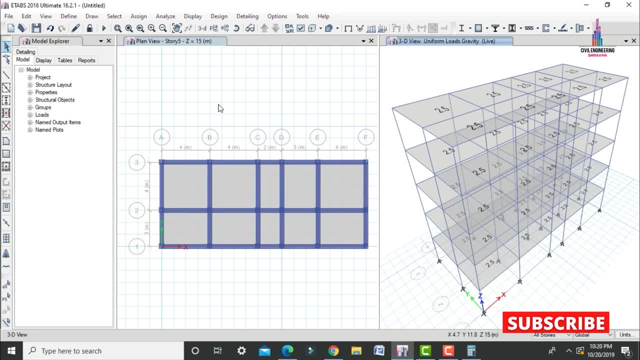 seismic loading condition which is in x direction as well as y direction direction, as well as y direction direction as well as y direction. so for that initially we need to select. so for that initially we need to select. so for that initially we need to select all the structure by using control a. 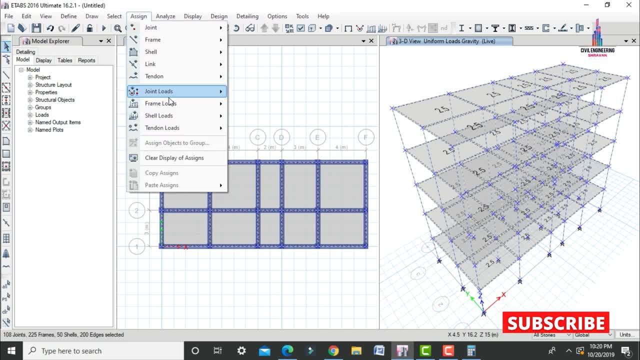 all the structure by using control a all the structure by using control a option. so go to click on assign option option. so go to click on assign option option. so go to click on assign option. shell area loads: we have to select. shell area loads: we have to select. 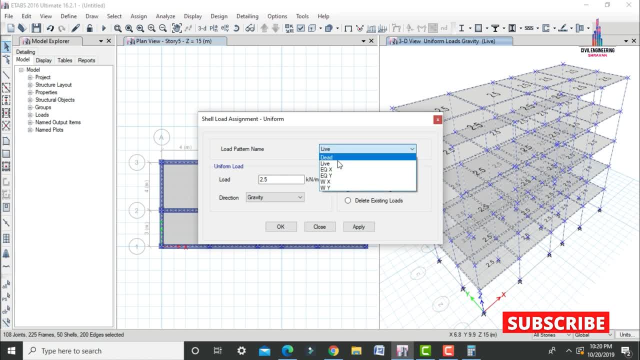 shell area loads. we have to select uniform load now. we have to select the uniform load now. we have to select the uniform load now. we have to select the load pattern as per the earthquake load pattern. as per the earthquake load pattern as per the earthquake load in x direction condition. so here: 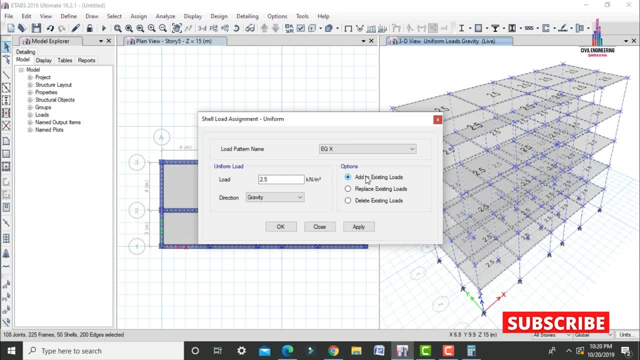 load in x direction condition. so here load in x direction condition. so here we have to add the new load cases which we have to add, the new load cases which we have to add, the new load cases which is related to the add to existing one is related to the add to existing one. 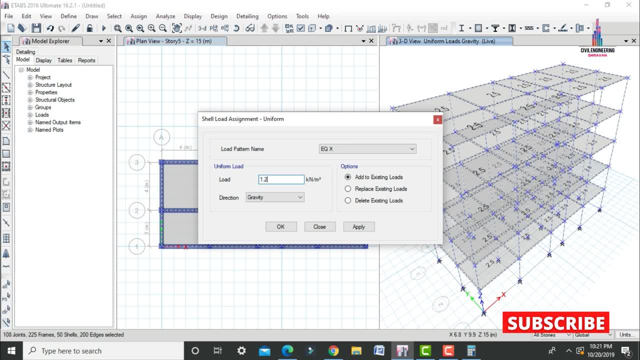 is related to the add to existing one. now, here we have to enter the load. now, here we have to enter the load. now, here we have to enter the load intensity which is related to the 50 intensity, which is related to the 50 intensity which is related to the 50 percentage of the live loading condition. 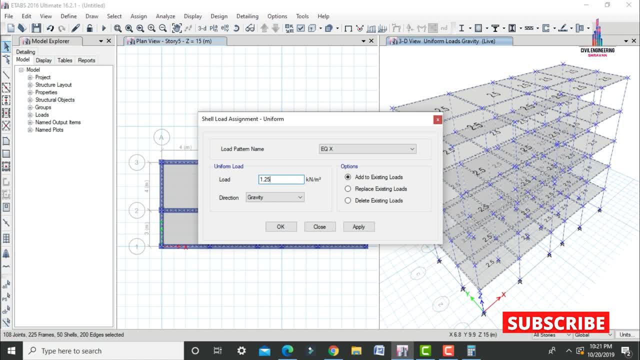 percentage of the live loading condition. percentage of the live loading condition. so here i was considered the live loading, so here i was considered the live loading, so here i was considered. the live loading condition for the building is 2.5. condition for the building is 2.5. 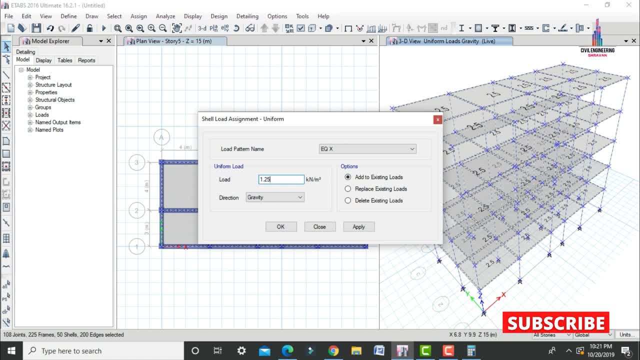 condition for the building is 2.5. we need to take 2.5 divided by 2, which we need to take 2.5 divided by 2, which we need to take 2.5 divided by 2, which is equals to 1.25. 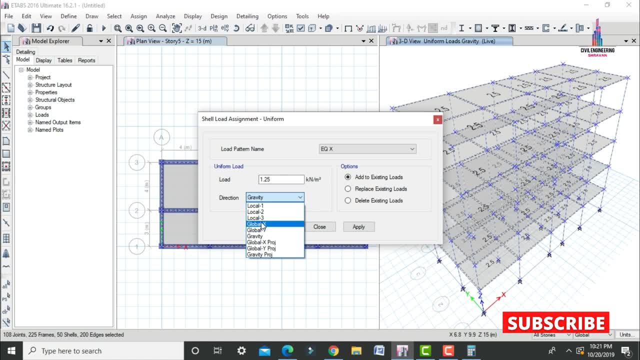 is equals to 1.25 is equals to 1.25, which is act in global x direction only which is act in global x direction, only which is act in global x direction only. please remember this point, click on add. please remember this point, click on add. 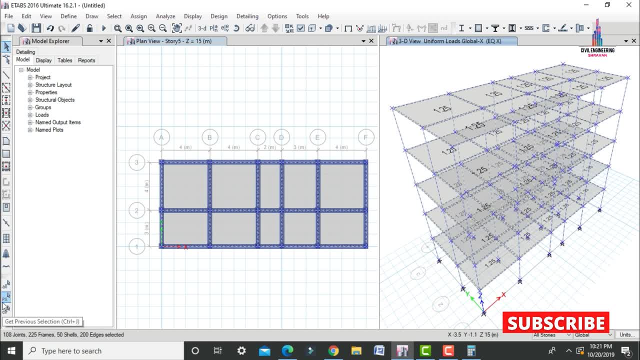 please remember this point. click on add close. in the same way, we have to select close. in the same way, we have to select close. in the same way, we have to select previous section, which is nothing but the previous section, which is nothing but the previous section, which is nothing but the selection of all building. 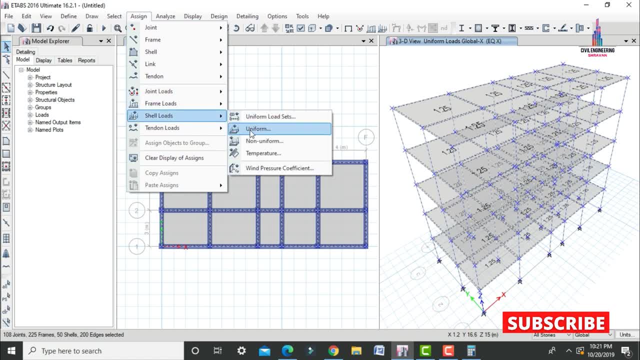 selection of all building. selection of all building again. go to assign shell area load uniform again. go to assign shell area load uniform again. go to assign shell area load uniform load again. we have to select the load again. we have to select the load again. we have to select the ethnic load in y direction. condition add: 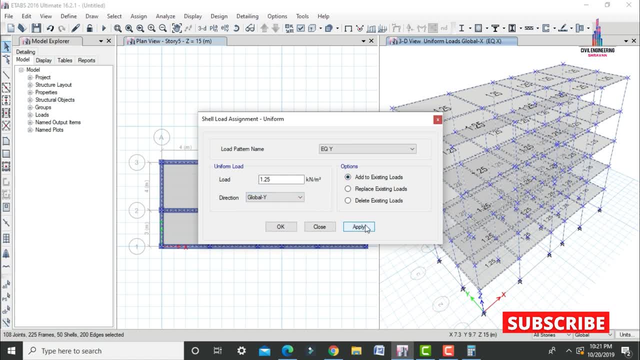 ethnic load in y direction condition: add: ethnic load in y direction condition: add to existing load. with the direction as to existing load. with the direction as to existing load, with the direction as global y click on apply. click on ok. global y click on apply. click on ok. 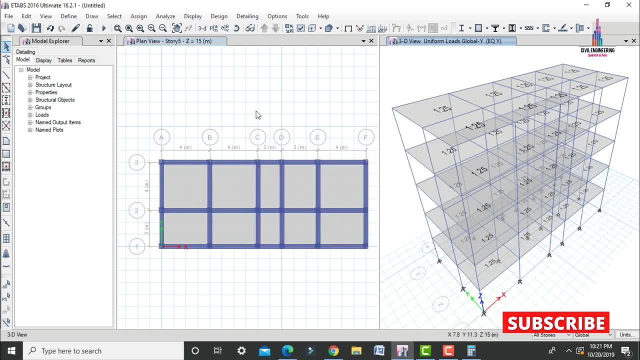 global y. click on apply, click on ok option. so after that we have to apply option. so after that we have to apply option. so after that we have to apply the wind load for this respective, the wind load for this respective, the wind load for this respective structure. so initially i am selecting. 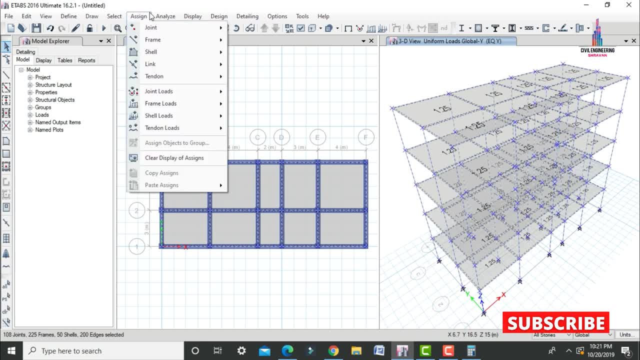 structure. so initially i am selecting structure. so initially i am selecting all the building. so click on assign all the building. so click on assign option. so click on select shell area option. so click on select shell area option. so click on select shell area load. in this it will be consisting of: 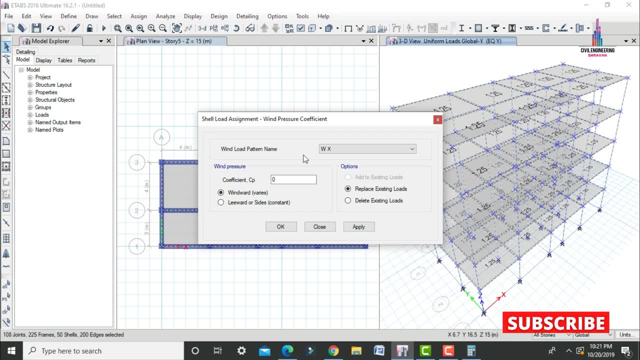 load. in this it will be consisting of load. in this, it will be consisting of wind pressure coefficient here. select wind pressure coefficient here. select wind pressure coefficient here. select this option. and now we have to enter this option. and now we have to enter this option. and now we have to enter the wind pressure coefficient 0.86. 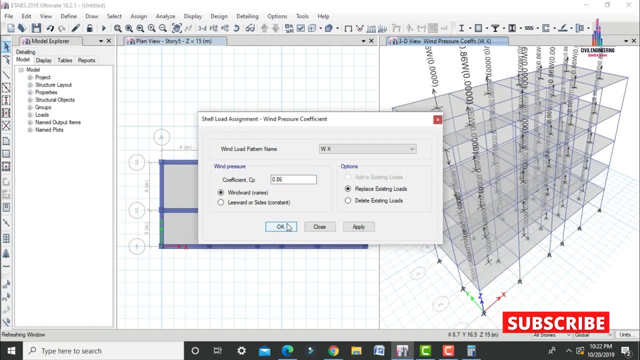 the wind pressure coefficient 0.86. the wind pressure coefficient 0.86. so click on apply option. so click on ok. so click on apply option. so click on ok. so click on apply option. so click on ok. so it will apply your respected wind. so it will apply your respected wind. 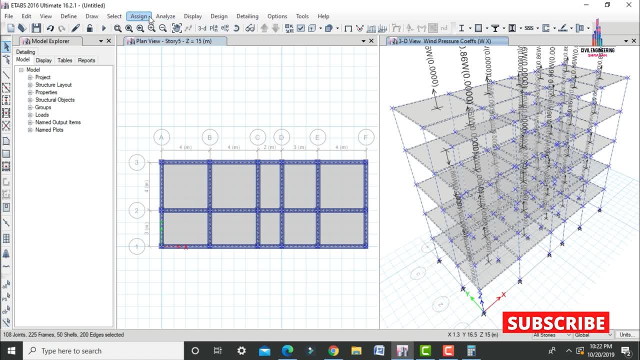 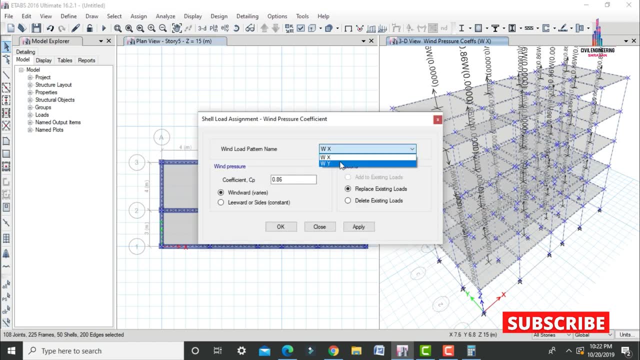 so it will apply your respected wind load again. i am selecting all the load again. i am selecting all the load again. i am selecting all the building structure. go to assign again i building structure. go to assign again i building structure. go to assign again i existing one. click on ok. so after adding, 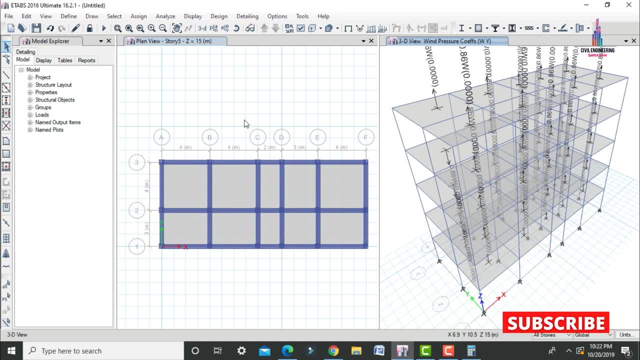 existing one. click on ok. so, after adding existing one, click on ok. so, after adding the load cases, we need to apply the load, the load cases. we need to apply the load, the load cases. we need to apply the load combinations for this, respective combinations for this respective. 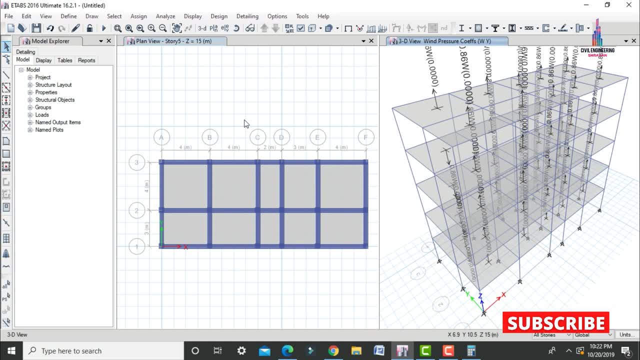 combinations for this respective structure. load combination is nothing. structure load combination is nothing. structure load combination is nothing but the combination of two or more load, but the combination of two or more load, but the combination of two or more load cases with the suitable value of the cases, with the suitable value of the. 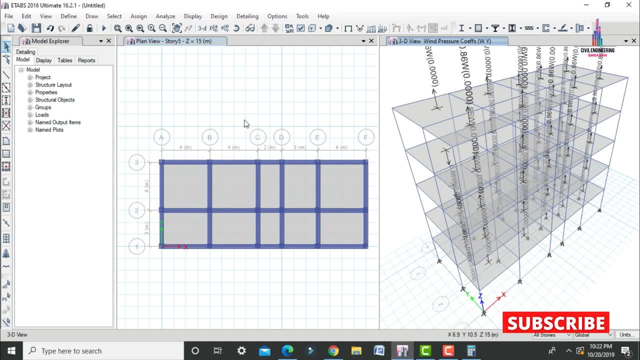 cases with the suitable value of the factor. okay, that suitable value of the factor. okay, that suitable value of the factor. okay, that suitable value of the factor will be available in is456 code. factor will be available in is456 code. factor will be available in is456 code. otherwise we have is875 part code that. 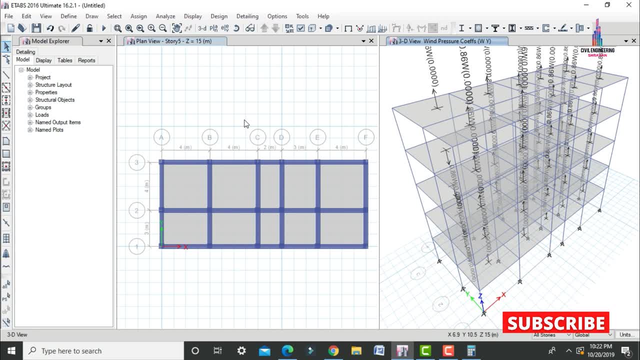 otherwise we have is875 part code that. otherwise we have is875 part code that. suitable properties of the factors will suitable properties of the factors, will suitable properties of the factors will be considered as per the tables. okay, so be considered as per the tables. okay, so be considered as per the tables. okay. so initially i am selecting define here. so 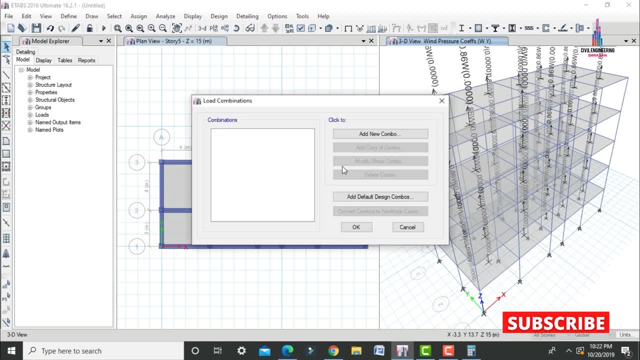 initially i am selecting define here. so initially i am selecting define here. so select load combination option here. so select load combination option here. so select load combination option here. so here i am selecting default design, here i am selecting default design here. i am selecting default design combinations here. so why? because i am 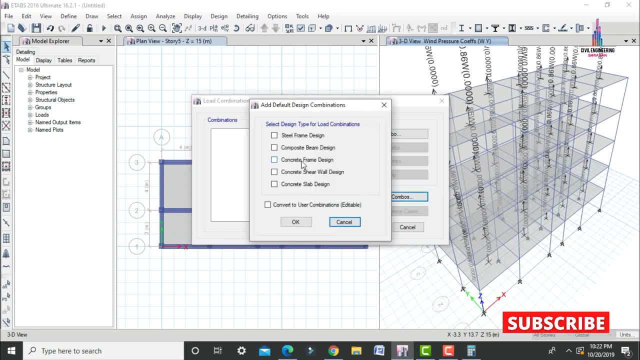 combinations here. so why? because i am combinations here? so why? because i am adding as per the concrete design section. adding as per the concrete design section. adding as per the concrete design section. so select the concrete frame design here. so select the concrete frame design here. so select the concrete frame design here. click on ok option so it will add your. 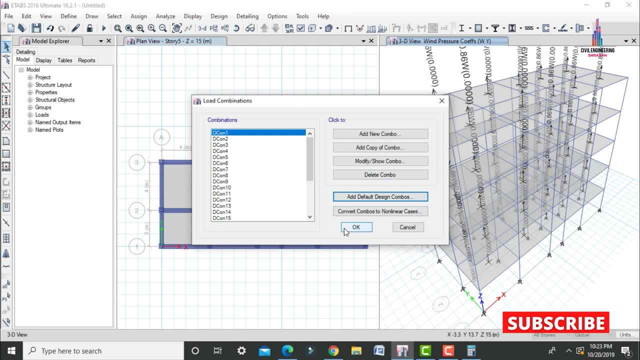 click on ok option, so it will add your. click on ok option so it will add your default design combinations as 26 options. default design combinations as 26 options. default design combinations as 26 options. click on ok option here, so it will add. click on ok option here, so it will add. 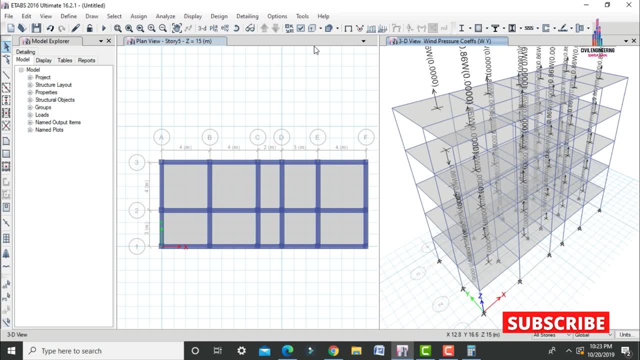 click on ok option here, so it will add your respected properties of load, your respected properties of load, your respected properties of load. combinations here, combinations here, combinations here. now, after assigning the load combinations, now, after assigning the load combinations, now, after assigning the load combinations, we need to assign the support set, the 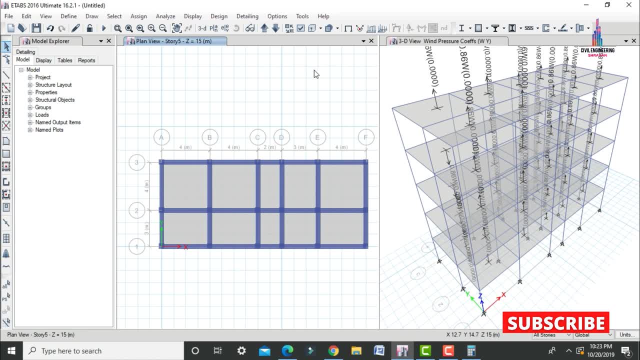 we need to assign the support set, the. we need to assign the support set, the base, base, base. okay, so for that initially. we need to okay. so for that initially. we need to okay, so for that initially. we need to select this plan view. select this plan view. 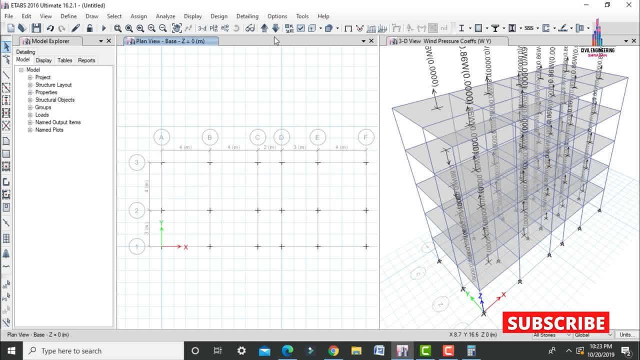 select this plan view again. go to the top view. okay, so it will again go to the top view. okay, so it will again go to the top view. okay, so it will move your respected object to the move, your respected object to the move, your respected object to the downward direction or upward direction. 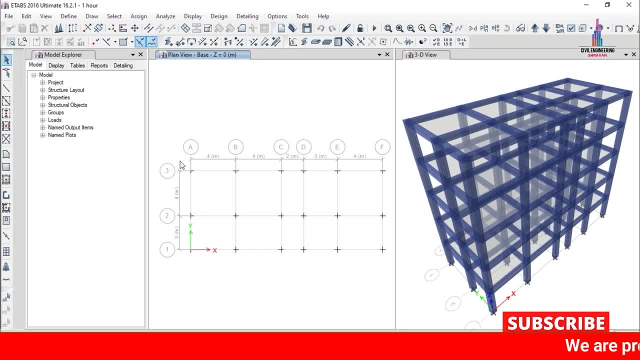 downward direction or upward direction? downward direction or upward direction, depending upon your considerations, depending upon your considerations, depending upon your considerations. so here i am selecting all the base at. so here i am selecting all the base at. so here i am selecting all the base at the ground story for this building. 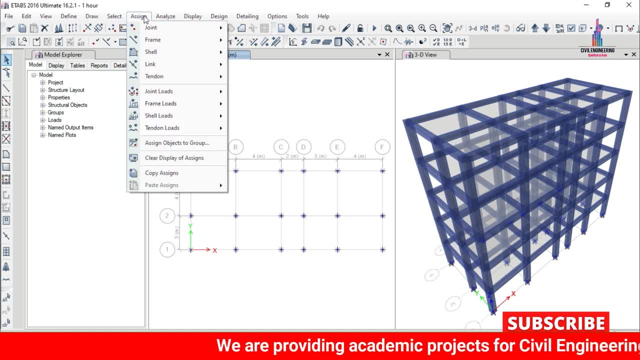 the ground story for this building. the ground story for this building. so after that, click on assign option. so after that, click on assign option. so after that, click on assign option. select join point on the top. so here we. select join point on the top. so here we. 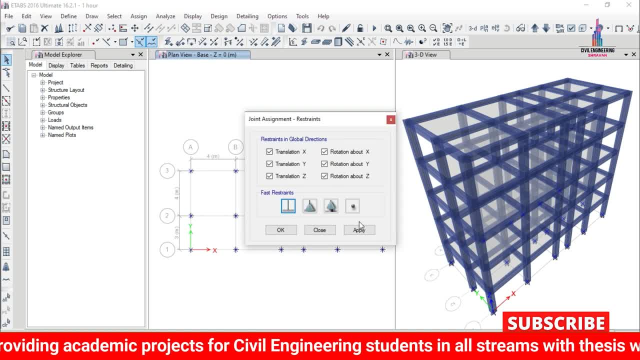 select join point on the top. so here we need to select the restraints option. need to select the restraints option. need to select the restraints option, so select your fixed supports. click on so select your fixed supports. click on so select your fixed supports. click on apply. click on okay, so it will apply. 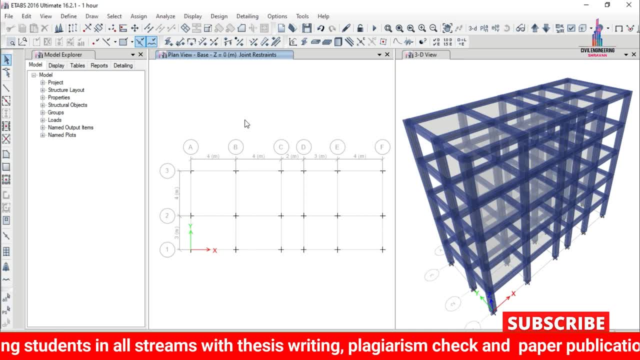 apply. click on okay, so it will apply. apply. click on okay, so it will apply. your respective fixed supports at the. your respective fixed supports at the. your respective fixed supports at the base. so after that we have to add the base. so after that, we have to add the. 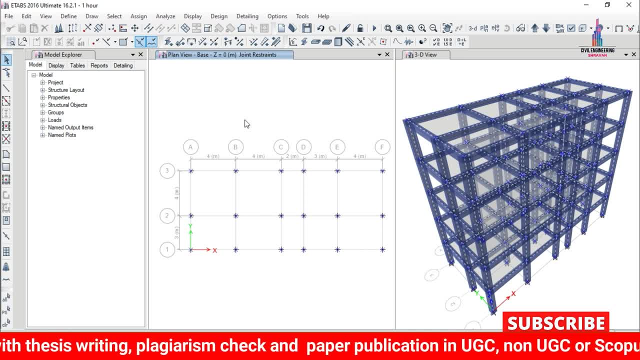 base. so after that we have to add the diaphragm. so initially we need to diaphragm. so initially we need to diaphragm. so initially we need to select all the building for that. so select all the building for that. so select all the building for that. so diaphragm is nothing but the center. 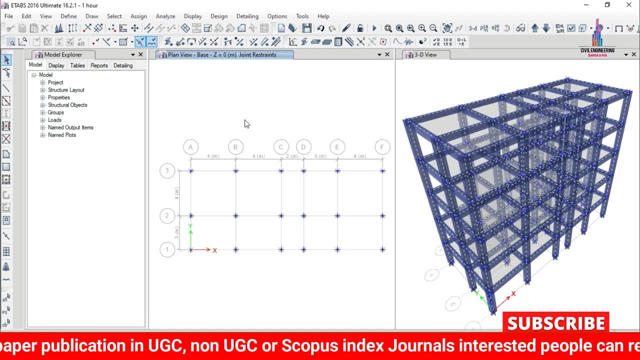 diaphragm is nothing but the center. diaphragm is nothing but the center point of the building as well as load point of the building. as well as load point of the building as well as load action rate. okay, so for different action rate. okay, so for different. 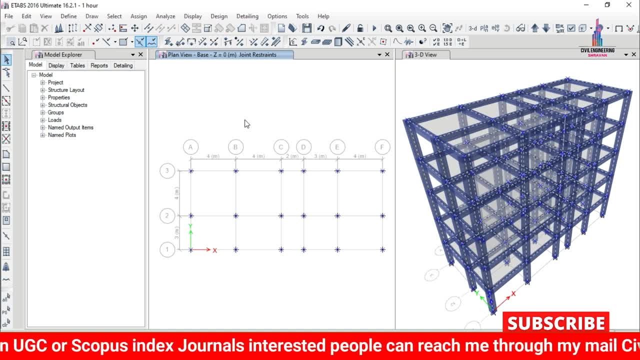 action rate. okay, so for different buildings. there is different types of buildings, there is different types of buildings, there is different types of diaphragm depending upon the geometry of diaphragm, depending upon the geometry of diaphragm, depending upon the geometry of the building. okay, so click on apply. 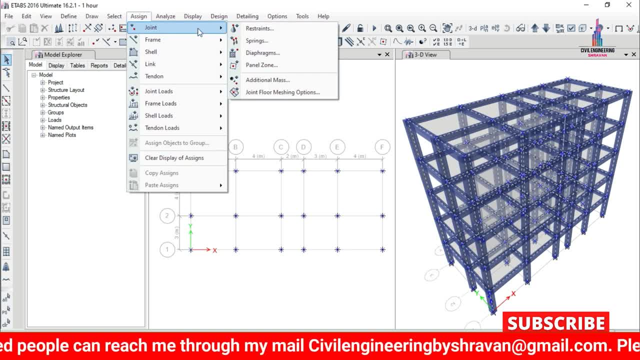 the building. okay, so click on apply the building. okay, so click on apply option. nothing but your assign option option: nothing but your assign option option: nothing but your assign option. here, so click on join. so here we have to. here, so click on join. so here we have to. 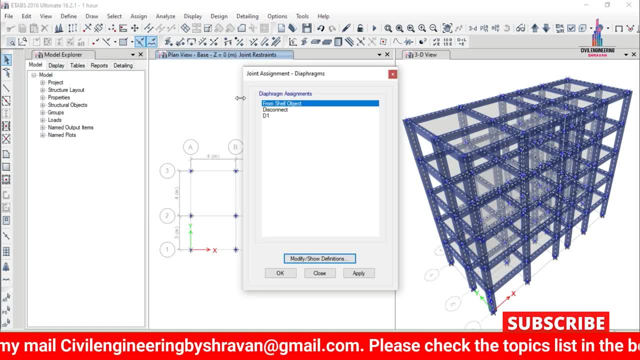 here, so click on join. so here we have to select the diaphragms here, so it will be select the diaphragms here, so it will be select the diaphragms here, so it will be consisting of default uh diaphragm like. consisting of default uh diaphragm like. 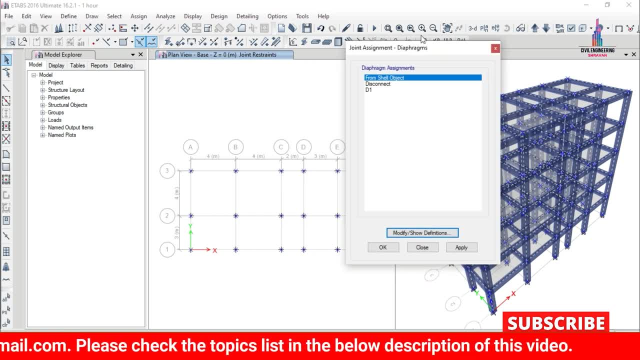 consisting of default uh, diaphragm, like from shell object disconnect and d1, so from shell object disconnect and d1, so from shell object disconnect and d1. so from this. just i am selecting the from this. just i am selecting the from this, just i am selecting the diaphragm section as d1. click on apply. 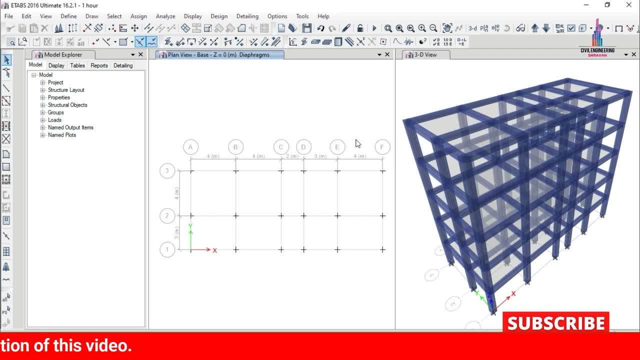 diaphragm section as d1: click on apply. diaphragm section as d1. click on apply option here. click on ok so it will apply option here. click on ok, so it will apply option here. click on ok so it will apply your diaphragm for this respective. 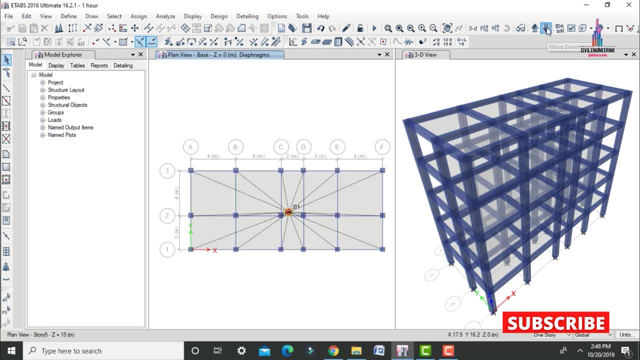 your diaphragm for this respective, your diaphragm for this respective structure, but it is not visible to you structure. but it is not visible to you structure. but it is not visible to you. respected 3d model. it is only visible to respected 3d model. it is only visible to: 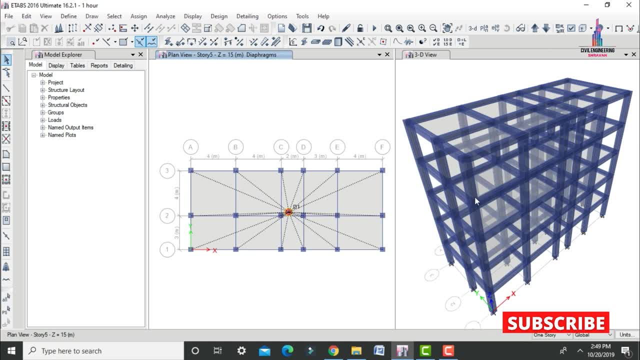 respected 3d model. it is only visible to the the the 2d model. if you want to visible that 2d model, if you want to visible that 2d model, if you want to visible that respected diaphragm for the 3d model. so 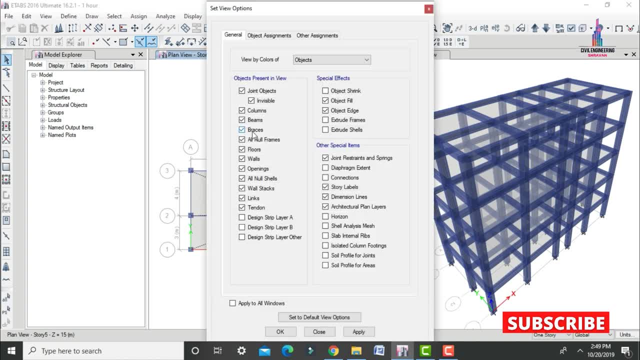 respected diaphragm for the 3d model. so, respected diaphragm for the 3d model. so we have to select the right mark on the. we have to select the right mark on the. we have to select the right mark on the right hand side section. so here we have. 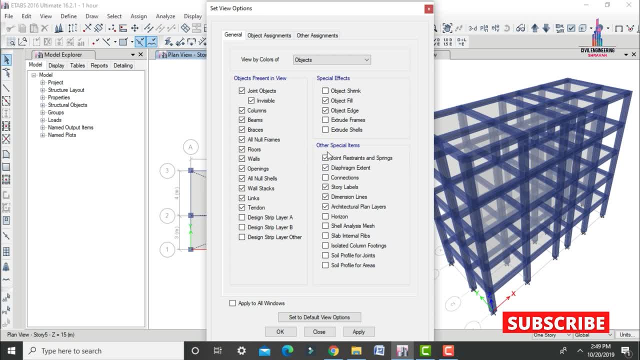 right hand side section. so here we have right hand side section. so here we have to select the diaphragm extend option in. to select the diaphragm extend option in to select the diaphragm extend option in other special items: click on apply to other special items. click on apply to. 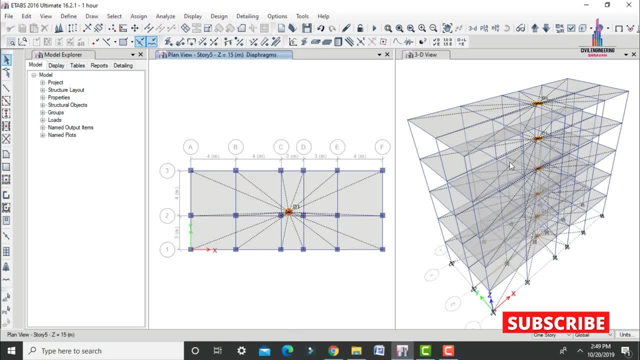 other special items. click on apply to all windows. click on apply. click on ok. all windows. click on apply. click on ok. all windows. click on apply. click on ok. so here you can see diaphragm was. so here you can see diaphragm was. so here you can see diaphragm was applied for this respective structure. 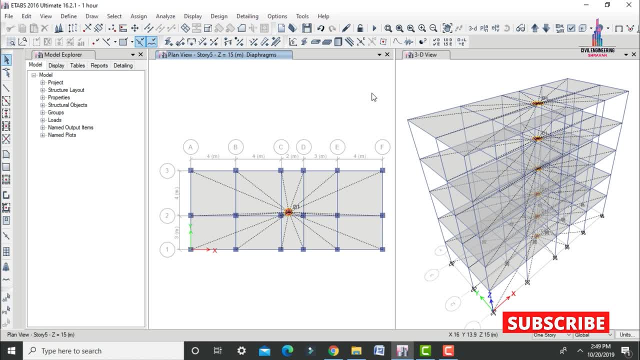 applied for this respective structure. applied for this respective structure: okay. so after assigning the diaphragm: we okay. so after assigning the diaphragm, we okay. so, after assigning the diaphragm, we need to analyze this respective need, to analyze this respective need to analyze this respective structure as per the seismic loading. 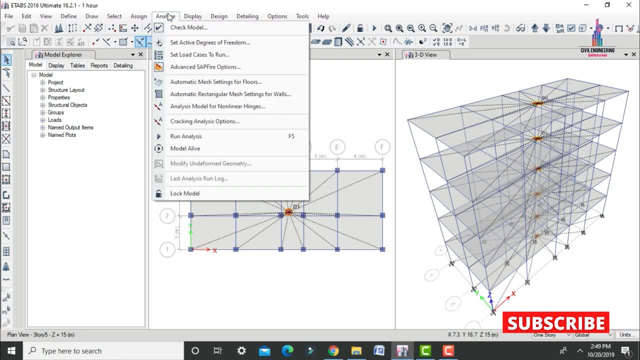 structure as per the seismic loading structure, as per the seismic loading point of view. so for that, initially we point of view. so for that initially we point of view. so for that, initially we need to click on analyze. so initially we need to click on analyze. so initially we 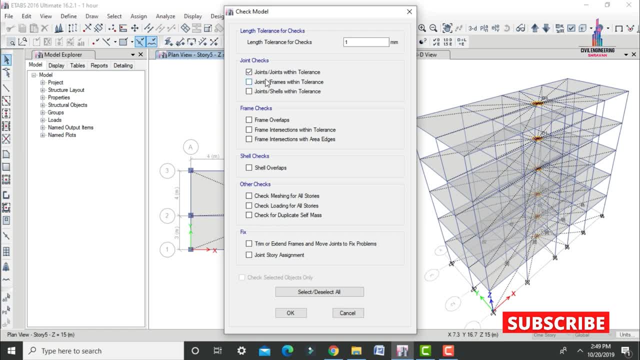 need to click on analyze. so initially we need to check the model for any errors, need to check the model for any errors, need to check the model for any errors. so now i am selecting the joint checks. so now i am selecting the joint checks. so now i am selecting the joint checks. it will be consisting of rain checks and 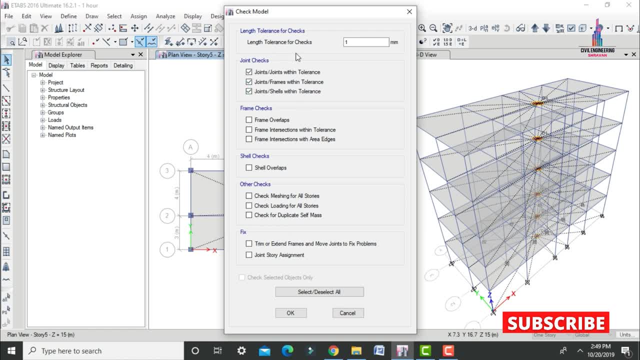 it will be consisting of rain checks. and it will be consisting of rain checks and shell checks, other checks- fixed one. so shell checks, other checks- fixed one. so shell checks, other checks- fixed one. so in this just, i am selecting only the. in this, just i am selecting only the. 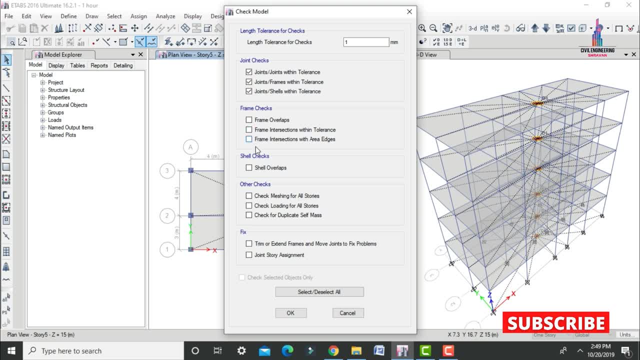 in this, just i am selecting only the joint six. if any errors, otherwise, you joint six. if any errors, otherwise you joint six. if any errors, otherwise you can select any one of this respected can select any one of this respected can select any one of this respected option for analysis. so click on ok option. 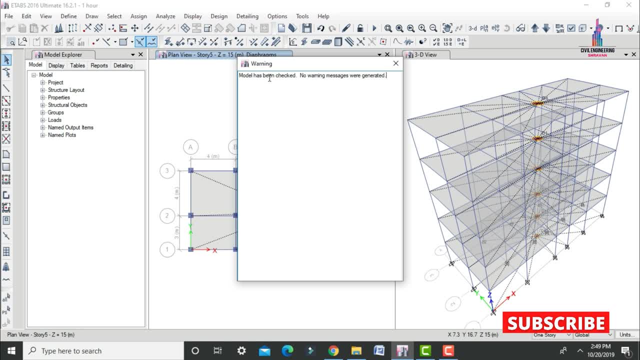 option for analysis, so click on ok option. option for analysis, so click on ok option. now we have to select the. now we have to select the. now we have to select the analyze option. so now it is showing the analyze option. so now it is showing the analyze option. so now it is showing: the model has been checked. no warning. 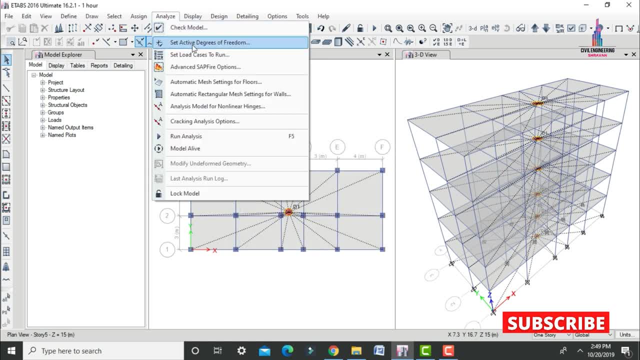 model has been checked. no warning model has been checked. no warning messages here. so after that go to messages here. so after that go to messages here. so after that go to analyze option. so here we have to select analyze option. so here we have to select analyze option. so here we have to select the set load cases to run. so initially the set load cases to run. so, initially, the set load cases to run, so initially, we need to select the load cases for we need to select the load cases for we need to select the load cases for that respected building. now i am. that respected building, now i am. 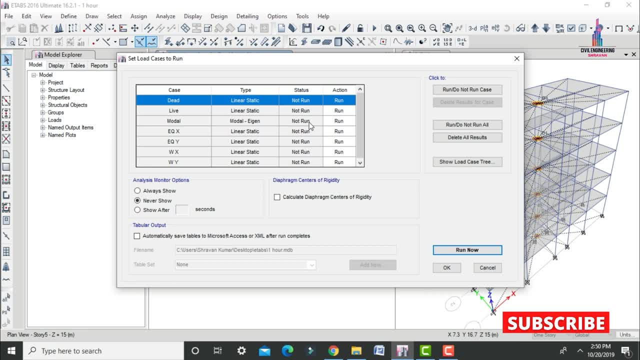 that respected building. now i am selecting all the load cases, which is selecting all the load cases, which is selecting all the load cases, which is related to the related to the related to the dead loading condition, live loading, dead loading condition, live loading, dead loading condition, live loading condition and. 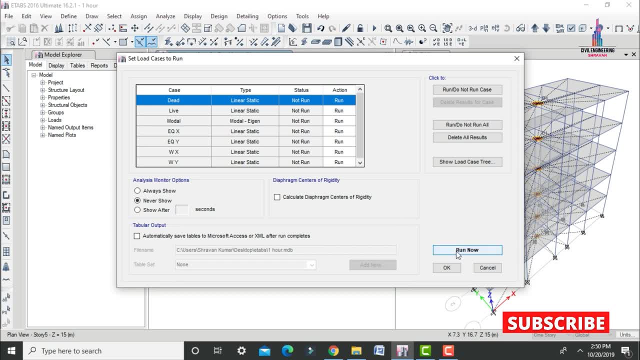 condition and condition and ethnic loading condition as well as ethnic loading condition, as well as ethnic loading condition as well as wind loading condition. so click on run wind loading condition. so click on run wind loading condition. so click on run now option, so it will run your respected 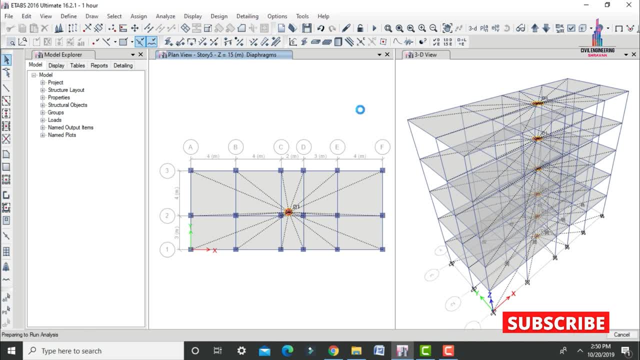 now option so it will run your respected now option, so it will run your respected model for analysis process. so after that model for analysis process, so after that model for analysis process, so after that, i will show you that the values which is, i will show you that the values which is. 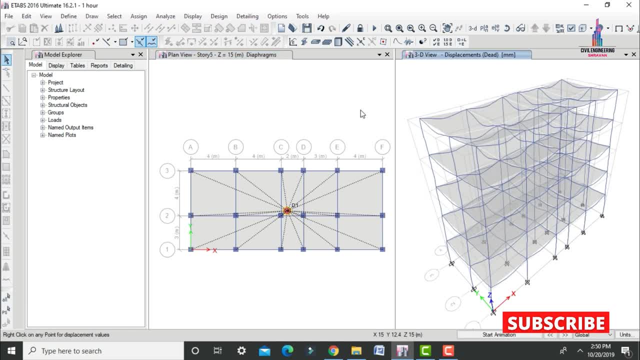 i will show you that the values which is related to the deflection shear bending, related to the deflection shear bending, related to the deflection shear bending and everything okay. so here my model was and everything okay. so here my model was and everything okay. so here my model was analyzed with zero errors. so here my 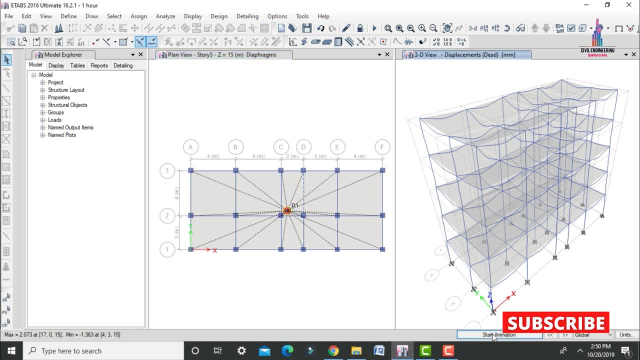 analyzed with zero errors. so here my: analyzed with zero errors, so here my model was analyzed, so initially we need. model was analyzed, so initially we need. model was analyzed, so initially we need to click on start animation option. due to click on start animation option. due to click on start animation option due to presence of the dead loading condition. 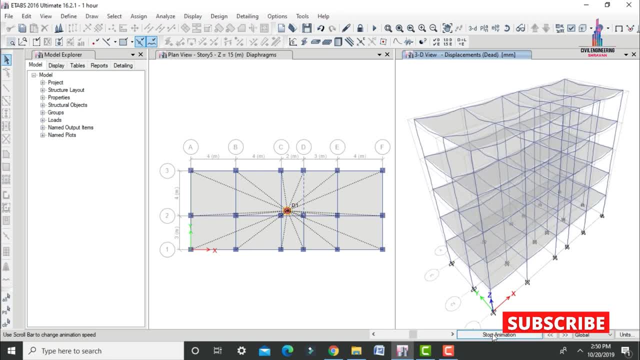 to presence of the dead loading condition. to presence of the dead loading condition. the building is deflecting like this. so the building is deflecting like this. so the building is deflecting like this. so we have to check the deflection for we have to check the deflection for 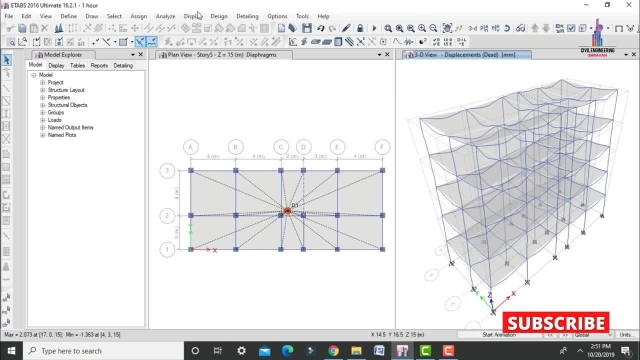 we have to check the deflection for different types of the load cases. so for different types of the load cases, so for different types of the load cases. so for that we have to go to display option, that we have to go to display option, that we have to go to display option here. so click on deform shape. here we 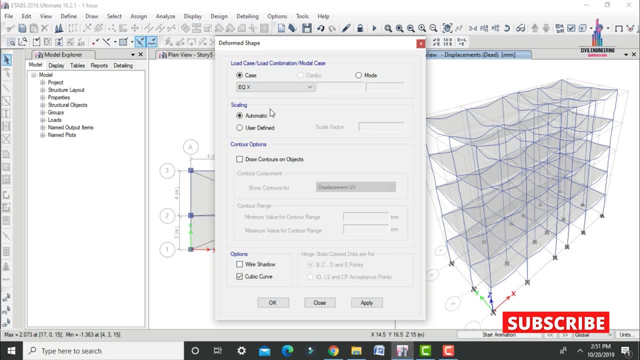 here. so click on deform shape. here we here, so click on deform shape. here we can select any one of the load case here can select any one of the load case. here can select any one of the load case here. so here i'm selecting example as at: 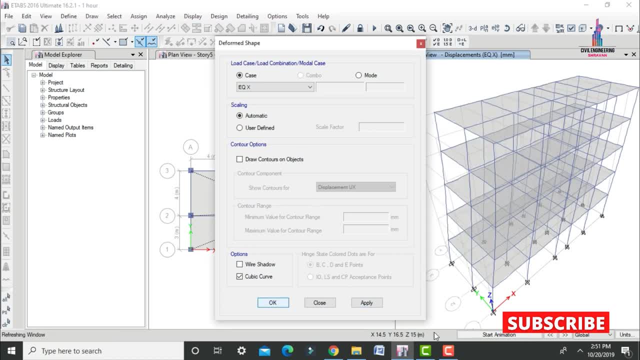 so here i'm selecting example as at: so here i'm selecting example as at: click load in x direction. click load in x direction. click load in x direction. click on apply. click on ok, so click on. click on apply. click on ok, so click on. click on apply. click on ok, so click on start animation option. 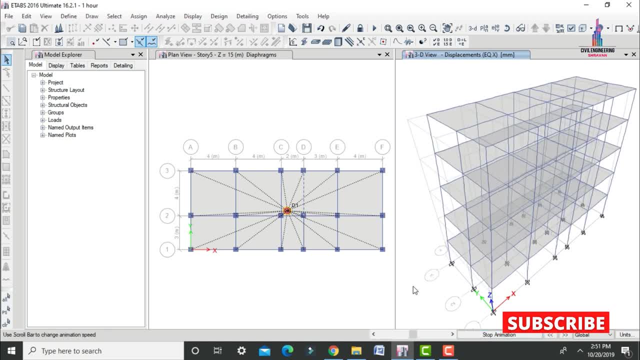 start animation option. start animation option. now we can see the building is now we can see the building is now we can see the building is deflecting in x direction condition due: deflecting in x direction condition due: deflecting in x direction condition due to presence of the. 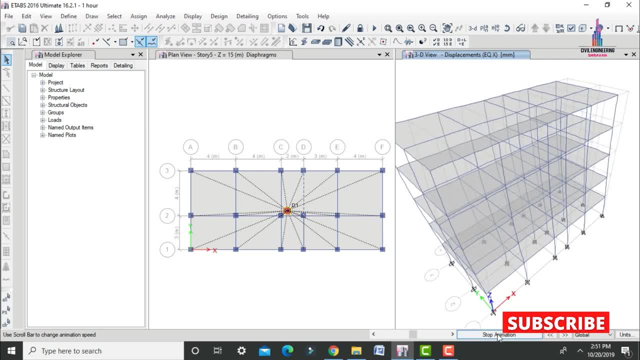 to presence of the, to presence of the ethnic load in x direction condition. so ethnic load in x direction condition, so ethnic load in x direction condition. so after that, click on stamp animation now. after that, click on stamp animation now. after that, click on stamp animation now we have to see the shear force diagram. 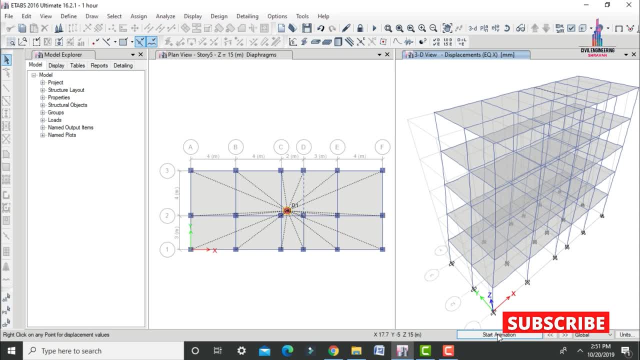 we have to see the shear force diagram. we have to see the shear force diagram, bending movement diagram, as well as your bending movement diagram. as well as your bending movement diagram as well as your torsion diagram for this building. torsion diagram for this building. torsion diagram for this building. so for that, go to click on display option. 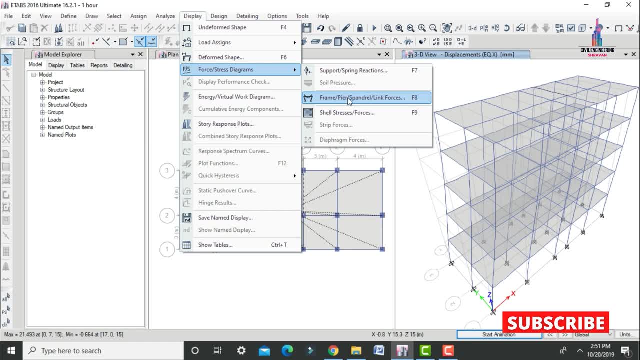 so for that, go to click on display option. so for that, go to click on display option. select forces stresses diagram. so here select forces stresses diagram. so here select forces stresses diagram. so here we have to select the, we have to select the, we have to select the frame. pierce pandrella forces. so in this: 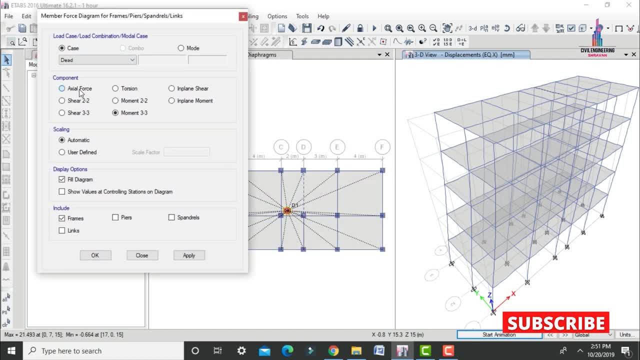 frame, pierce pandrella forces. so in this frame, pierce pandrella forces. so in this we need to select any one of the force. we need to select any one of the force. we need to select any one of the force. so here i'm selecting axial force click. 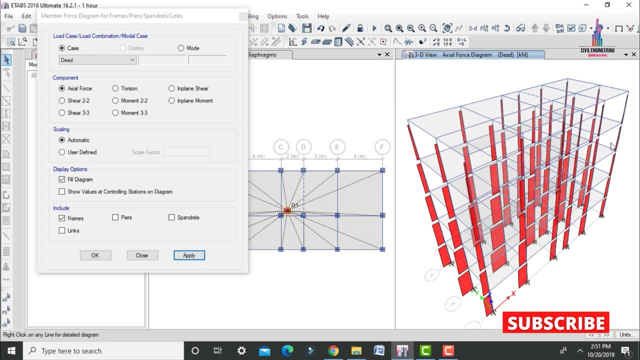 so here i'm selecting axial force click. so here i'm selecting axial force. click on apply. now we can see. this is the on apply. now we can see. this is the on apply. now we can see. this is the axial force diagram for this respective axial force diagram for this respective 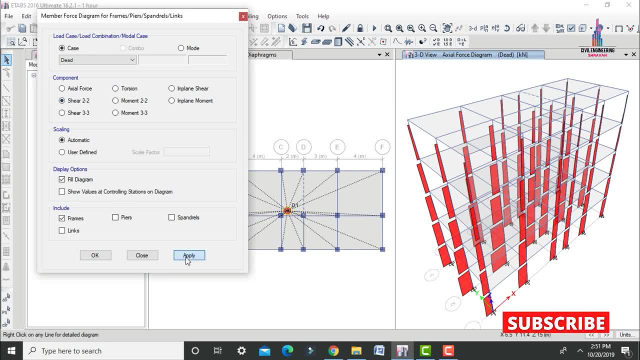 axial force diagram for this respective structure. again in the same way. we have structure, again in the same way. we have structure, again in the same way. we have to select the shear force x direction, to select the shear force x direction, to select the shear force x direction. so this is the shear force diagram for. 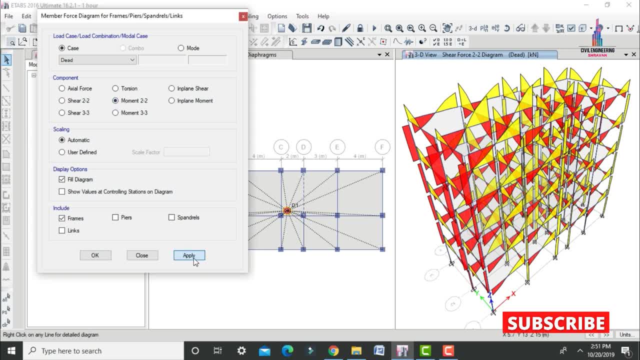 so this is the shear force diagram for. so this is the shear force diagram for this structure. again select the bending this structure. again select the bending this structure. again select the bending movement diagram. so click on apply. so movement diagram. so click on apply. so movement diagram. so click on apply. so this is the bending moment diagram for. 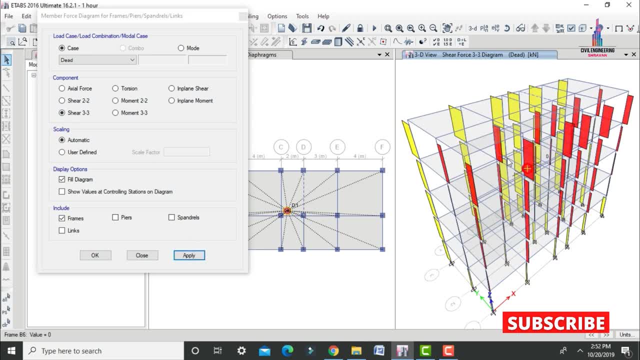 this is the bending moment diagram for. this is the bending moment diagram for this structure. select the shear 3: 3. click this structure. select the shear 3: 3. click this structure. select the shear 3- 3. click on apply. so this is the shear force. 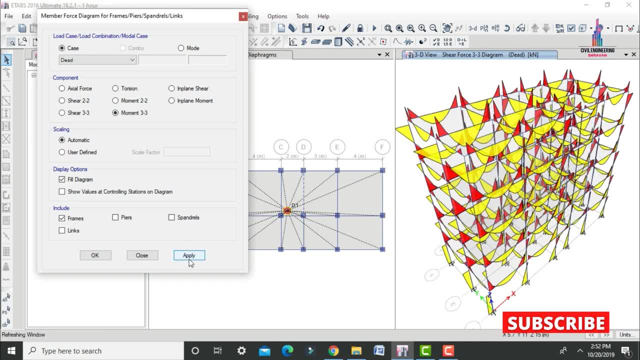 on apply. so this is the shear force on apply. so this is the shear force diagram in y direction condition bending diagram in y direction condition bending diagram in y direction. condition bending movement three. so click on apply. so this movement three. so click on apply. so this movement three. so click on apply. so this is the bending moment three, and again i. 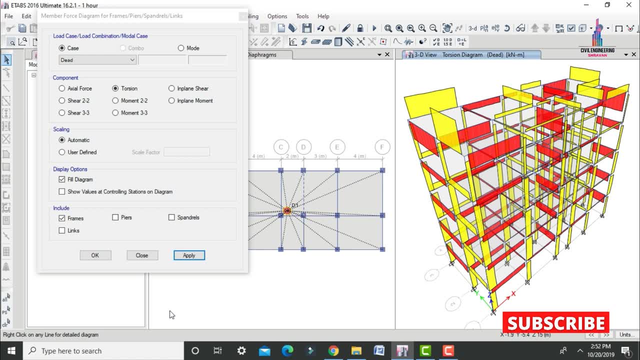 is the bending moment three, and again, i is the bending moment three. and again i am applying the torsion. click on apply. am applying the torsion. click on apply. am applying the torsion. click on apply option. so this is the building torsion option. so this is the building torsion. 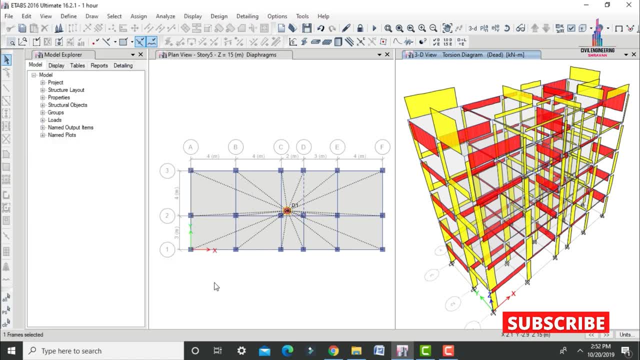 option. so this is the building torsion for this respective structure. so after for this respective structure. so after for this respective structure. so, after checking the diagrams which are related, checking the diagrams which are related, checking the diagrams which are related to the shear bending, as well as. 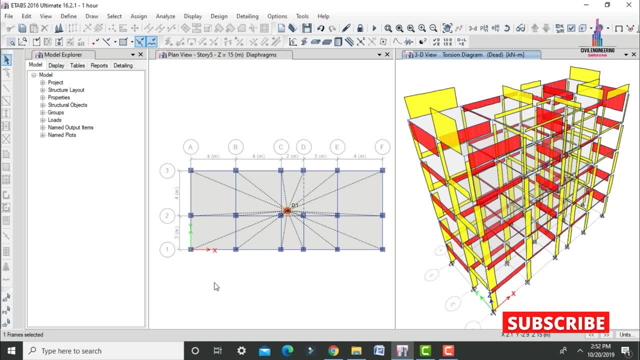 to the shear bending as well as to the shear bending as well as deflection values. we have to see the deflection values. we have to see the deflection values. we have to see the tables as well as results. okay, so for tables as well as results. okay, so for. 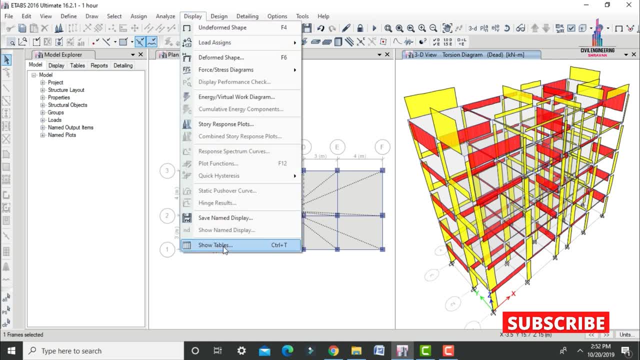 tables as well as results. okay, so for that we have to click on display option. that we have to click on display option. that we have to click on display option. so here we have to select the show. so here we have to select the show. so here we have to select the show tables option. in this we need to select. 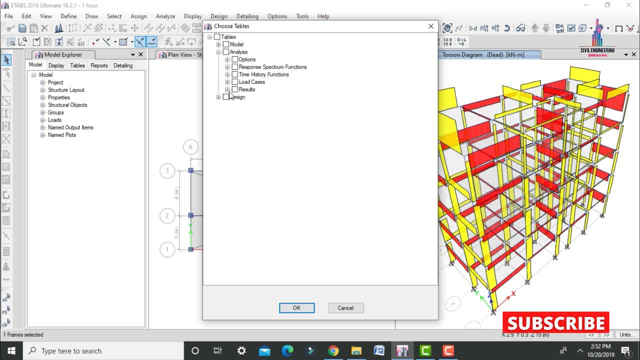 tables option. in this, we need to select tables option. in this, we need to select the analysis data results, which is the analysis data results, which is the analysis data results, which is related to your respected uh deflection, related to your respected uh deflection, related to your respected uh deflection value, which is nothing but displacement. 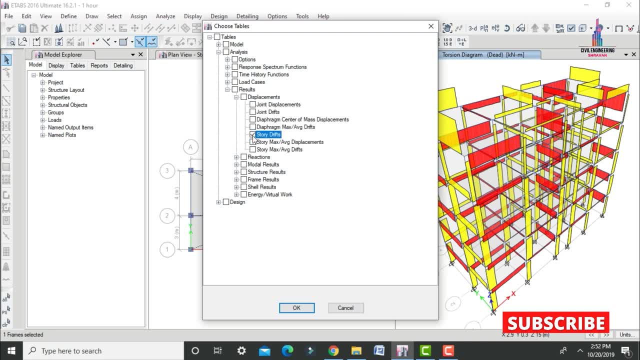 value which is nothing but displacement value, which is nothing but displacement values. so here i'm selecting story drift values. so here i'm selecting story drift values. so here i'm selecting story drift value. let us consider again: i'm value. let us consider again i'm value. let us consider again: i'm selecting reactions, base reaction again. 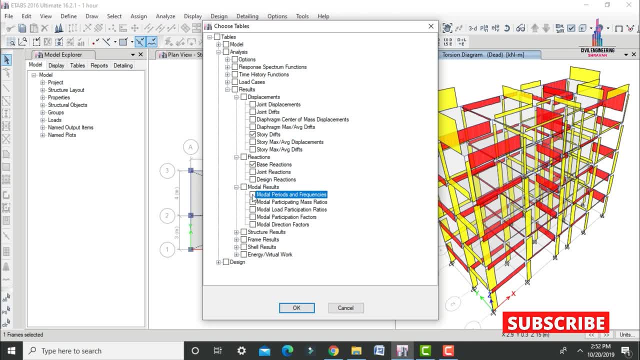 selecting reactions: base reaction- again selecting reactions- base reaction. again i'm selecting model results, which is i'm selecting model results, which is i'm selecting model results which is related to time period and frequency, related to time period and frequency, related to time period and frequency values. again in the same way, just i'm. 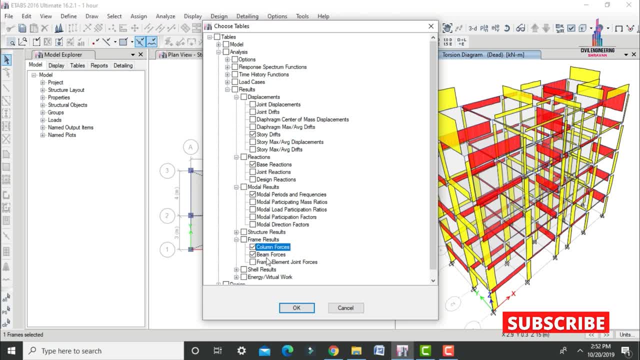 values again in the same way. just i'm values. again in the same way. just i'm selecting frame results for the columns. selecting frame results for the columns. selecting frame results for the columns and beams. so after that we have to click and beams. so after that we have to click. 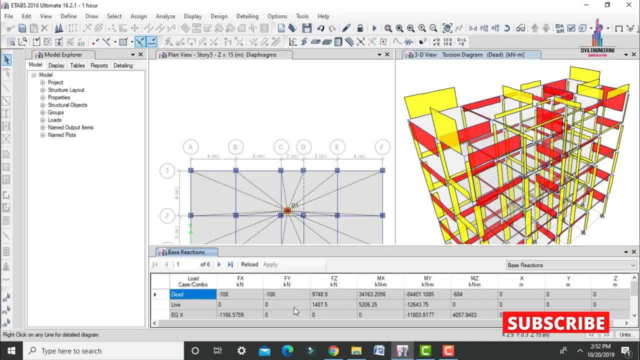 and beams. so after that we have to click on okay option, on okay option, on okay option, so it will load the output values which, so it will load the output values which, so it will load the output values. which is related to the deflection value base. is related to the deflection value base. 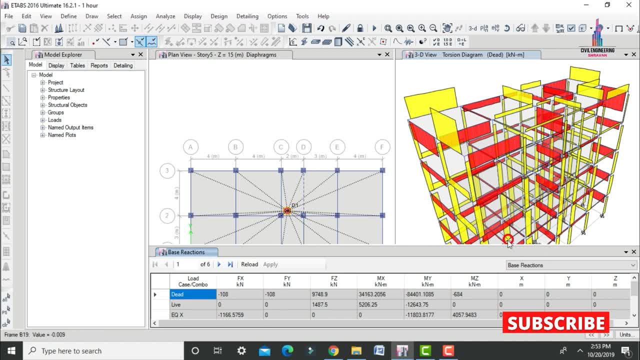 is related to the deflection value base reactions and everything on the tables- reactions and everything on the tables- reactions and everything on the tables here like this: okay, so you can check the here like this. okay, so you can check the here like this: okay, so you can check the results. which is related to this. 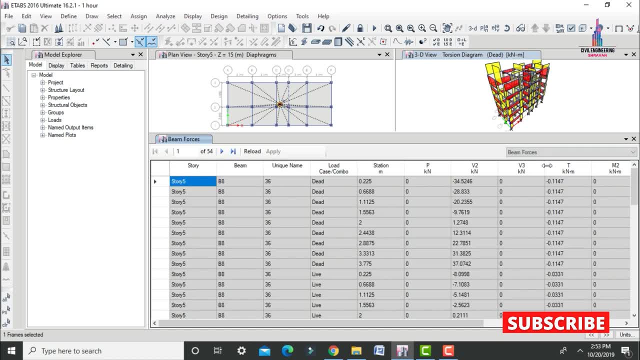 results which is related to this results which is related to this respected part. so here i'm selecting base respected part. so here i'm selecting base respected part. so here i'm selecting base reaction and beam forces. again i'm reaction and beam forces. again i'm reaction and beam forces. again i'm selecting one more section: column forces. 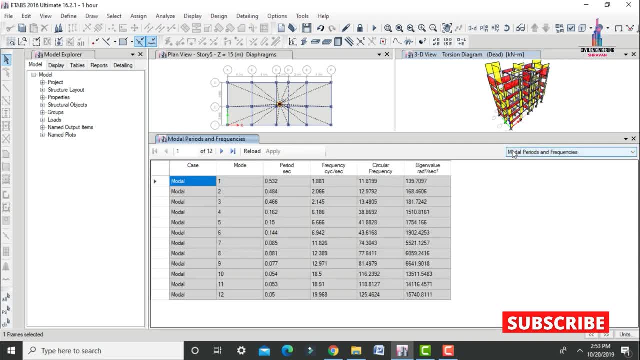 selecting one more section. column forces. selecting one more section. column forces- again, i'm selecting one more section. again i'm selecting one more section. again i'm selecting one more section. model time period and frequency values. model time period and frequency values. model time period and frequency values. ison values: again i'm selecting story. 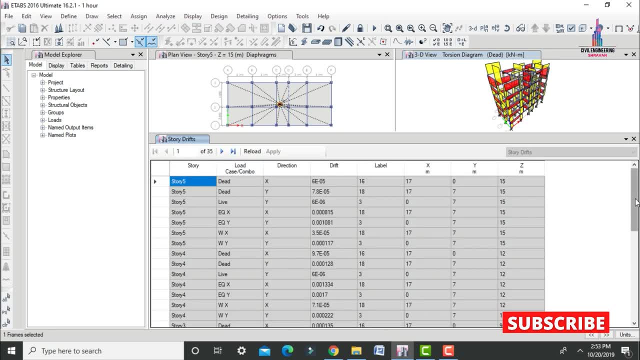 ison values. again i'm selecting story ison values. again i'm selecting story drift values. so these are the output drift values. so these are the output drift values. so these are the output values for this respected g, place 4. values for this respected g, place 4. 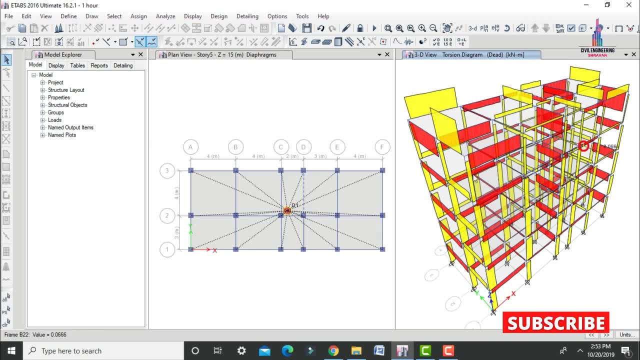 values for this respected g place 4 structure. so after analysis process structure. so after analysis process structure. so after analysis process completed, we need to design this completed, we need to design this completed. we need to design this respected structure of g plus 4. so this respected structure of g plus 4. so this: 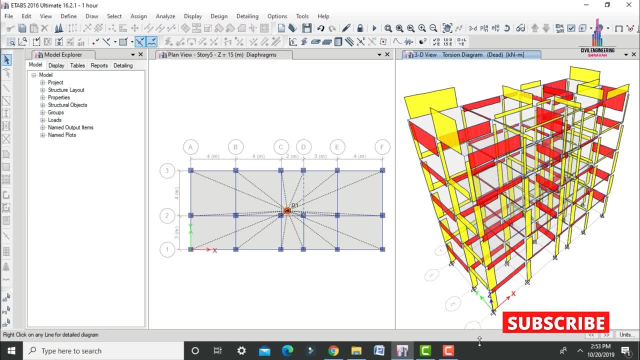 respected structure of g plus 4. so this is the important part of building design. is the important part of building design, is the important part of building design process in etamp software. okay, so, as per process in etamp software. okay, so, as per process in etamp software. okay, so, as per my considerations, i am designing this. 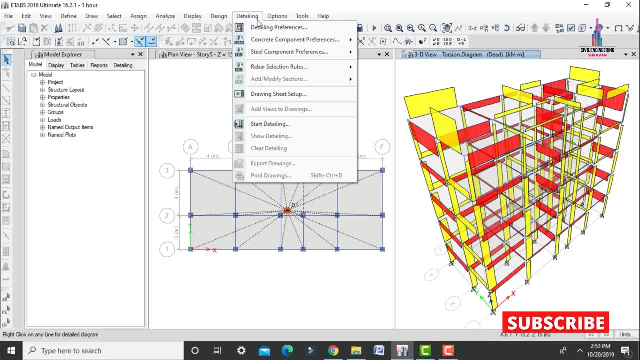 my considerations. i am designing this, my considerations, i am designing this: respected building as per is456 code. so respected building as per is456 code. so respected building as per is456 code. so for that, select your design option here. for that, select your design option here. for that, select your design option here. so in this, we need to select the. 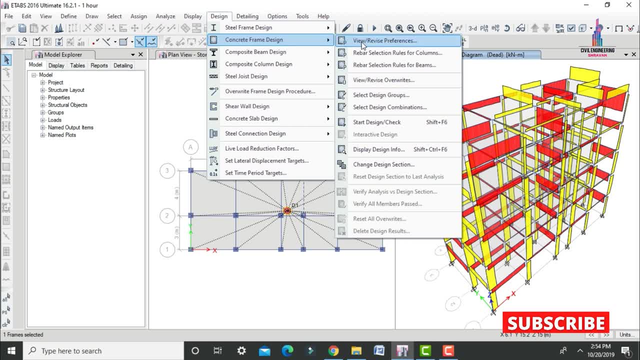 so in this, we need to select the. so in this, we need to select the concrete frame design. so here, initially, concrete frame design. so here, initially, concrete frame design. so here, initially, we need to select the view preferences. we need to select the view preferences, we need to select the view preferences option, so it will be consisting of your. 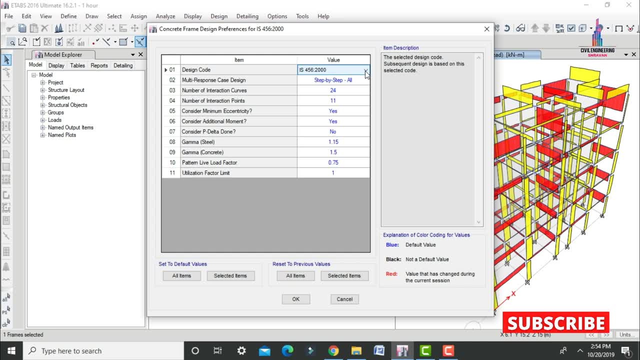 option. so it will be consisting of your option. so it will be consisting of your design code as per the indian standard design code. as per the indian standard design code. as per the indian standard system of 456. you can select any one of system of 456. you can select any one of: 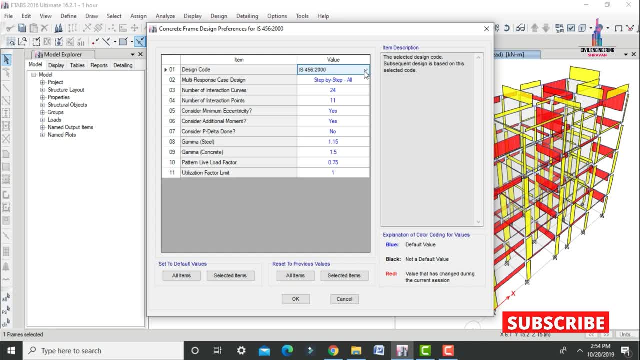 system of 456, you can select any one of the code. other code also, depending upon the code. other code also depending upon the code other code also depending upon your considerations. so, as per my your considerations, so as per my your considerations, so as per my assumption, just i am taking it as is456. 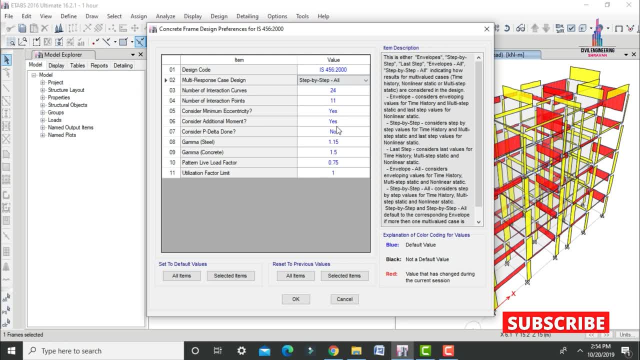 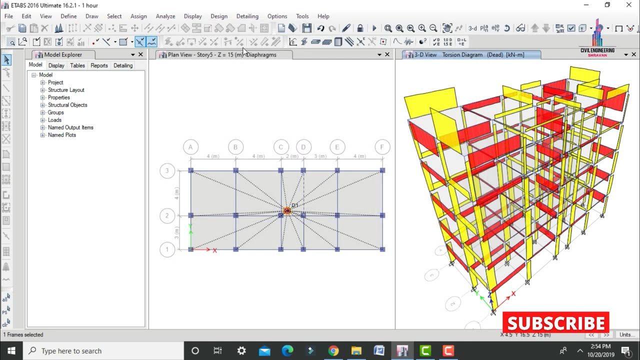 assumption: just i am taking it as is456 assumption, just i am taking it as is456 code. so again it will be consisting of code. so again it will be consisting of code. so again it will be consisting of it as same values. click on ok. so after: 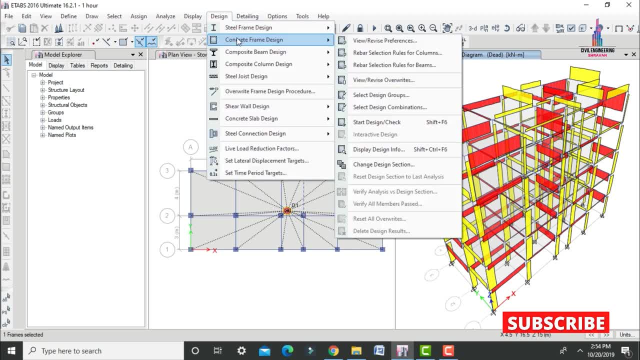 it as same values: click on ok. so after it as same values: click on ok. so after that we have to click on uh design. that we have to click on uh design. that we have to click on uh design option. here again we have to select the option. here again we have to select the. 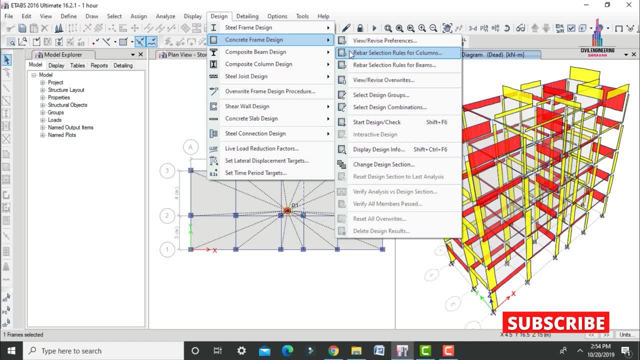 option. here again, we have to select the concrete frame design now. we need to concrete frame design now. we need to concrete frame design now we need to select the rebar section. rules for the. select the rebar section. rules for the. select the rebar section. rules for the column section. so select this, respected. 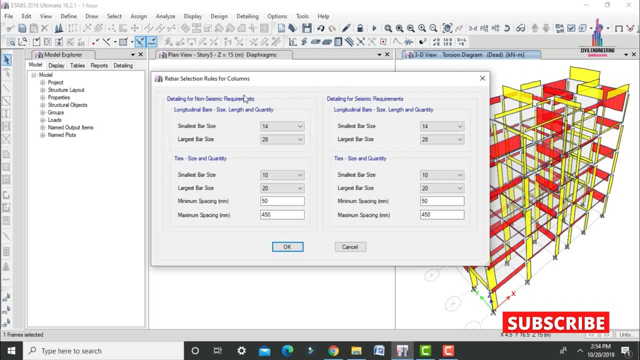 column section. so select this respected column section. so select this respected option. so for the column resection: it option. so for the column resection: it option. so for the column resection, it will be consisting of the detailing for: will be consisting of the detailing for. will be consisting of the detailing for: non-seismic requirement case and seismic. 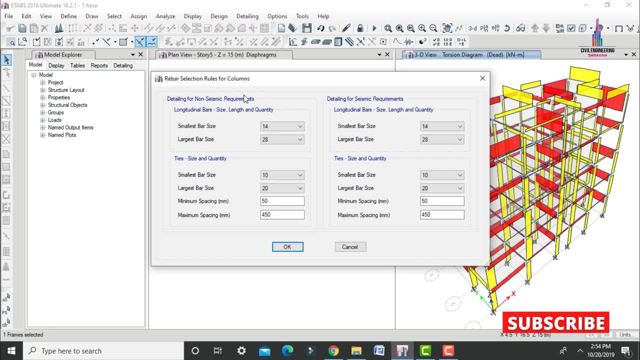 non-seismic requirement case and seismic, non-seismic requirement case and seismic requirement case. so if you are designing requirement case, so if you are designing requirement case, so if you are designing any one of the building which is related, any one of the building which is related, 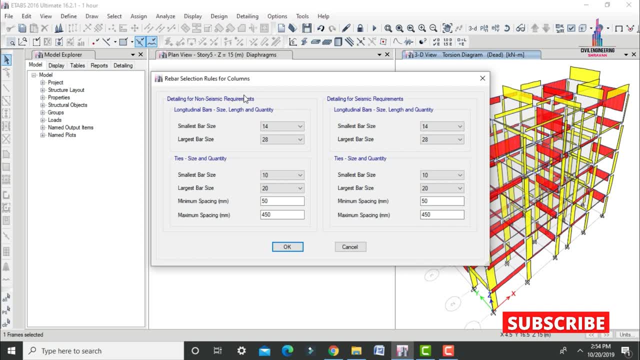 any one of the building which is related to the gravity loads only, which is to the gravity loads only, which is to the gravity loads only, which is nothing but your dead loading condition, nothing but your dead loading condition, nothing but your dead loading condition. live loading condition, floor loading. 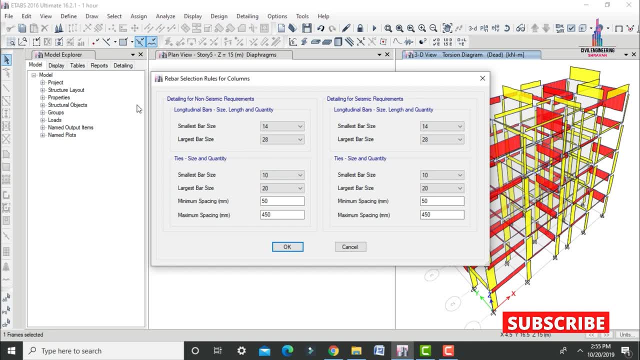 live loading condition floor loading- live loading condition floor loading condition, then you need to consider it condition. then you need to consider it condition, then you need to consider it as this respected detailing option for as this respected detailing option for as this respected detailing option for non-seismic requirements. 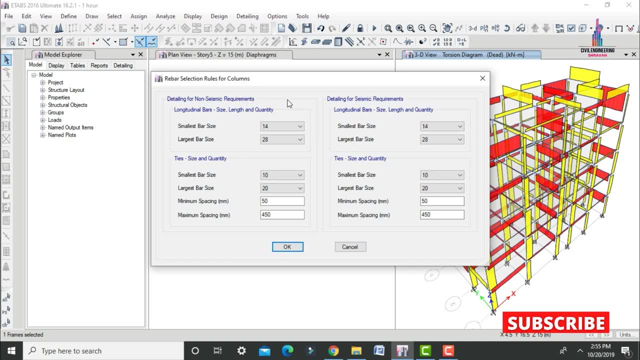 non-seismic requirements. otherwise, if you want to calculate the otherwise, if you want to calculate the otherwise, if you want to calculate the respected, respected, respected uh designing details as per the seismic uh designing details. as per the seismic uh designing details as per the seismic loading considerations. 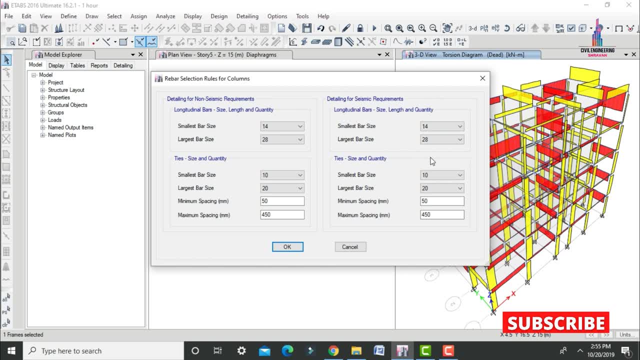 loading considerations. loading considerations only. you need to consider the right hand only you need to consider the right hand only. you need to consider the right hand side section data. so as per the problem side section data. so as per the problem side section data. so as per the problem statement. as per the g plus 4 building. 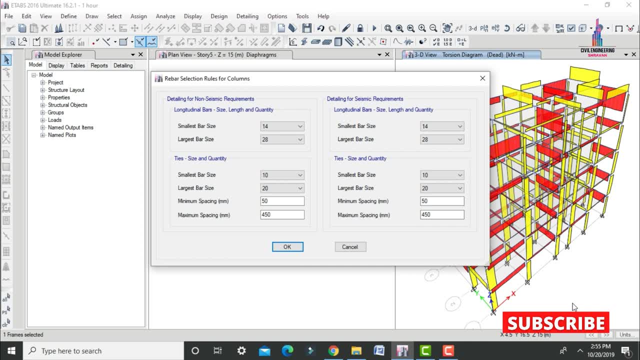 statement. as per the g plus 4 building statement. as per the g plus 4 building design: i was considered the load cases design. i was considered the load cases design. i was considered the load cases which is related to the earthquake load which is related to the earthquake load. 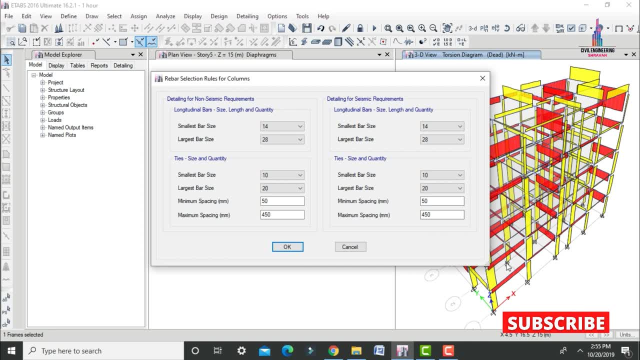 which is related to the earthquake load, as well as wind loading condition. so as well as wind loading condition. so as well as wind loading condition. so that's why just i am selecting the data, that's why just i am selecting the data, that's why just i am selecting the data which is related to the seismic. 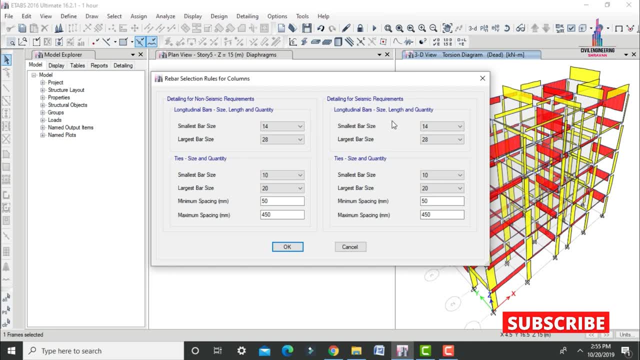 which is related to the seismic, which is related to the seismic requirements, only requirements only requirements only. now we have to select the smallest bar now. we have to select the smallest bar now. we have to select the smallest bar size as well as largest bar size. so, size as well as largest bar size. so 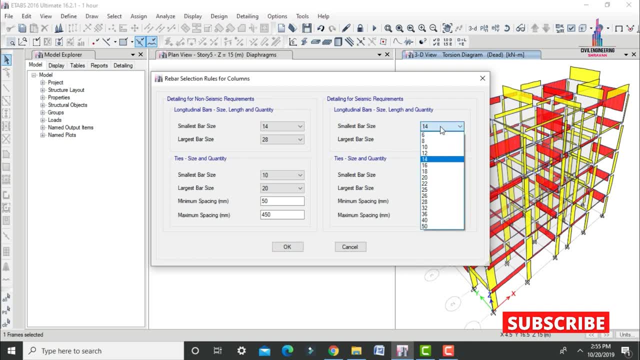 size as well as largest bar size. so here i am selecting the largest bar size. here i am selecting the largest bar size. here i am selecting the largest bar size is 20. again i am selecting smallest bar is 20. again i am selecting smallest bar is 20. again i am selecting smallest bar size is 12. so after that we have to. 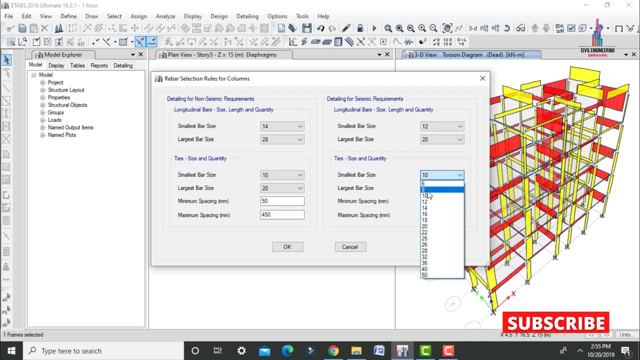 size is 12, so after that we have to size is 12, so after that we have to select the twice bar size. so here i am select the twice bar size. so here i am select the twice bar size. so here i am selecting twice bar size. smallest is 8. 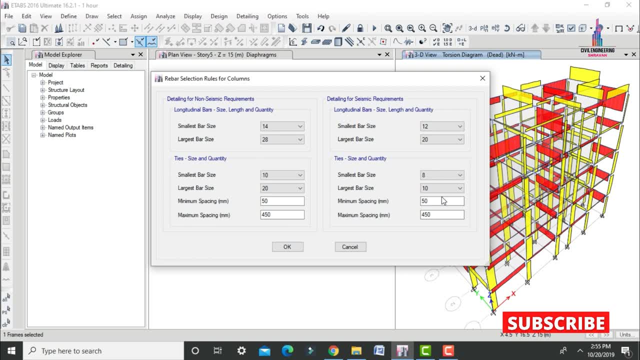 selecting twice bar size: smallest is 8. selecting twice bar size: smallest is 8 and largest is 10. so after that we have, and largest is 10. so after that we have and largest is 10. so after that we have to enter the minimum spacing option. 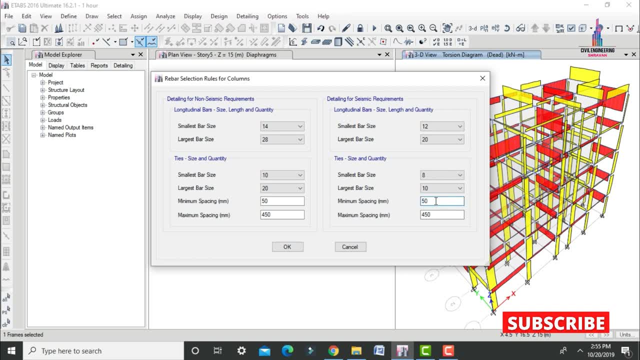 to enter the minimum spacing option. to enter the minimum spacing option, so as per the consideration. we will, so as per the consideration. we will, so as per the consideration. we will consider minimum spacing. consider minimum spacing. consider: minimum spacing is 50 mm. again, i am selecting the 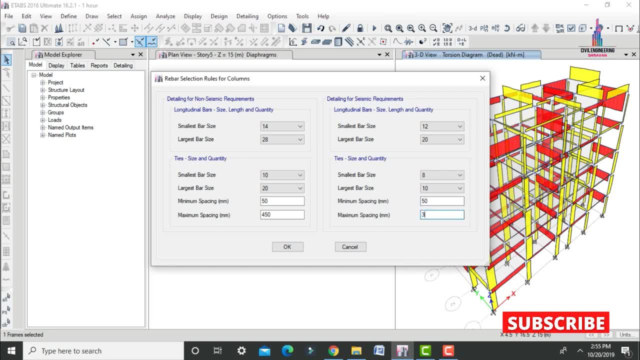 is 50 mm. again i am selecting the is 50 mm. again i am selecting the maximum spacing option. just i am taking maximum spacing option. just i am taking maximum spacing option. just i am taking it as 350, it as 350, it as 350. okay, so click on ok option. so after that, 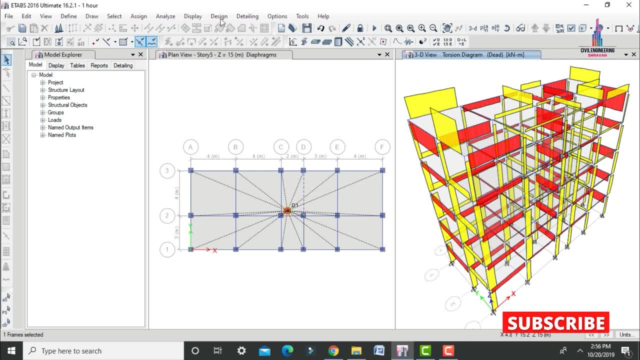 okay, so click on ok option. so after that: okay, so click on ok option. so after that we have to select the detailing for the. we have to select the detailing for the. we have to select the detailing for the. respected column also in the same way. respected column also in the same way. 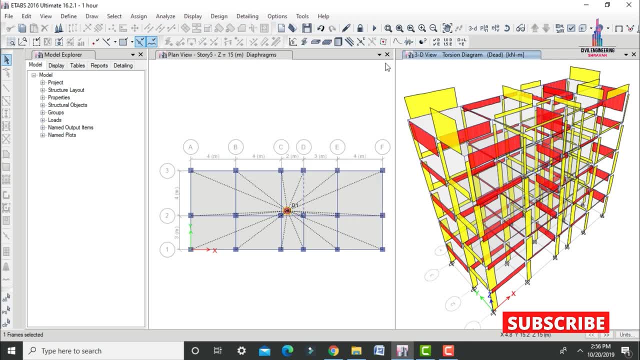 respected column also. in the same way. click on design so click on concrete. click on design, so click on concrete. click on design: so click on concrete frame design. so select the rebar section frame design. so select the rebar section frame design. so select the rebar section. rules for the respected uh beams also. 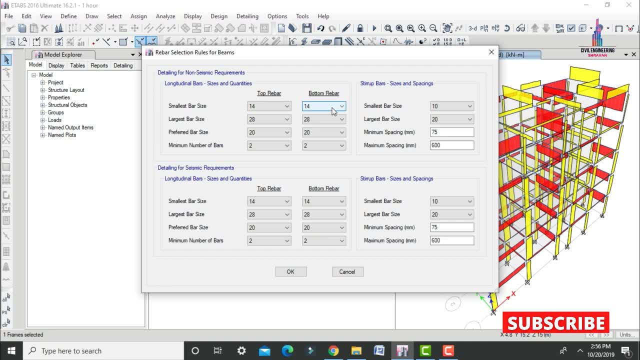 rules for the respected uh beams also. rules for the respected uh beams also. okay, so it is also consisting of two. okay, so it is also consisting of two. okay, so it is also consisting of two types here, which is related to the types here, which is related to the. 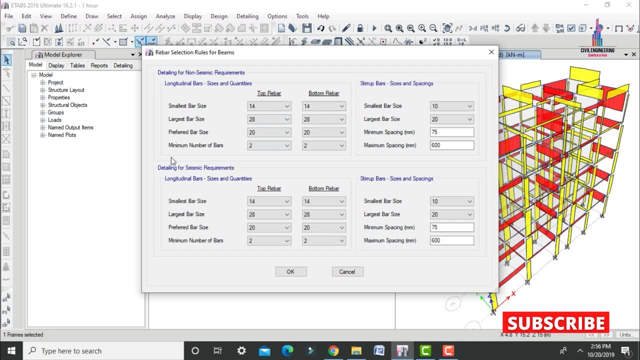 types here, which is related to the non-seismic requirements and seismic non-seismic requirements and seismic non-seismic requirements and seismic requirements and for this respected requirements and for this respected requirements and for this respected building. just, i was considering the building, just i was considering the. 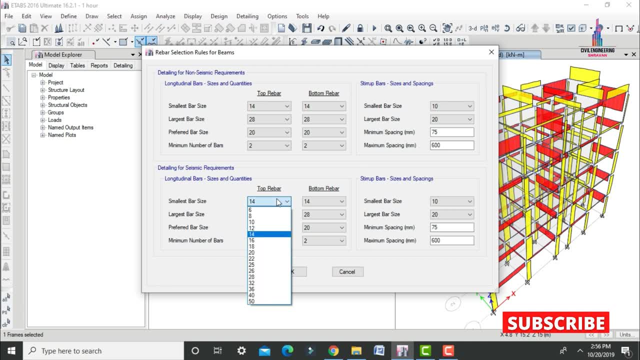 building. just i was considering the seismic loading condition. that's why i'm seismic loading condition, that's why i'm seismic loading condition, that's why i'm taking this. so here we have to select taking this. so here we have to select taking this. so here we have to select the smallest bar size. just i'm. 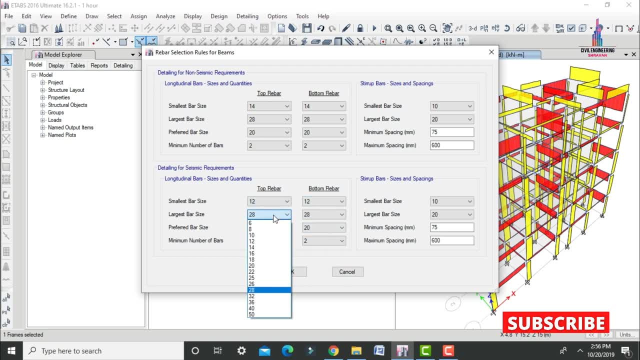 the smallest bar size. just i'm the smallest bar size, just i'm considering it as 12 mm bar. again i'm considering it as 12 mm bar. again i'm considering it as 12 mm bar again. i'm selecting the largest bar size, which is: 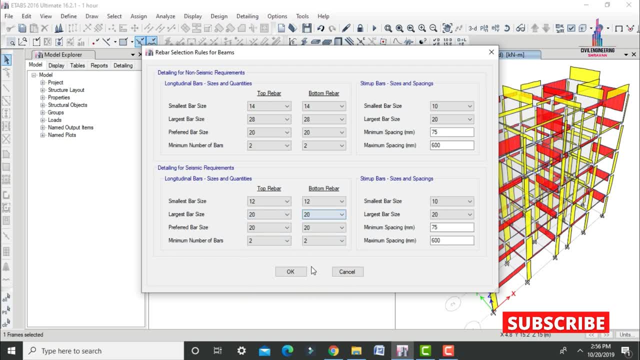 selecting the largest bar size, which is selecting the largest bar size, which is equals to 20 mm bars. now we have to equals to 20 mm bars. now we have to equals to 20 mm bars. now we have to select the preferred bar size. so, select the preferred bar size. so 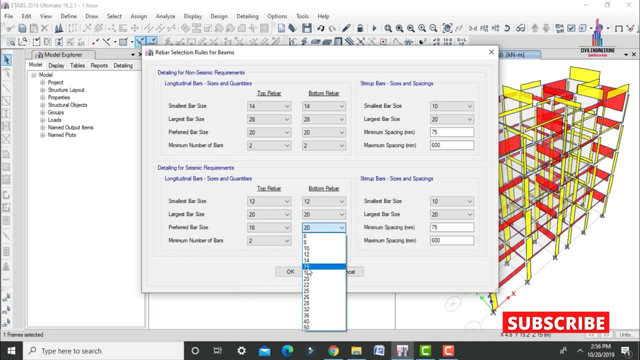 select the preferred bar size. so, preferred by size, just i'm taking it as preferred by size, just i'm taking it as preferred by size. just i'm taking it as 16 mm bars. 16 mm bars, 16 mm bars. again we have to enter the number of. 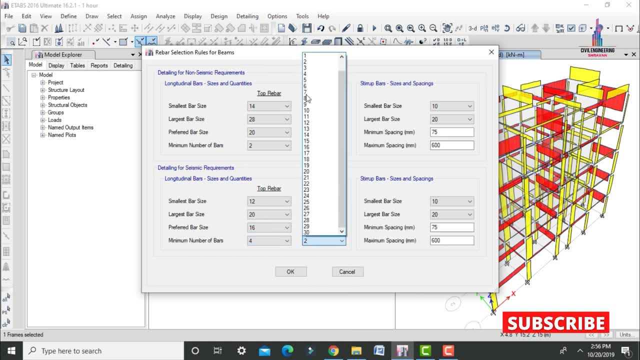 again we have to enter the number of. again we have to enter the number of bars here, so select it as. let us assume bars here. so select it as. let us assume bars here. so select it as. let us assume it as four. again, i'm selecting it as. 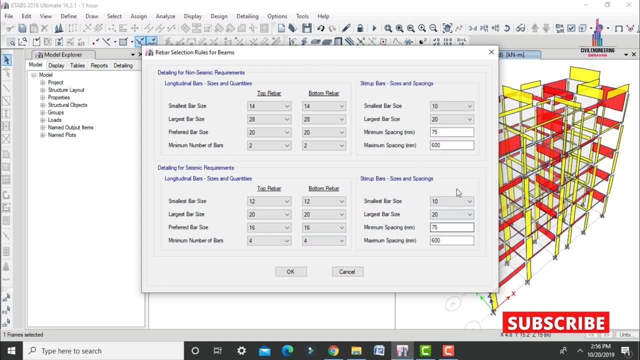 it as four. again i'm selecting it as it as four. again i'm selecting it as four. so after that we have to select the four. so after that we have to select the four. so after that we have to select the stirrups data. so here i'm selecting the. 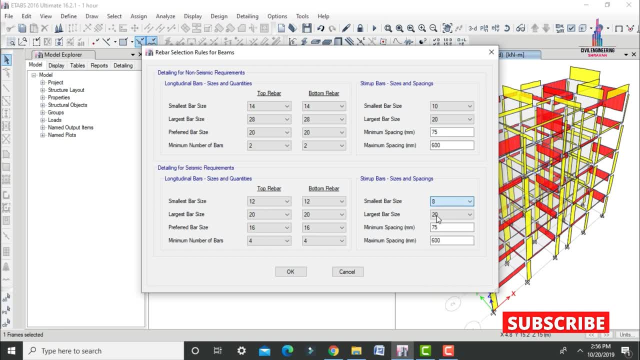 stirrups data. so here i'm selecting the stirrups data. so here i'm selecting the stirrups data: uh- largest bar size. so stirrups data. uh- largest bar size. so stirrups data. uh- largest bar size. so sorry, smallest bar size is 8 and largest. sorry, smallest bar size is 8 and largest sorry. smallest bar size is 8 and largest bar size is 10.. so again we have to. bar size is 10.. so again we have to. bar size is 10.. so again we have to enter the minimum spacing and maximum. 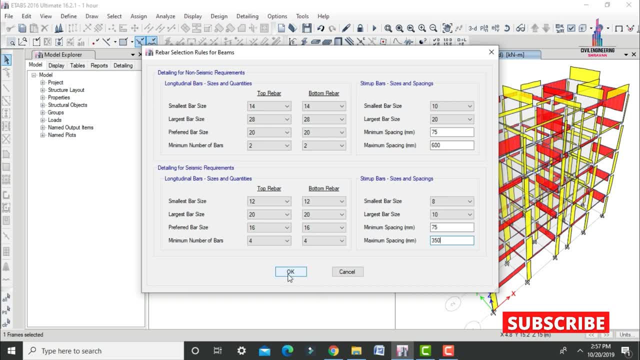 enter the minimum spacing and maximum. enter the minimum spacing and maximum spacing. just i'm taking it as maximum spacing, just i'm taking it as maximum spacing, just i'm taking it as maximum as 150 here. click on ok option. so after. as 150 here. click on ok option, so after. 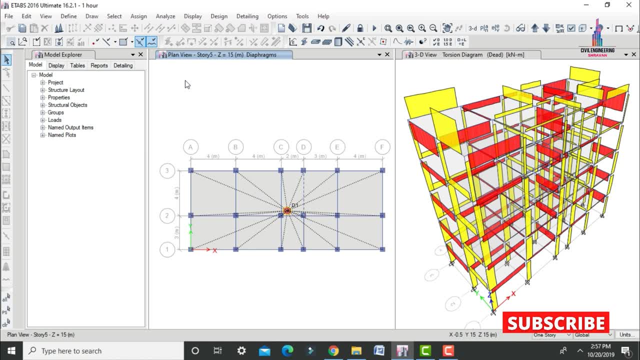 as 150 here. click on ok option. so after that, we need to check the data, which is that we need to check the data, which is that we need to check the data which is related to the start design checks for. related to the start design checks for. 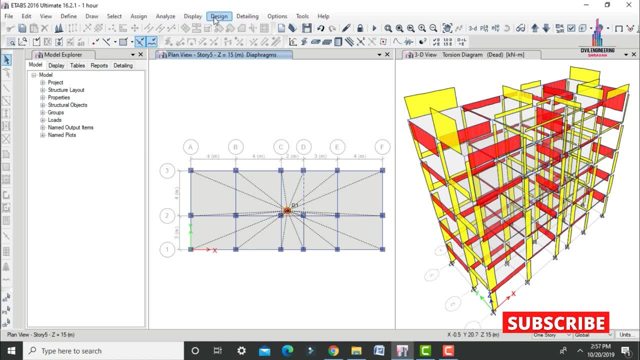 related to the start design checks for the column and beam sections. so click on the column and beam sections. so click on the column and beam sections. so click on our design option. here so select the our design option. here so select the our design option. here so select the concrete frame design. so here we need to. 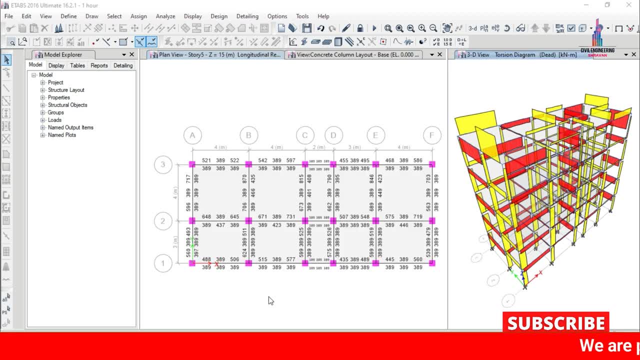 concrete frame design. so here we need to concrete frame design. so here we need to click on stat design checks here. so it click on stat design checks here. so it click on stat design checks here so it will show your respective reinforcement, will show your respective reinforcement, will show your respective reinforcement value diagram here, like this: so this is. 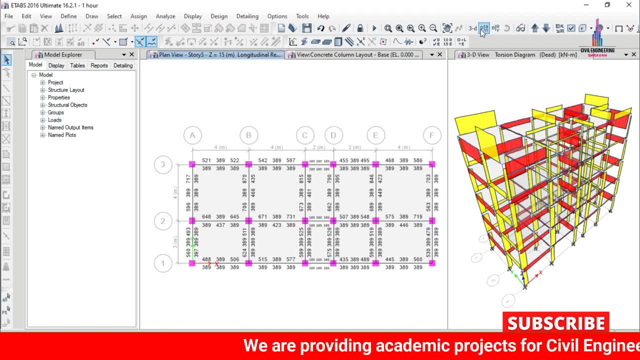 value diagram here like this: so this is value diagram here. like this: so this is the hd requirement for the different, the hd requirement for the different, the hd requirement for the different members. i will show you this diagram in members. i will show you this diagram in members. i will show you this diagram in 3d view. click on 3d view option. so. 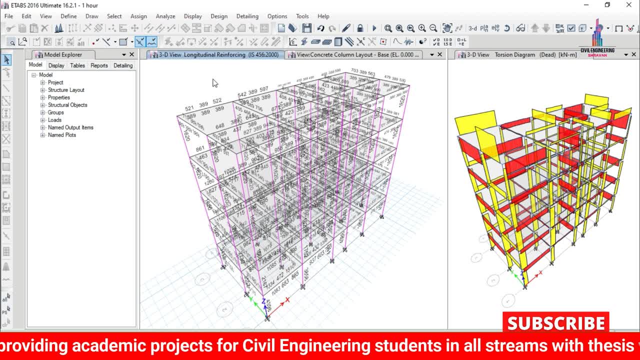 3d view: click on 3d view option. so 3d view: click on 3d view option. so after that, we have to see this respected. after that, we have to see this respected. after that, we have to see this respected. values as per the reinforcement section. 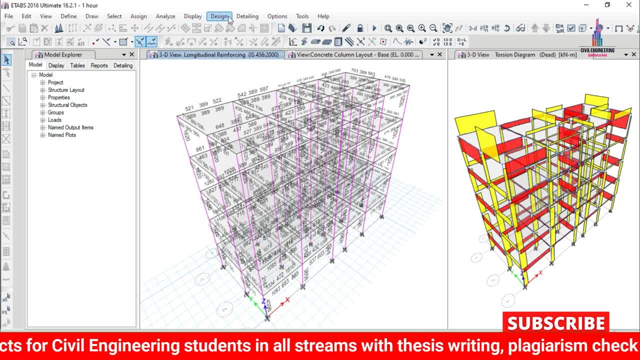 values as per the reinforcement section. values as per the reinforcement section of beams and columns of beams and columns of beams and columns. so click on design again. again we have to. so click on design, again, again we have to. so click on design again. again we have to select the. 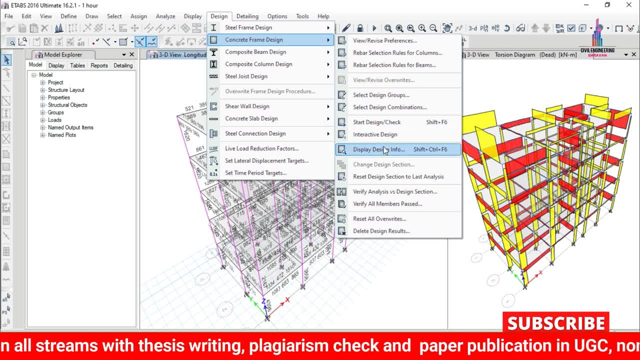 select the select the concrete design. so here i'm selecting concrete design. so here i'm selecting concrete design. so here we have to click on display concrete design. so here we have to click on display concrete design. so here we have to click on display design information, design information. 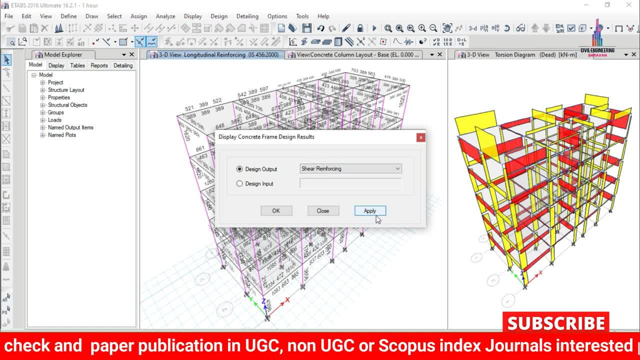 design information: now, here we have to select the display. now here we have to select the display. now here we have to select the display design information as per the shear design information: as per the shear design information as per the shear reinforcing section. so it will show your 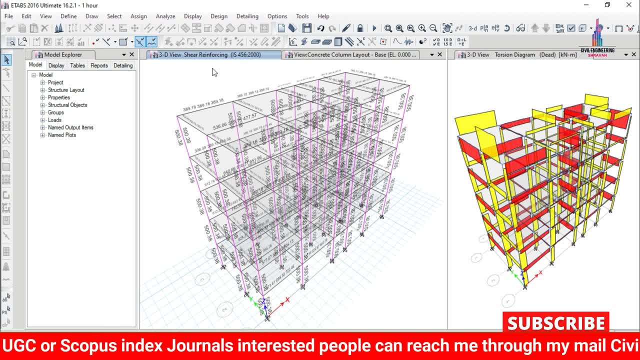 reinforcing section. so it will show your reinforcing section. so it will show your respected beam section and column. respected beam section and column. respected beam section and column section. different types of reinforcement section. different types of reinforcement section. different types of reinforcement section. so after that we have to detail. 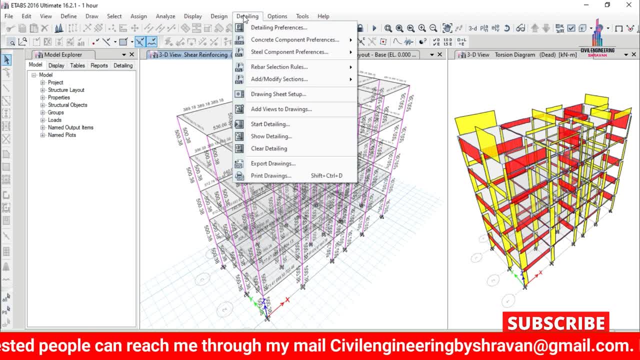 section. so after that we have to detail section. so after that we have to detail this respected beam design column design. this respected beam design column design. this respected beam design column design sections. so click on detailing option sections. so click on detailing option sections. so click on detailing option. initially we need to select the. 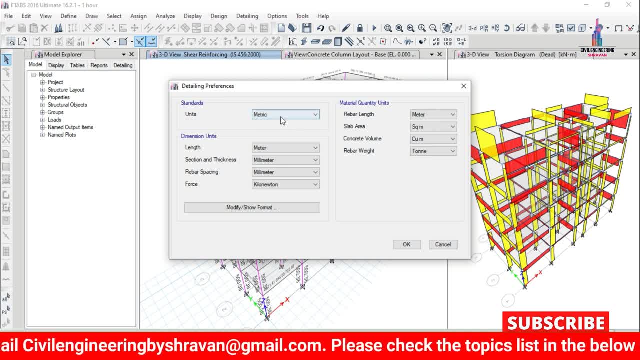 initially we need to select the. initially we need to select the preferences. so here we have to select the preferences. so here we have to select the preferences. so here we have to select the standard units will be in metric. standard units will be in metric. standard units will be in metric system length will be in meter and. 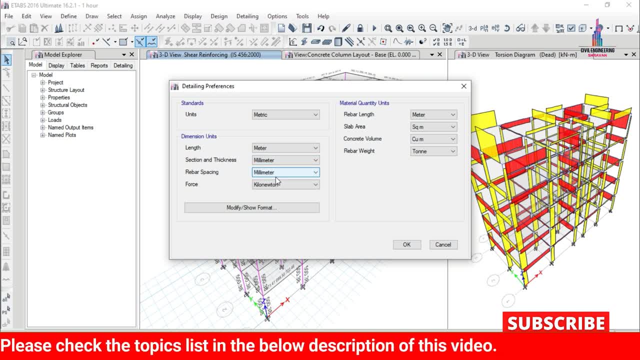 system length will be in meter and system length will be in meter and section thickness will be in millimeter. section thickness will be in millimeter. section thickness will be in millimeter and rebar spacing will be in millimeter and rebar spacing will be in millimeter. 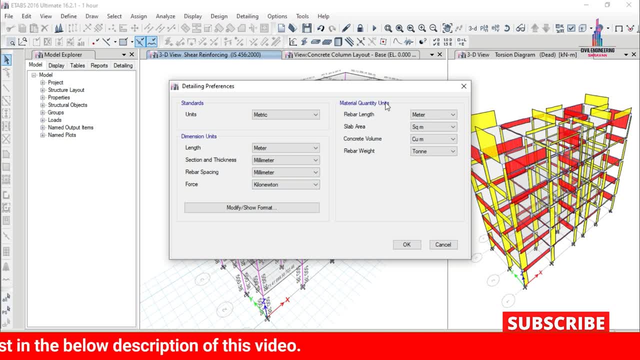 and rebar spacing will be in millimeter, and force will be in kilometer, so after. and force will be in kilometer, so after and force will be in kilometer, so after that, we have to select the material that we have to select the material that we have to select the material quality as per the meter square meter. 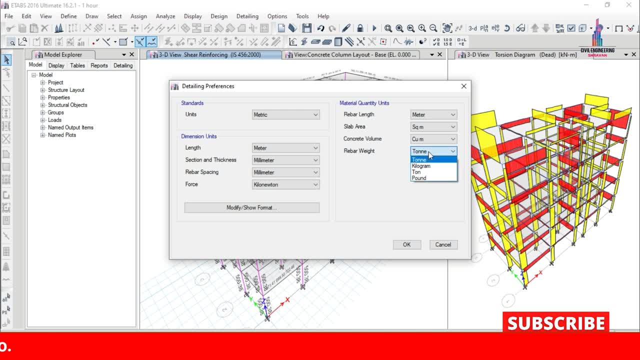 quality as per the meter square meter. quality as per the meter square meter, cubic meter and ton. so here we have to cubic meter and ton. so here we have to cubic meter and ton. so here we have to select the select, the select the uh ton values. so here we have to select. 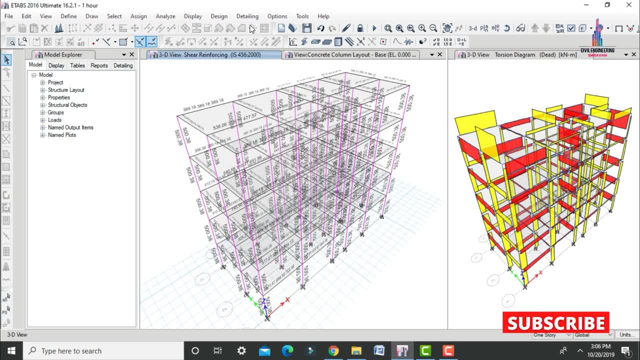 uh ton values. so here we have to select uh ton values. so here we have to select the ton. so after that click on. okay, okay, the ton. so after that click on. okay, okay, the ton. so after that click on. okay, okay. so after that we have to click on. 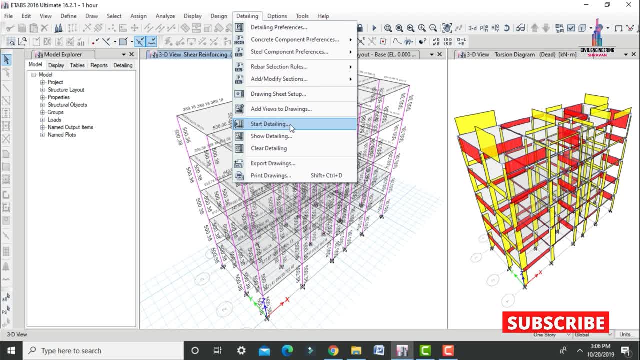 so after that we have to click on. so after that we have to click on detailing again. again we have to click detailing again. again we have to click detailing again. again we have to click on stat detailing option here, so click on on stat detailing option here, so click on. 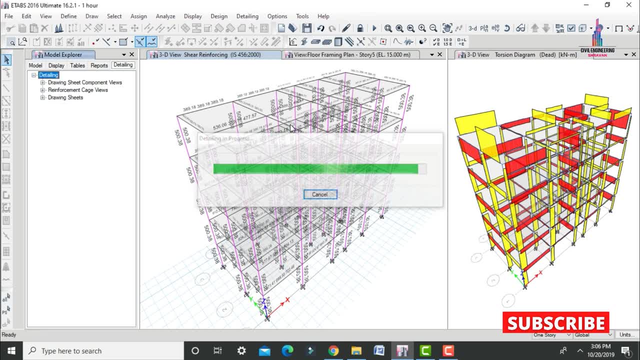 on stat detailing option here. so click on stat detailing option here so it will stat detailing option here. so it will stat detailing option here so it will show your respected designing here like: show your respected designing here. like: show your respected designing here like this: so it will design this respected. 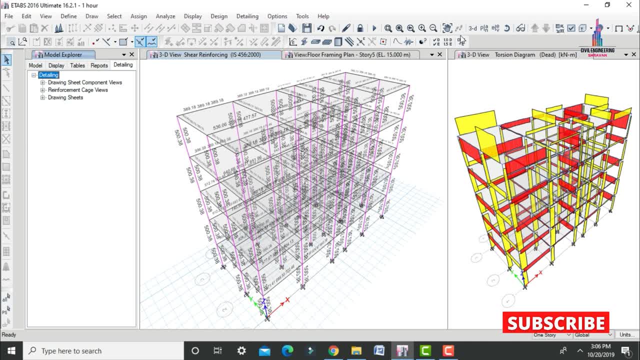 this, so it will design this. respected this, so it will design this. respected building structure, so i will show you building structure. so i will show you building structure. so i will show you that respected reinforcement values. now that respected reinforcement values. now that respected reinforcement values now. so for displaying the information which 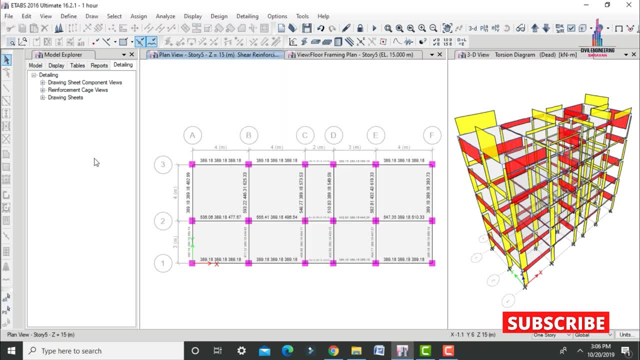 so for displaying the information which. so for displaying the information which is related to the beam design section, is related to the beam design section, is related to the beam design section. column design section. column design section. column design section. results. so we have to select this. results. so we have to select this. 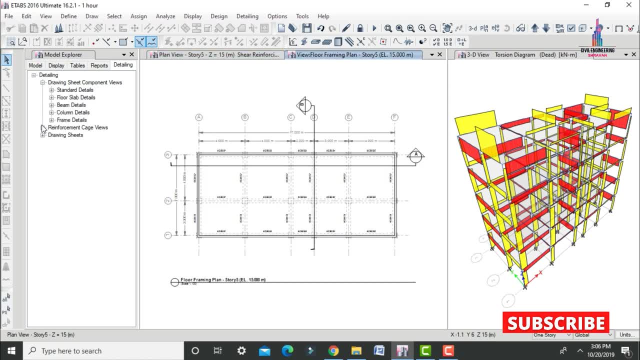 results. so we have to select this detailing option. so it will be detailing option. so it will be detailing option. so it will be consisting of drawing sheet components, consisting of drawing sheet components, consisting of drawing sheet components. and reinforcement cage views: okay, and reinforcement cage views: okay, and reinforcement cage views: okay. initially, i will explain you that. 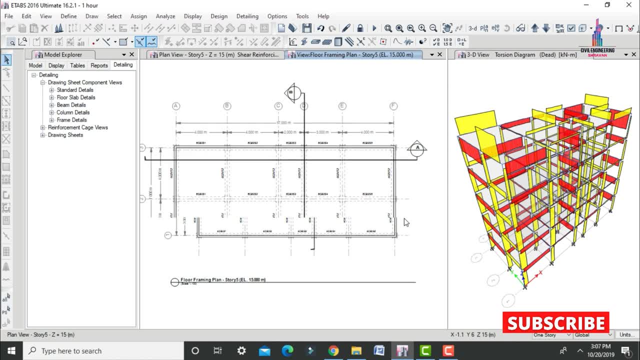 initially, i will explain you that. initially, i will explain you that respected detailings: okay, so this is the respected detailings. okay, so this is the respected detailings. okay, so this is the diagram after designing of this diagram. after designing of this diagram, after designing of this respected building, it will be showing. 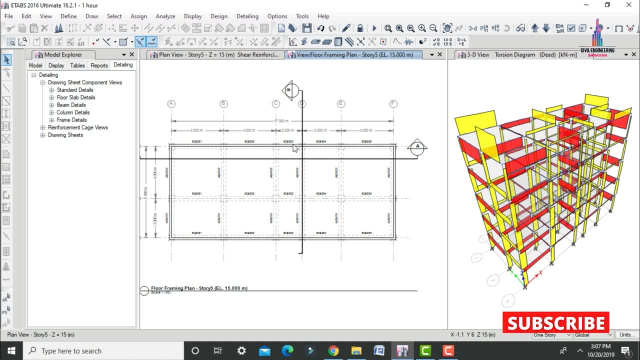 respected building. it will be showing respected building. it will be showing here like this: so it will be consisting here like this: so it will be consisting here like this: so it will be consisting of your beam sections and beam numbering of your beam sections and beam numbering of your beam sections and beam numbering. and center to center distance between: 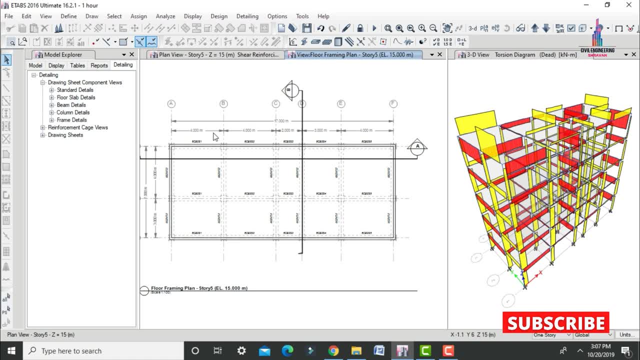 and center to center distance between and center to center distance between the columns. okay, so this is the length the columns. okay, so this is the length the columns. okay, so this is the length of the building, which is approximately of the building, which is approximately of the building, which is approximately equal to 4 plus 4 plus 2 plus 3 plus 4. equal to 4 plus 4 plus 2 plus 3 plus 4. equal to 4 plus 4 plus 2 plus 3 plus 4, which is equals to 17 meter, and width of which is equals to 17 meter and width of. 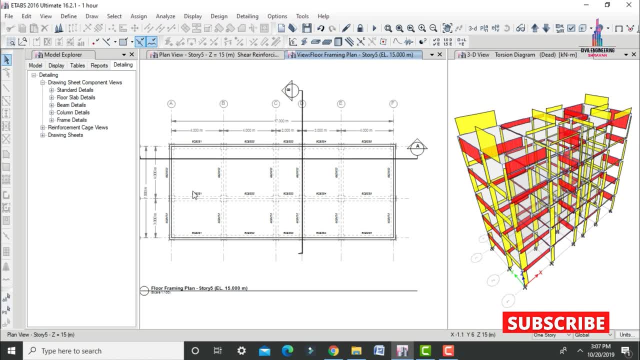 which is equals to 17 meter, and width of the building is 3 plus 4, which is equals the building is 3 plus 4, which is equals the building is 3 plus 4, which is equals to 7 meter. okay, so after that we have to. 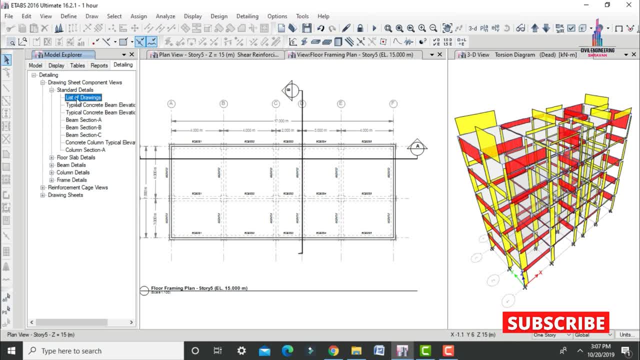 to 7 meter. okay, so after that we have to to 7 meter. okay, so after that we have to select the standard details here. select the standard details here. select the standard details here. so select the list of drawings here. so. so select the list of drawings here. so select the building: uh elevation. 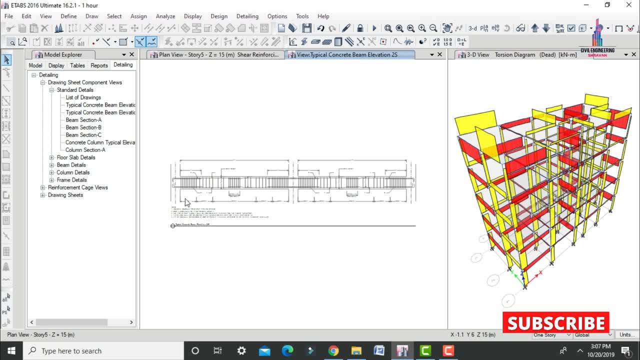 select the building uh elevation. select the building uh elevation- section 2s section. so this is the 2s section, 2s section. so this is the 2s section, 2s section. so this is the 2s section, which is consisting of different. 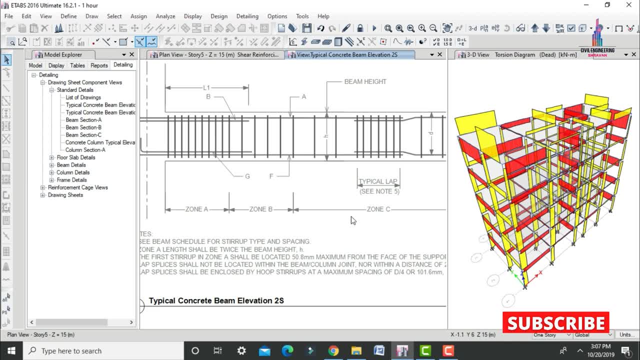 section which is consisting of different section, which is consisting of different types of zones. here you can zoom this. so types of zones: here you can zoom this. so types of zones: here you can zoom this. so this is the zone a, zone b, zone c section. this is the zone a, zone b, zone c section. 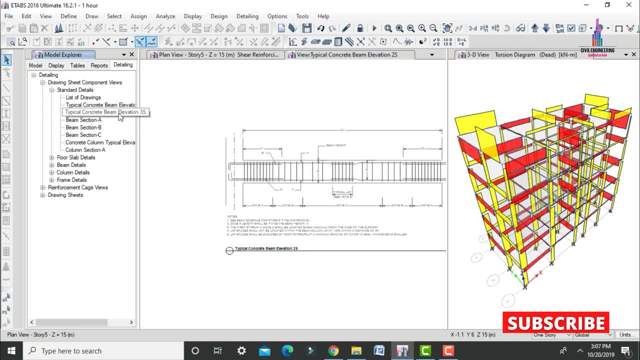 this is the zone a, zone b, zone c section for the typical beam section. okay again for the typical beam section. okay again for the typical beam section. okay again, i am selecting the typical beam section. i am selecting the typical beam section. i am selecting the typical beam section for the 3s section. so this is a 3s. 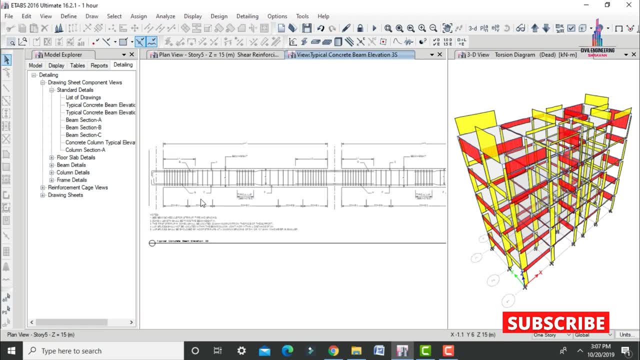 for the 3s section. so this is a 3s section. typical elevation section. again section typical elevation section. again section typical elevation section. again, it will be consisting of zones here. it will be consisting of zones here. it will be consisting of zones here like this: zone a, zone b, zone c, zone a is. 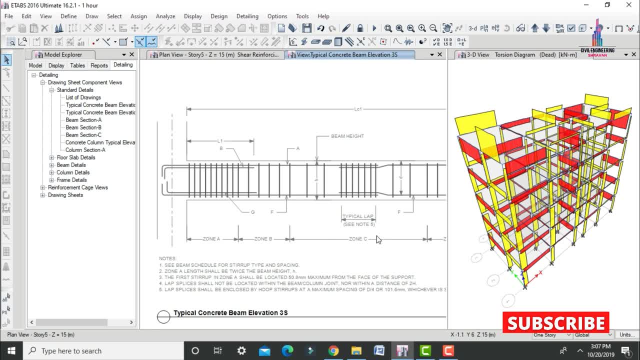 like this: zone a, zone b, zone c. zone a is like this: zone a, zone b, zone c, zone a is nothing but the corner section and zone, nothing but the corner section and zone, nothing but the corner section. and zone c is nothing but the ending point of. 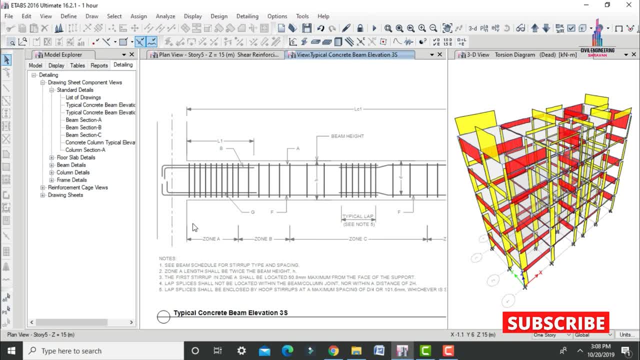 c is nothing, but the ending point of c is nothing, but the ending point of this restricted reinforcement section, this restricted reinforcement section, this restricted reinforcement section, and zone b is nothing but the center and zone b is nothing, but the center and zone b is nothing but the center section, elevation section. so after that, 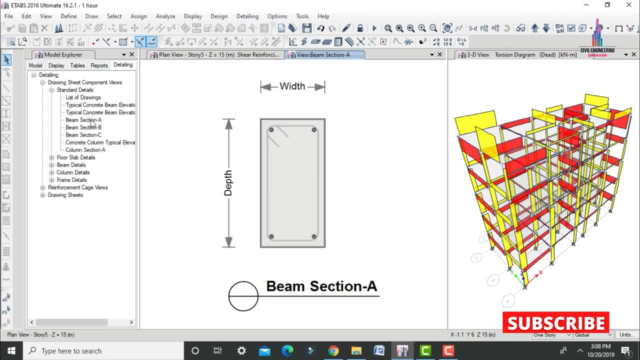 section: elevation section. so after that section, elevation section. so after that, in the same way we have to select the, in the same way we have to select the, in the same way we have to select the concrete elevation section. again it is: concrete elevation section. again it is. 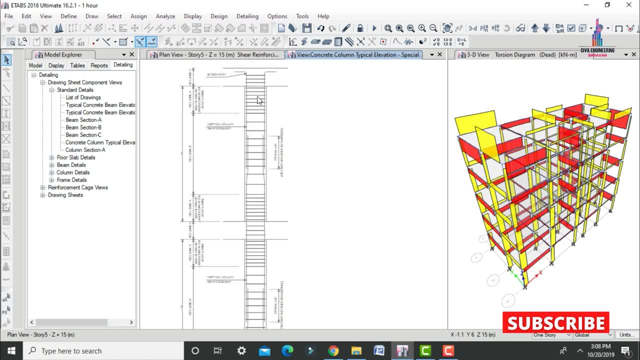 concrete elevation section. again, it is also consisting of different types of. also consisting of different types of. also consisting of different types of zones and different reinforcement zones and different reinforcement zones and different reinforcement sections. again i'm selecting column sections. again i'm selecting column sections. again i'm selecting column section a. okay, so this is the diagram. 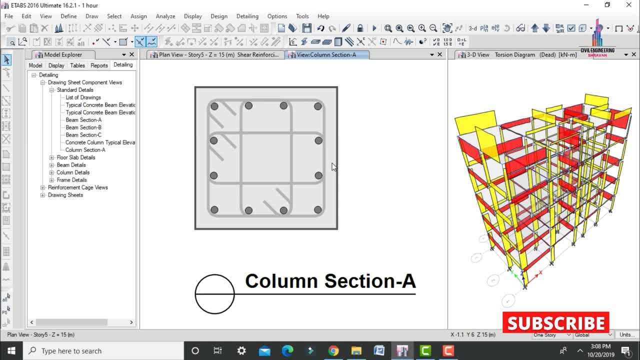 section a. okay, so this is the diagram, section a: okay, so this is the diagram which is related to the column section a, which is related to the column section a, which is related to the column section a: a section, so after that we have to a section, so after that we have to. 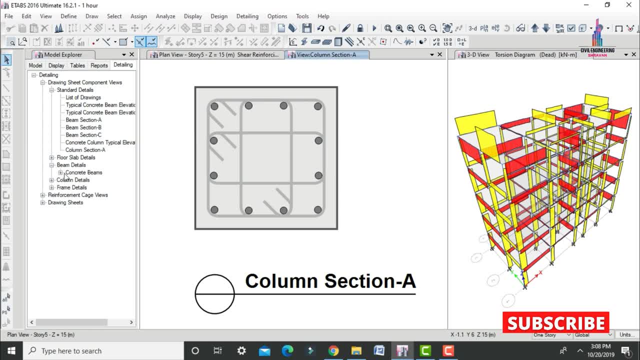 a section. so after that we have to select the beam detailing options here. select the beam detailing options here. select the beam detailing options here. okay, we have to check the output values. okay, we have to check the output values. okay, we have to check the output values for the detailing of the beams. okay, so 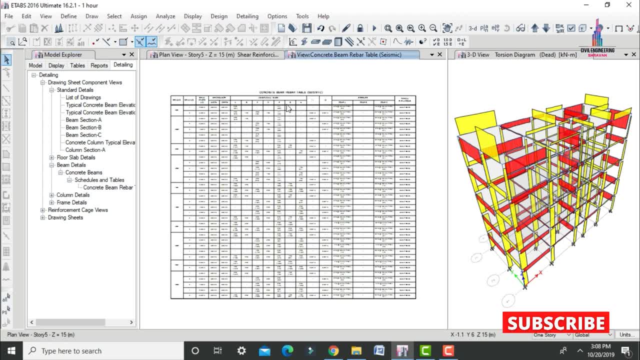 for the detailing of the beams. okay, so for the detailing of the beams. okay. so here i'm selecting beam detailing. here i'm selecting beam detailing. here i'm selecting beam detailing. schedules and bars. select this concrete schedules and bars. select this concrete schedules and bars. select this concrete section, so it will be consisting of the. 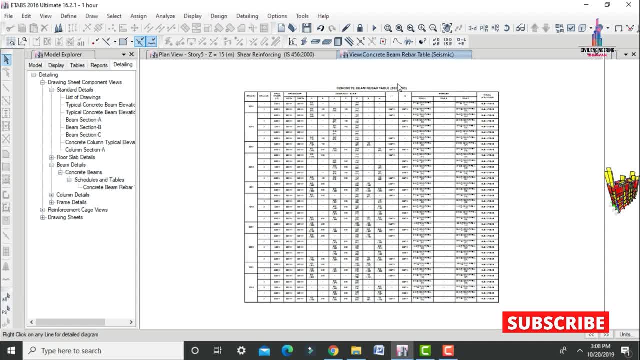 section, so it will be consisting of the section. so it will be consisting of the output file here, like this: okay, so it output file here. like this: okay, so it output file here. like this: okay, so it will be consisting of each and individual will be consisting of each and individual. 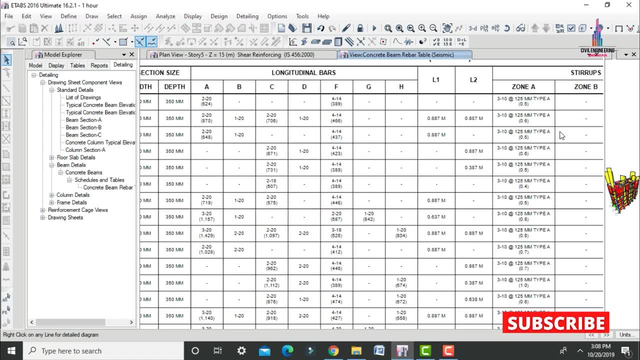 will be consisting of each and individual section. member design results like this section. member design results like this section. member design results like this: okay, so this is the excel sheet and this. okay, so this is the excel sheet and this. okay, so this is the excel sheet and this is the tabular format we need to take for 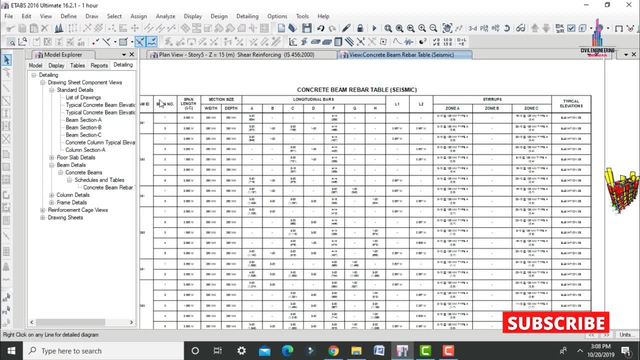 is the tabular format we need to take, for is the tabular format we need to take for the designing of any kind of the, the designing of any kind of the, the designing of any kind of the building, for example. let us consider the building. for example, let us consider the. 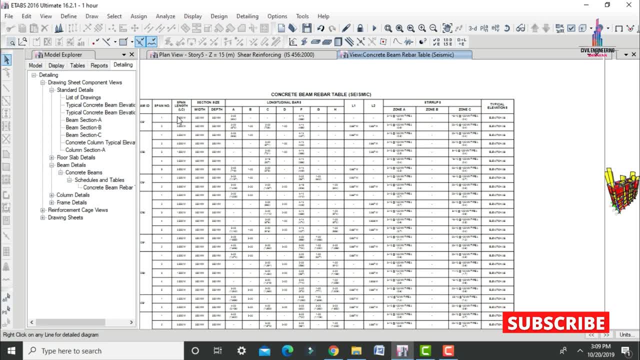 building. for example, let us consider the bill uh beam number one, which is having bill uh beam number one, which is having bill uh beam number one, which is having a span of one and which is having the a span of one and which is having the a span of one and which is having the length of the beam is 2.550 meter and 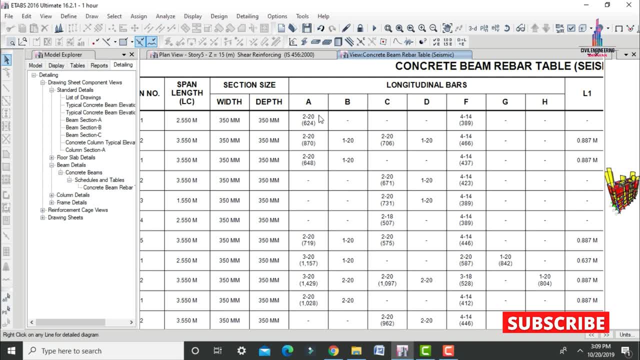 length of the beam is 2.550 meter and length of the beam is 2.550 meter and width is 350 cross 350. for longitudinal width is 350 cross 350. for longitudinal width is 350 cross 350. for longitudinal bars it is required two bars of 20 mm. 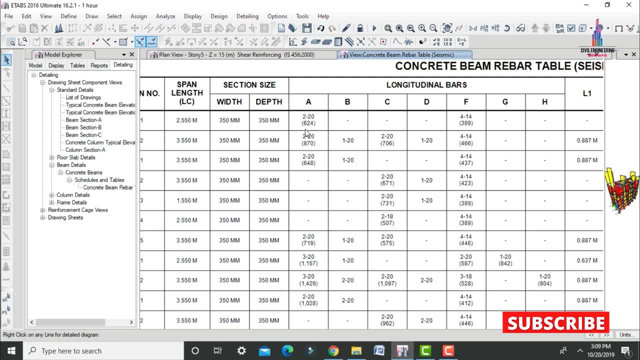 bars. it is required two bars of 20 mm bars. it is required two bars of 20 mm. okay which is having ast percentage and okay which is having ast percentage and okay which is having ast percentage and ast requirement is 624 mm square at the ast requirement is 624 mm square at the 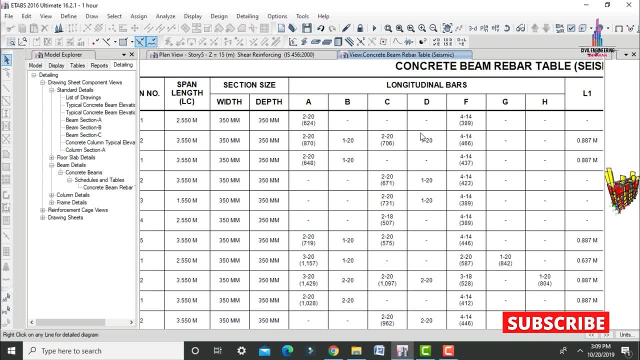 ast requirement is 624 mm square at the. a section. reinforcement b. section c. a section. reinforcement b. section c. a section. reinforcement b. section c. section d section will be empty and f section d section will be empty and f section d section will be empty and f section will be equals to four bars of. 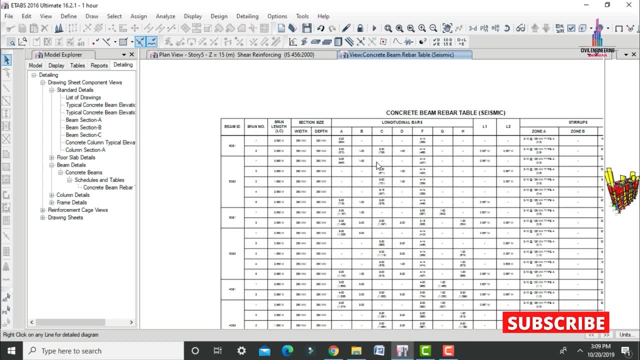 section will be equals to four bars of section will be equals to four bars of 14 mm dia. 14 mm dia, 14 mm dia. okay, again in the same way, we have to okay, again in the same way, we have to okay again. in the same way, we have to check the stirrups data, also okay, so 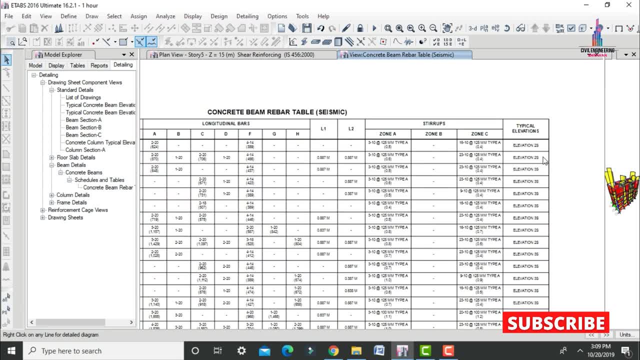 check the stirrups data also. okay. so check the stirrups data also. okay. so this is the stirrups data on the right. this is the stirrups data on the right. this is the stirrups data on the right hand side section. so it is also. 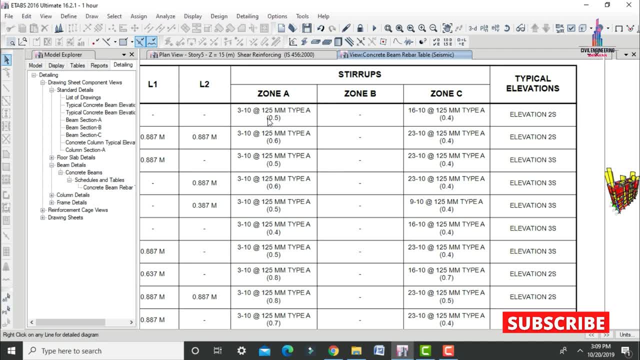 hand side section, so it is also hand side section, so it is also consisting of zones here, as per the consisting of zones here, as per the consisting of zones here, as per the considerations, so it will be consisting considerations, so it will be consisting considerations. so it will be consisting of the three bars of 10 mm, dia 125. 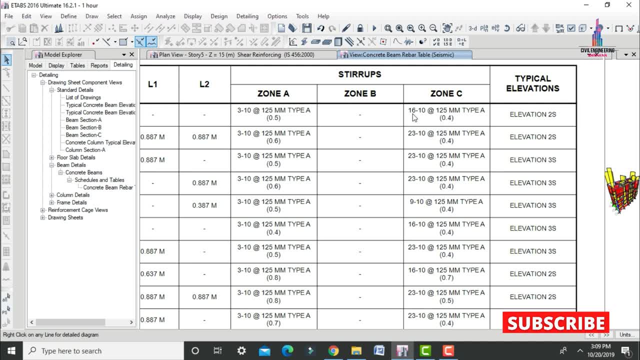 of the three bars of 10 mm dia 125. of the three bars of 10 mm dia 125 center to center distance for the 2a center to center distance for the 2a center to center distance for the 2a section. it will be consisting of 16 bars. 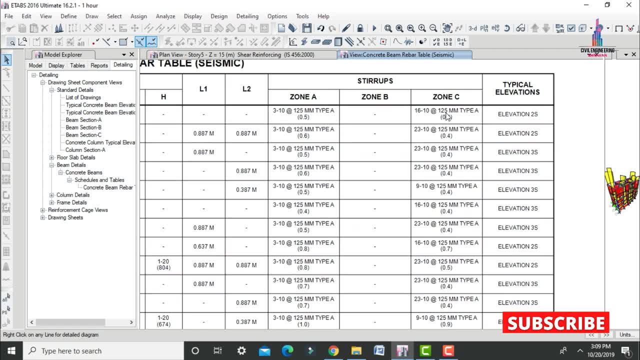 section. it will be consisting of 16 bars section. it will be consisting of 16 bars of 10 mm dia and 125 center to center of 10 mm dia and 125 center to center of 10 mm dia and 125 center to center distance for this respected section. okay. distance for this respected section: okay, distance for this respected section: okay. so, again in the same way, we have to so, again in the same way, we have to so, again in the same way, we have to check the data which is related to the, check the data which is related to the. 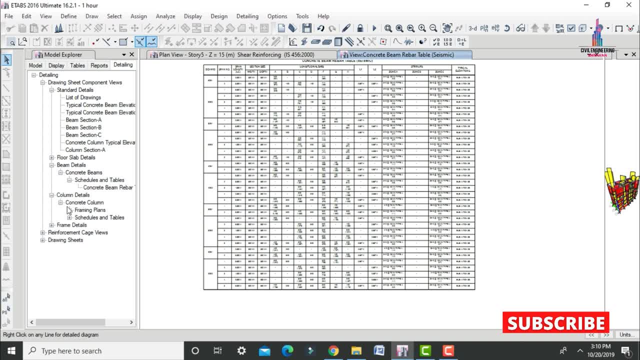 check the data which is related to the column. also again we have to click on column. also again we have to click on column. also again we have to click on column detailing. so click on concrete column detailing. so click on concrete column detailing. so click on concrete column. framing plans- so click on this. so 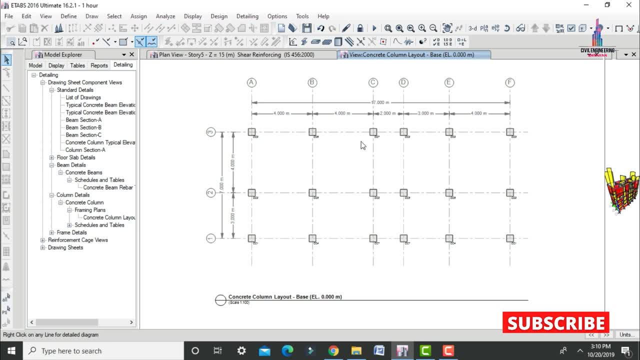 column framing plans, so click on this. so column framing plans, so click on this. so this is the framing plan for this. this is the framing plan for this. this is the framing plan for this. respected column section, which is respected. column section which is respected. column section which is nothing but the center to center. 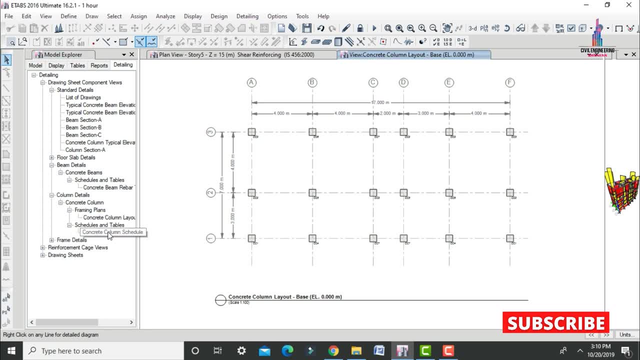 nothing but the center to center, nothing but the center to center. distance between the columns: okay so. distance between the columns: okay so distance between the columns, okay. so again i am selecting schedule. select the. again i am selecting schedule. select the. again i am selecting schedule. select the concrete column schedule. so here we have. 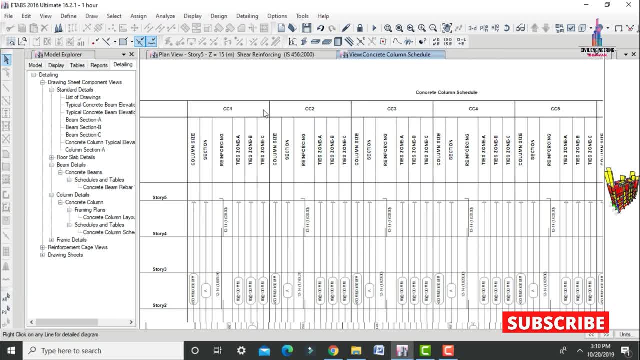 concrete column schedule. so here we have concrete column schedule. so here we have to select this respected option. okay, so, to select this respected option. okay, so to select this respected option. okay. so it will be consisting of the column, it will be consisting of the column, it will be consisting of the column number and column size section. 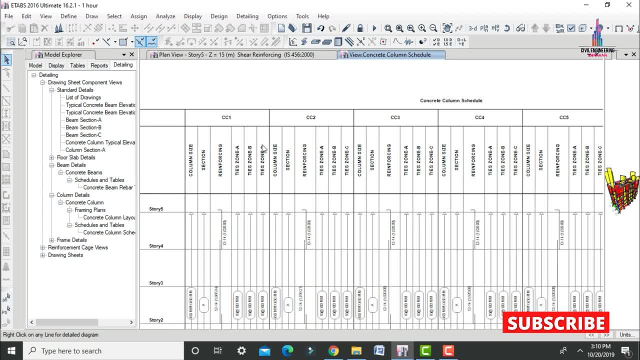 number and column size: section number and column size: section: reinforcing and twice jma zone b- zone c reinforcing and twice jma zone b- zone c reinforcing and twice jma zone b- zone c section. so it will be consisting of 12 section. so it will be consisting of 12. 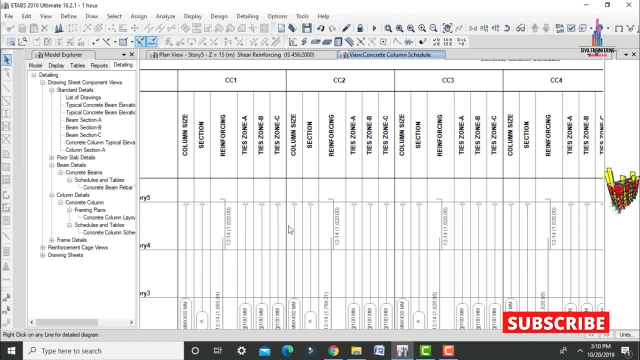 section, so it will be consisting of 12 bars of and 14 mm dia okay, which is bars of, and 14 mm dia okay, which is bars of, and 14 mm dia okay, which is consisting of the longitudinal section. consisting of the longitudinal section. consisting of the longitudinal section. reinforcement for the different types of. 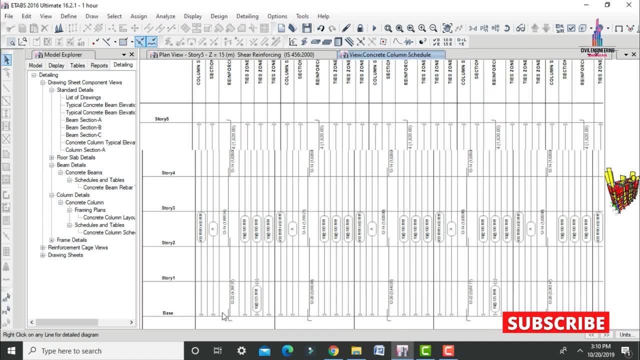 reinforcement for the different types of reinforcement, for the different types of the stories here. okay, it will be the stories here. okay, it will be the stories here. okay, it will be consisting of the reinforcement values, of consisting of the reinforcement values, of consisting of the reinforcement values of 12 bars of 22 mm dia at the base. again, 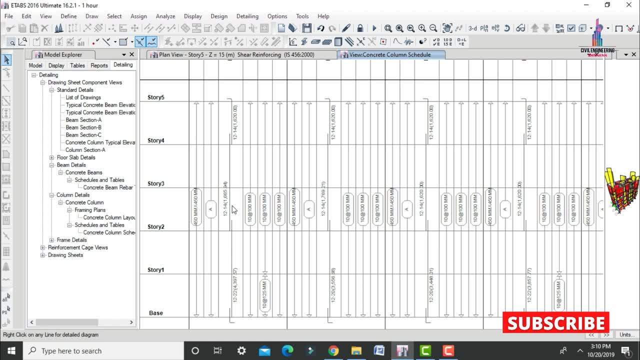 12 bars of 22 mm dia at the base. again 12 bars of 22 mm dia at the base. again, it will be consisting of 12 bars of 14. it will be consisting of 12 bars of 14. it will be consisting of 12 bars of 14 mm dia at the second story to the 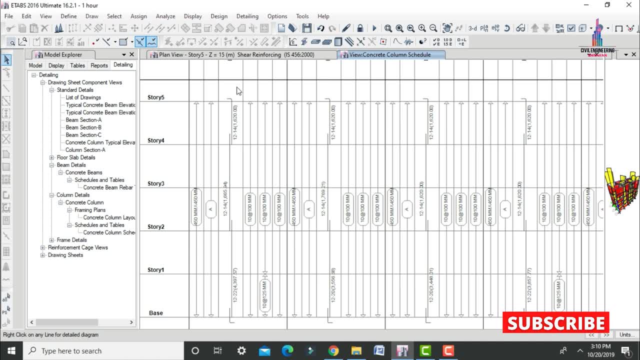 mm dia at the second story, to the mm dia at the second story, to the third story data and fourth story data, third story data and fourth story data, third story data and fourth story data. and at the end of the last story it will, and at the end of the last story it will. 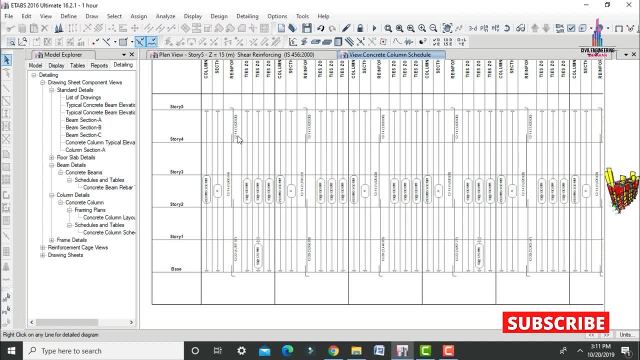 and at the end of the last story, it will be consisting of 12 bars of 14 mm dia. be consisting of 12 bars of 14 mm dia. be consisting of 12 bars of 14 mm dia for the respective section of cc1 column. 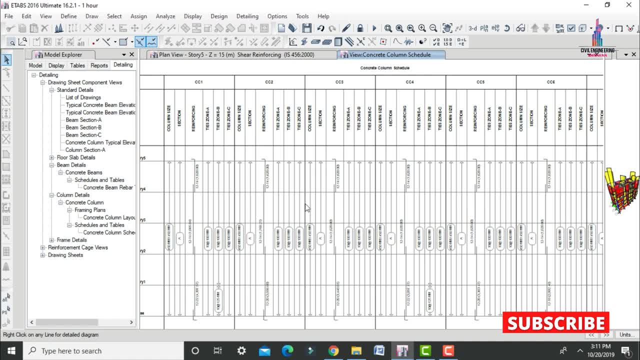 for the respective section of cc1 column. for the respective section of cc1 column. in the same way you can check the data. in the same way you can check the data. in the same way, you can check the data which is related to the cc2 column. 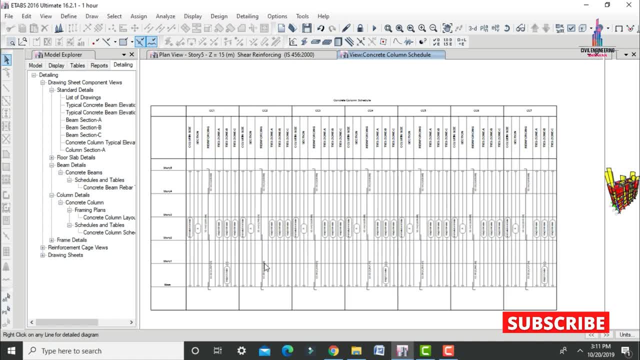 which is related to the cc2 column, which is related to the cc2 column again. it is also consisting of the. again it is also consisting of the. again it is also consisting of the different types of the reinforcement, different types of the reinforcement, different types of the reinforcement values at the ground story. and that the 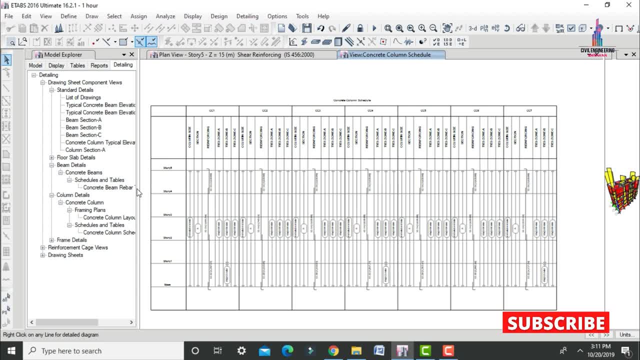 values at the ground story and that the values at the ground story and that the middle stories at the top stories. so middle stories at the top stories, so middle stories at the top stories. so after that we have to check the data. after that we have to check the data. 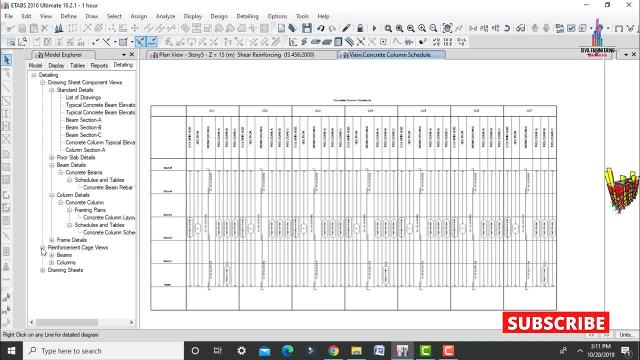 after that, we have to check the data which is related to the reinforcement, which is related to the reinforcement, which is related to the reinforcement. cage views. cage views. cage views. select this option. select the beams here. select this option. select the beams here. select this option. select the beams here, so it will be consisting of different. 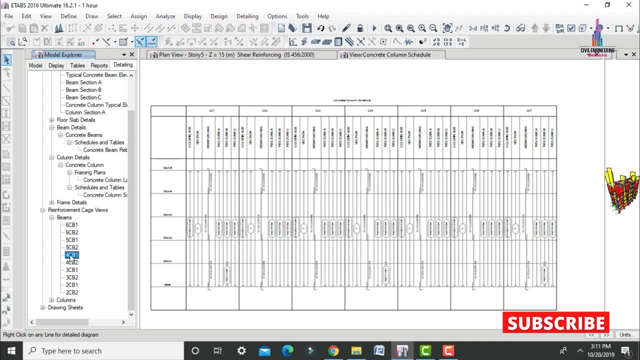 so it will be consisting of different. so it will be consisting of different types of beams, as per the types of beams. as per the types of beams. as per the considerations: you can select any one considerations. you can select any one considerations. you can select any one of the beam. just i'm selecting 4cb1. 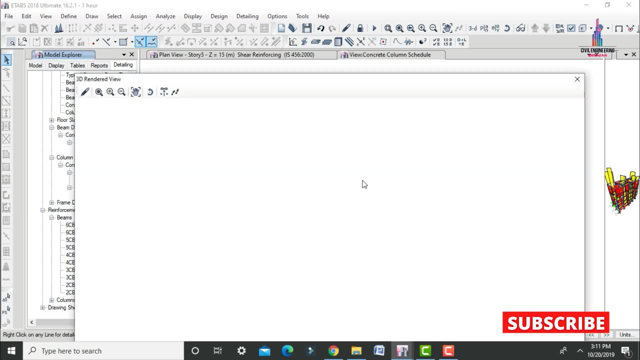 of the beam. just i'm selecting 4cb1 of the beam, just i'm selecting 4cb1. doubly connect so it will load your doubly connect, so it will load your doubly connect so it will load your respective reinforcement cage view for respective reinforcement cage view for. 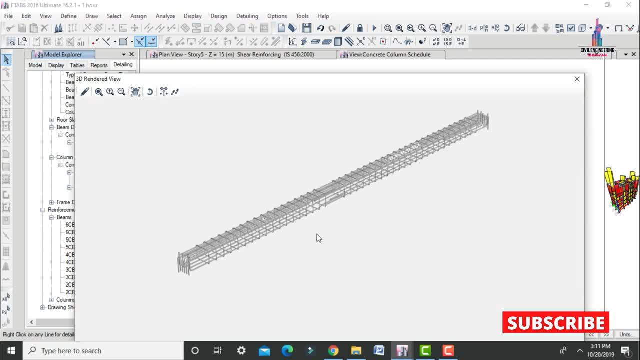 respective reinforcement cage view for this diagram. okay, so this is the beam- this diagram. okay, so this is the beam- this diagram. okay, so this is the beam. design results. reinforcement cage view. design results. reinforcement cage view. design results: reinforcement cage view. so it will be consisting of the different. 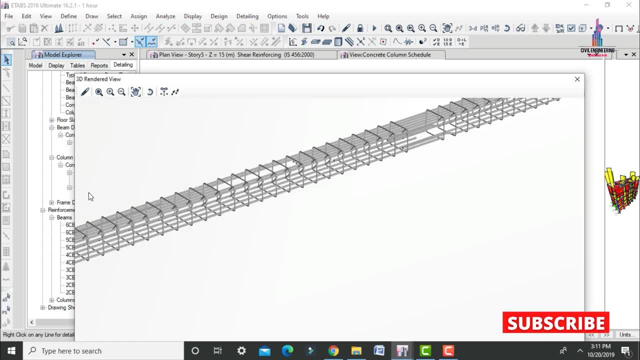 so it will be consisting of the different. so it will be consisting of the different properties and different zoning section properties and different zoning section properties and different zoning section for the two years member. okay, so this is for the two years member. okay, so this is for the two years member. okay, so this is the diagram which is showing for the 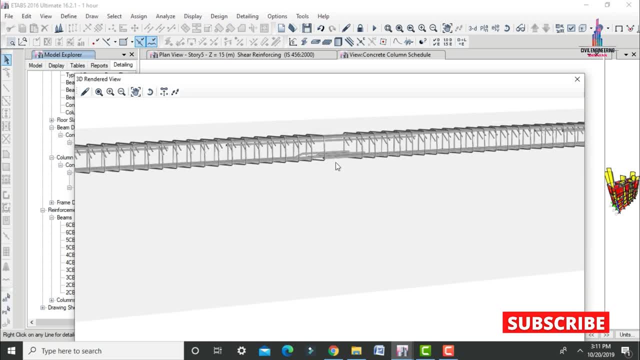 the diagram which is showing for the. the diagram which is showing for the reinforcement detailing for the beam reinforcement detailing for the beam reinforcement detailing for the beam section. okay, so this is the beam diagram section. okay, so this is the beam diagram section. okay, so this is the beam diagram results. again, in the same way we have to. 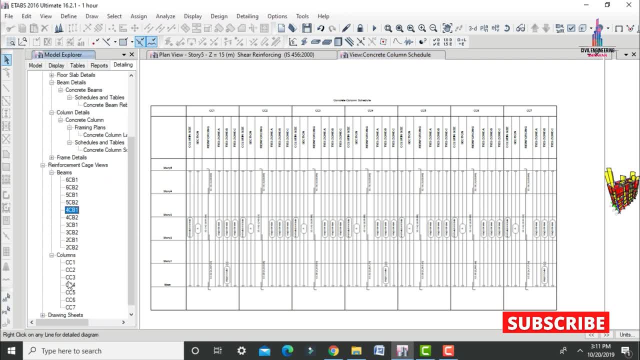 results again in the same way. we have to results. again in the same way. we have to select the reinforcement cage view for: select the reinforcement cage view for: select the reinforcement cage view for the column. also select the column. select the column. also select the column. select the column. also select the column. select any one of the columns. select this. 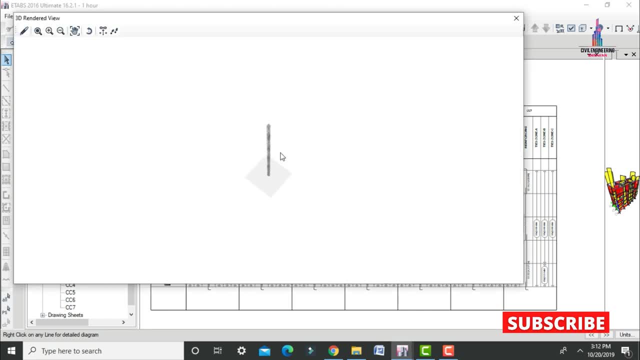 any one of the columns, select this. any one of the columns select this respected column cc1. so click on this respected column cc1. so click on this respected column cc1. so click on this respected option. so this is the data respected option. so this is the data. 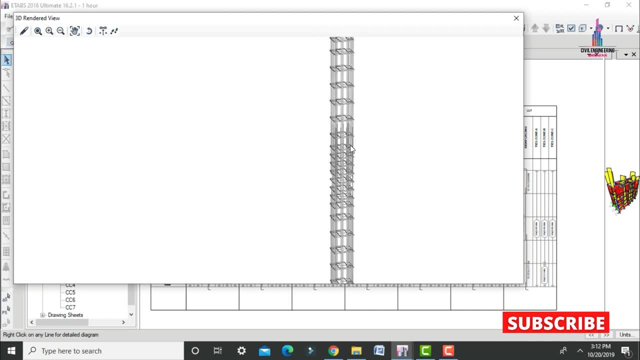 respected option. so this is the data which is related to the cc1. it will be which is related to the cc1. it will be which is related to the cc1. it will be consisting of the reinforcement values, consisting of the reinforcement values, consisting of the reinforcement values for the different floors here depending. 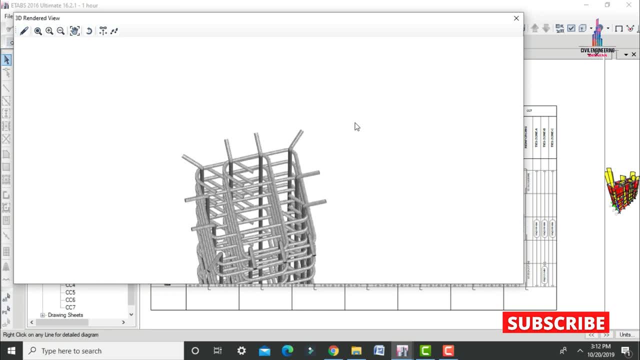 for the different floors here, depending for the different floors here, depending upon the considerations and depending upon the considerations, and depending upon the considerations and depending upon the output values. so this is also upon the output values, so this is also upon the output values. so this is also consisting of different types of 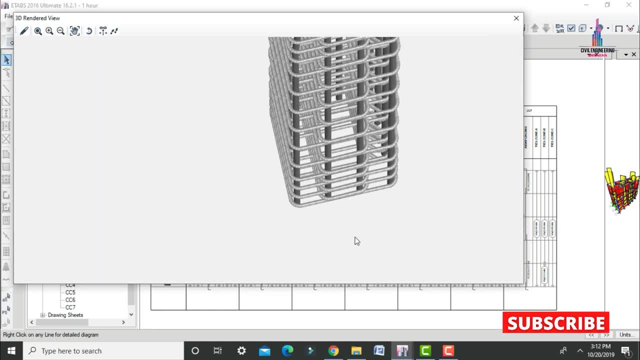 consisting of different types of, consisting of different types of reinforcement sections: okay, so as well. reinforcement sections- okay, so as well. reinforcement sections. okay, so as well, for the considerations we are taken. it for the considerations we are taken. it for the considerations we are taken. it has four bars: okay, in each direction. 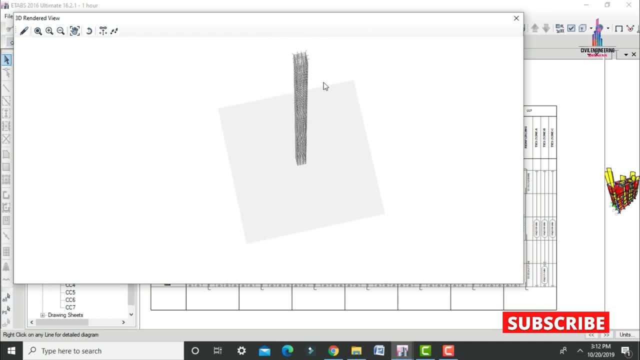 has four bars, okay, in each direction. has four bars, okay, in each direction, which is equals to 12. number of bars, which is equals to 12. number of bars, which is equals to 12. number of bars: total: okay, so this is the design. total: okay, so this is the design. 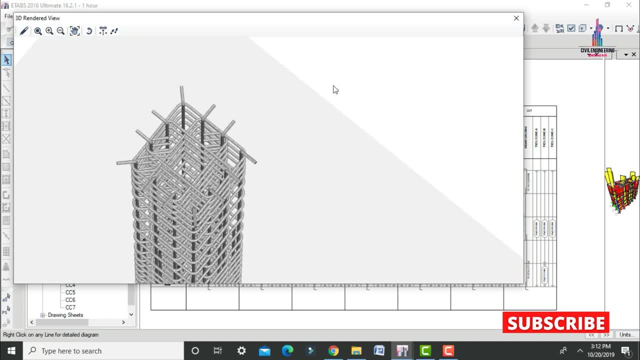 total. okay, so this is the design results, which is related to the column results, which is related to the column results, which is related to the column design section. okay, so, from this design section. okay, so, from this design section. okay, so, from this respected uh, values of the results. we 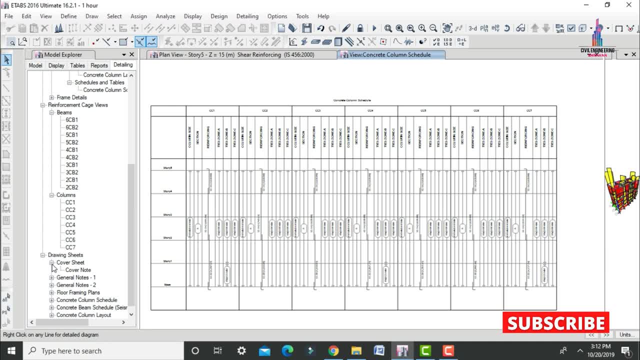 respected uh values of the results. we respected uh values of the results. we need to take the sheets drawing sheets. need to take the sheets drawing sheets. need to take the sheets drawing sheets. okay, so select the drawing sheet cover. okay, so select the drawing sheet cover. okay, so select the drawing sheet cover. note here: so this is the cover node. 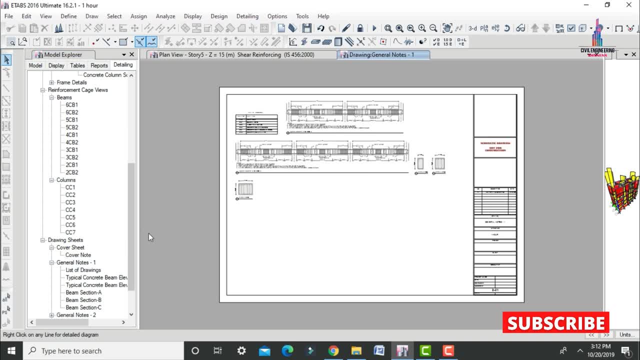 note here. so this is the cover node note here. so this is the cover node design results again. select a general design results again. select a general design results again. select a general notes option which is related to the notes option, which is related to the notes option which is related to the beam sections and column sections, and. 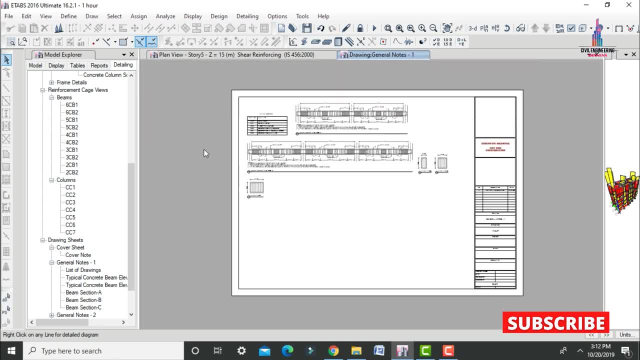 beam sections and column sections, and beam sections and column sections, and this is the output file we can give to. this is the output file we can give to. this is the output file we can give to the customers. okay, so, in the same way we the customers, okay, so, in the same way we. 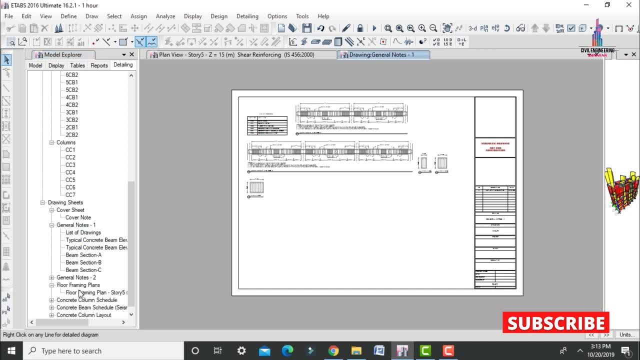 the customers. okay. so in the same way we have to select the have to select the have to select the flooring framing plans. okay, select the flooring framing plans. okay, select the flooring framing plans. okay, select the floor flaming plan. so this is the floor floor flaming plan. so this is the floor. 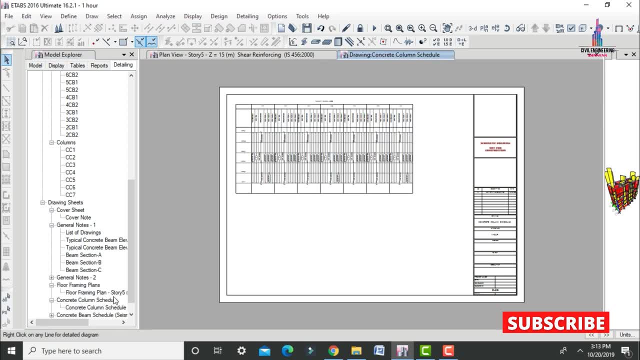 floor flaming plan. so this is the floor framing plans. again select the column framing plans. again select the column framing plans. again select the column scheduling details. so this is the column scheduling details. so this is the column scheduling details. so this is the column scheduling details. values: again select. 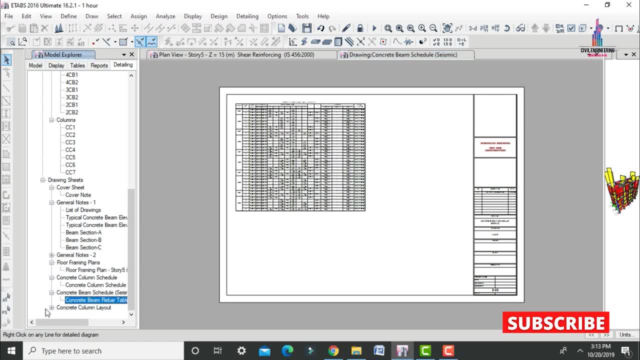 scheduling details. values again select scheduling details. values again select the beam scheduling details. so this is the beam scheduling details. so this is the beam scheduling details. so this is the beam scheduling details and column: the beam scheduling details and column: the beam scheduling details and column layout section diagram. so this is the. 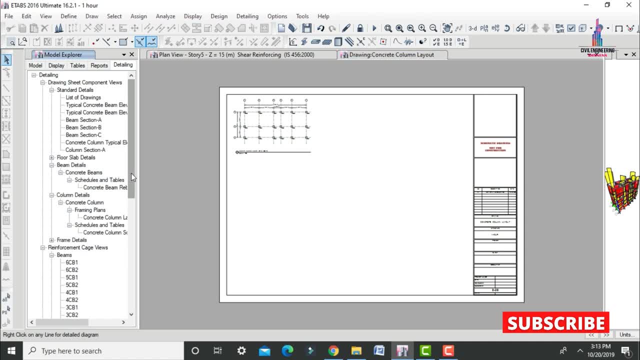 layout section diagram. so this is the layout section diagram. so this is the column layout section diagram. okay, so, column layout section diagram. okay, so column layout section diagram. okay, so after that we have to check the report. after that we have to check the report. after that we have to check the report here. okay, select the report here double. 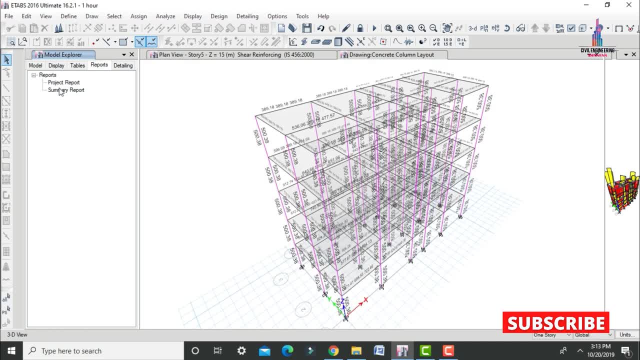 here: okay, select the report here double here. okay, select the report here double. click on it so click on project summary. click on it so click on project summary. click on it so click on project summary report. okay, so it will load your report. okay, so it will load your. 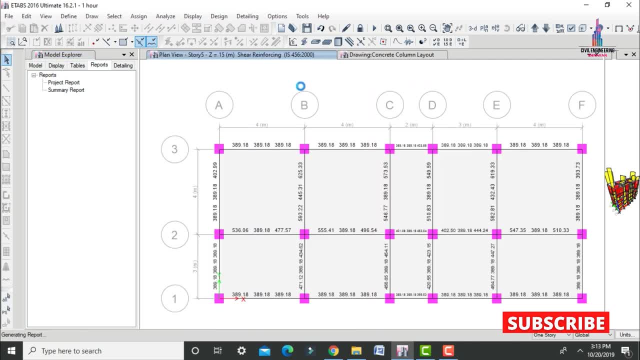 report. okay, so it will load your respective project summary report table. respective project summary report table. respective project summary report. table here: okay, which is consisting of all here. okay, which is consisting of all here. okay, which is consisting of all your design summary, which is related to your design summary, which is related to: 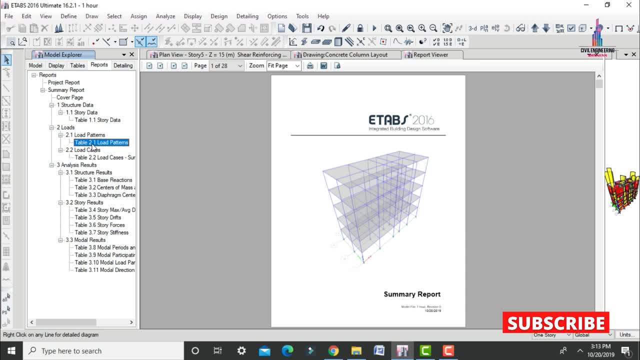 your design summary, which is related to the g plus 4 building, so select this: the g plus 4 building. so select this: the g plus 4 building. so select this. respected options: select any one of the respected options. select any one of the respected options. select any one of the page. it will be consisting of your all. 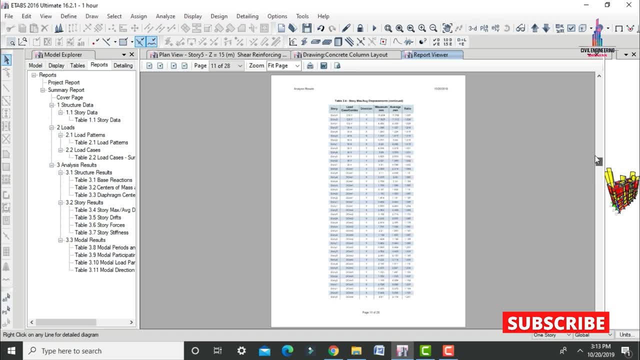 page. it will be consisting of your all page. it will be consisting of your all your calculation point, which is related, your calculation point, which is related, your calculation point, which is related to this respected building design, to this respected building design, to this respected building design process. okay, so this is the process. 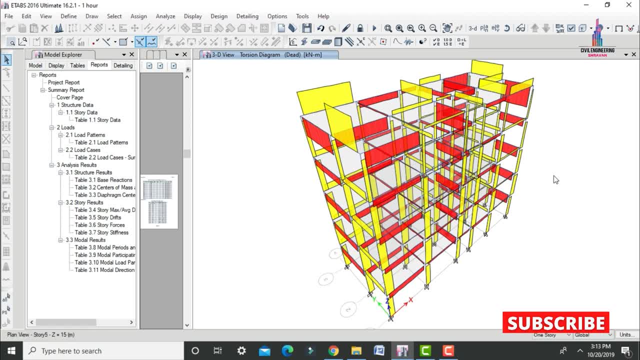 process. okay, so this is the process. process. okay, so this is the process. designing of g plus 4 building by using designing of g plus 4 building by using designing of g plus 4 building by using atap software, if you have any queries. atap software if you have any queries. 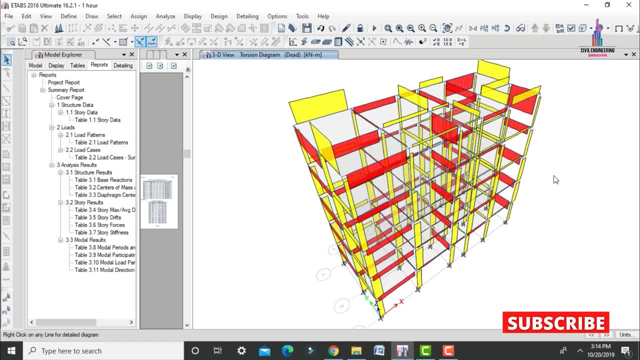 atap software. if you have any queries about this respected video, please text about this respected video. please text about this respected video. please text me your questions in the below. comment me your questions in the below. comment me your questions in the below comment box. i will give you the answers for the. 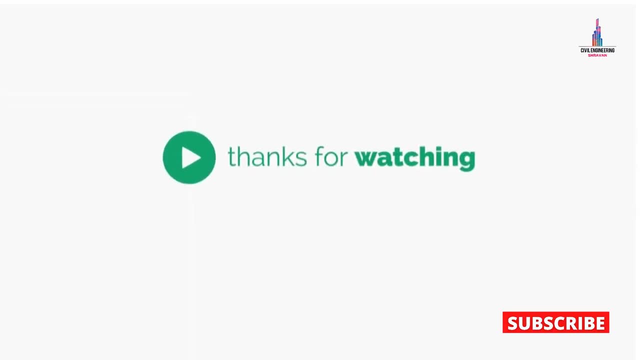 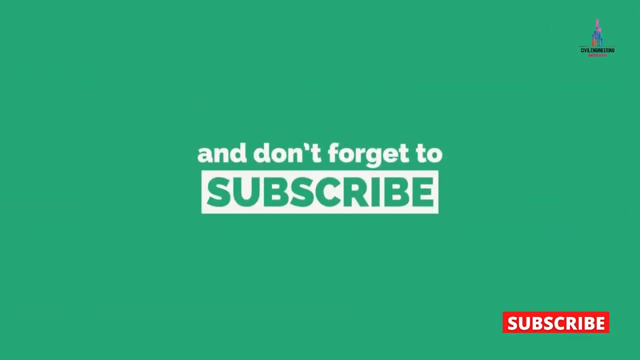 box. i will give you the answers for the box. i will give you the answers for the respected questions, thank you. 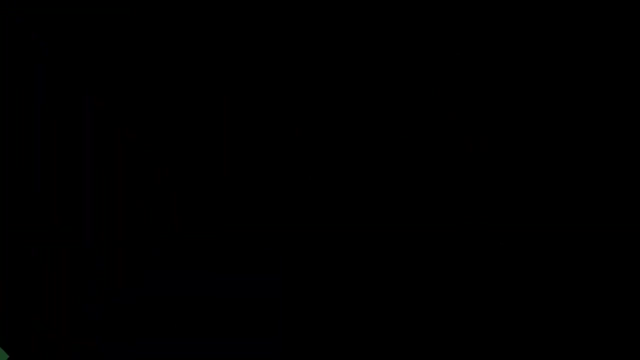 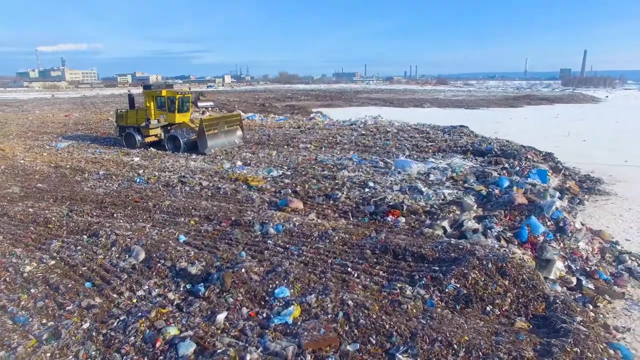 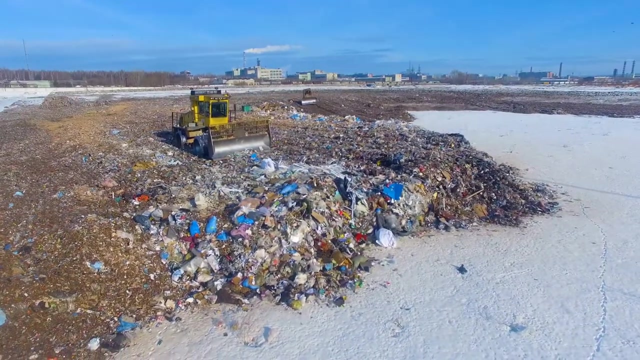 4 Ways of Waste Management. The environmental condition highly depends on the way you manage it and the way you deal with your waste. Waste management is the prevention, generation, monitoring, handling, treatment, residual disposition, characterization and reuse of solid wastes To know more about better waste. 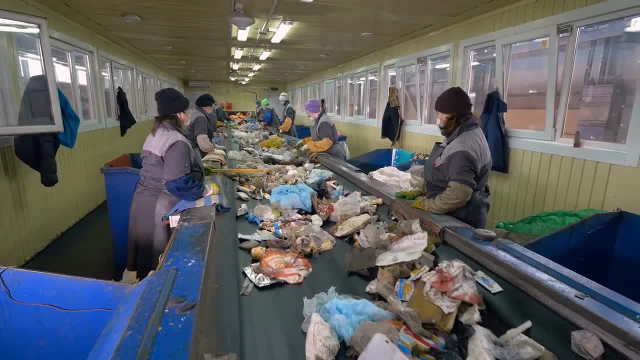 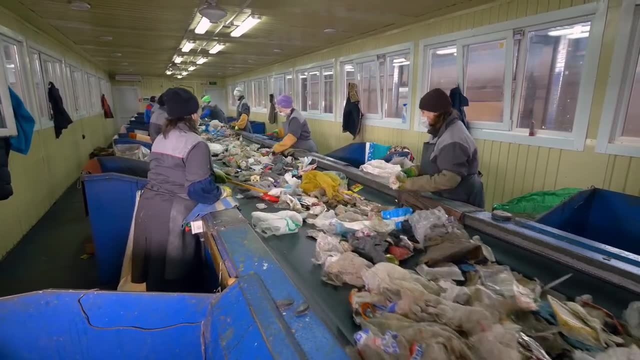 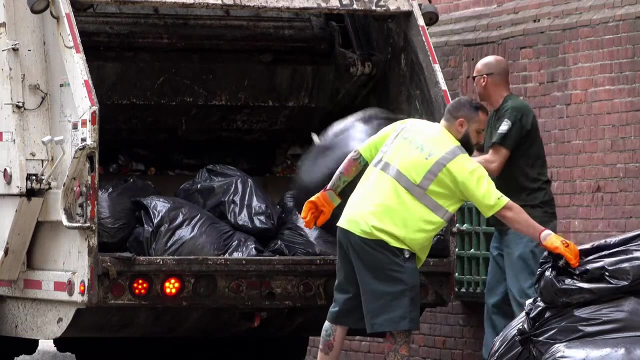 management and creating a better environment. read in this section. There are various types of solid waste, for example farming, municipal, commercial, residential, institutional and special sewage sludge, healthcare, household, hazardous wastes- Usually the word pertains to individuals' materials which are created by human activity. 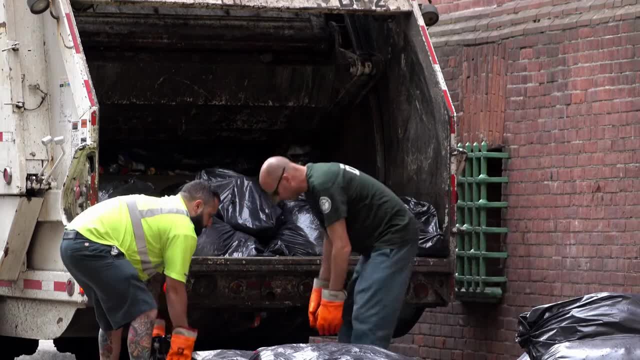 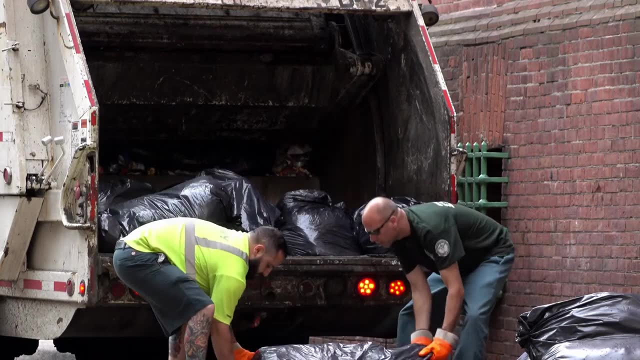 Besides, the operation is generally carried out to be able to decrease their impact on the environment, appearance or health. It is vital to understand how to conduct waste disposal In the realm of today, by which population is rising and thus is quick industrialization. it is vital to understand how to conduct waste disposal In the realm of today.